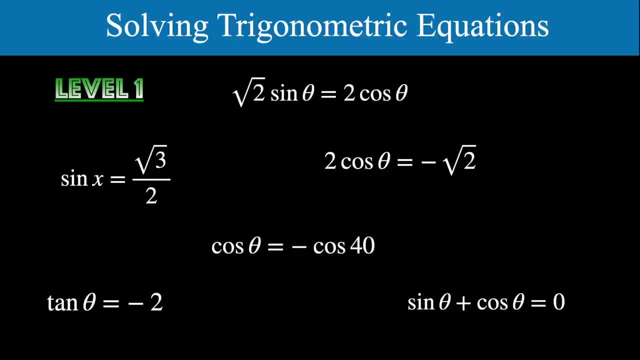 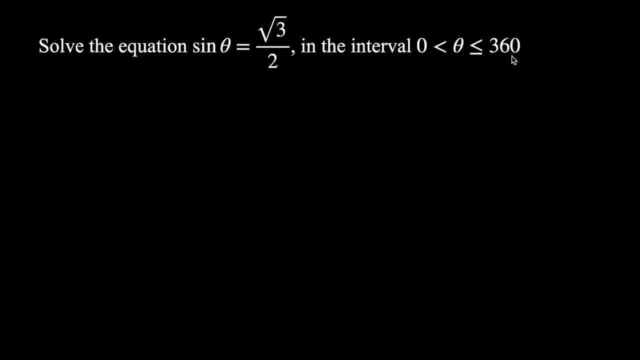 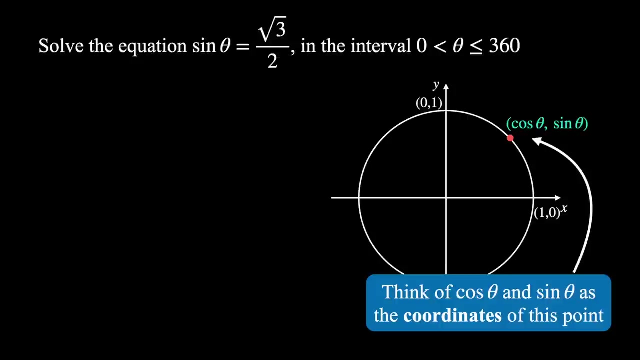 to solve for x here. Okay, let's jump into this first example then. So the question says solve the equation sine theta equals root three on two in the interval zero to 360 degrees. When they say solve the equation, they're really asking to find the value of theta or the values of theta in this interval. Okay, let's start with our unit circle. I'm going to be using the unit circle mostly in most of these problems, although I will show you an example using the graphs as well and how to solve equations with graphs. Okay, so remember how we're defining the sine function. Firstly, picture a point on this circle. And you can think of cosine theta and sine theta as the coordinates of this point. Okay, so it has x and y coordinates of cosine theta sine theta. Again, go back to that video on the unit circle if you're not sure about this. So now what this equation is telling you, if sine theta equals root three on two, that's saying the y coordinate of this point is root three on two. So that's saying the y coordinate of this point is root three on two. So that's saying the y coordinate of this point is root three on two. We also know there's another point on this circle in the second quadrant that will have this same y coordinate. So we can already see we're actually going to get at least two answers here. Okay, let's draw our radii in. And the question is when this question says find theta, it's asking what is the angle of rotation starting from one 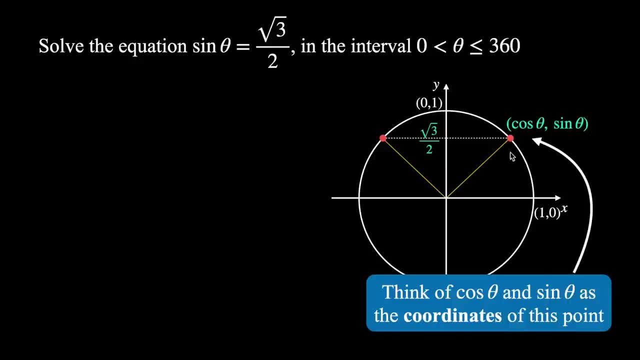 zero to this point on the circle? How many degrees have I rotated around the circle to get here where the y coordinate is? 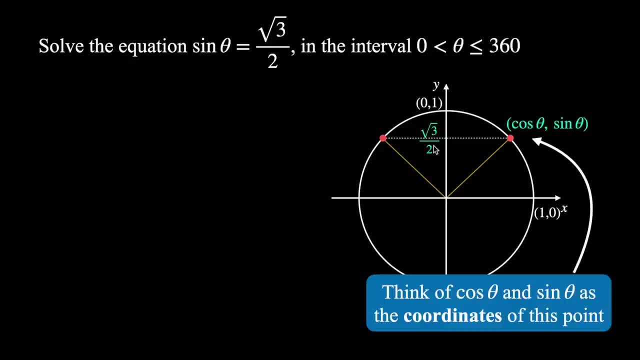 So actually you're going to be getting around to the sin. So this is the angle of rotation starting from zero to the half degree here. The y coordinate of the data is equal toится equal to six, same with therefore the angle of rotation starting from one zero to the half degree here is equal to one zero. So for y coordinate we are going to have x plus theJoie to the half degree. So we 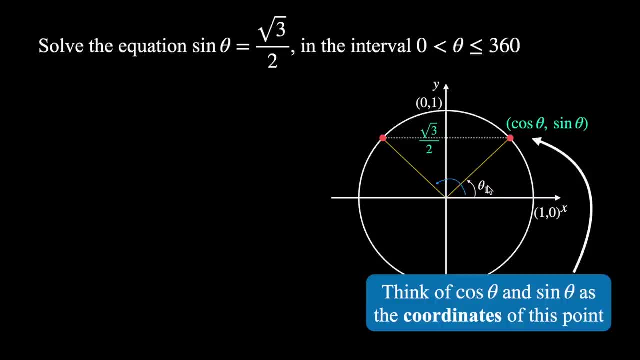 are going to haven't looked at the whole system of equations here because this is what we ever need to find, is the initial angle is equal to six. 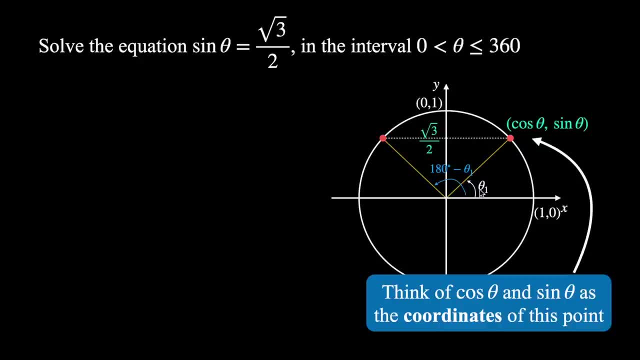 Okay, and in terms of anxiom dynamics – what you need to find is root three on two. And well to the angle i call the reference angle sometimes also called the base angle or principal value i don't know why it has different names doesn't really matter what you call it it's just the idea 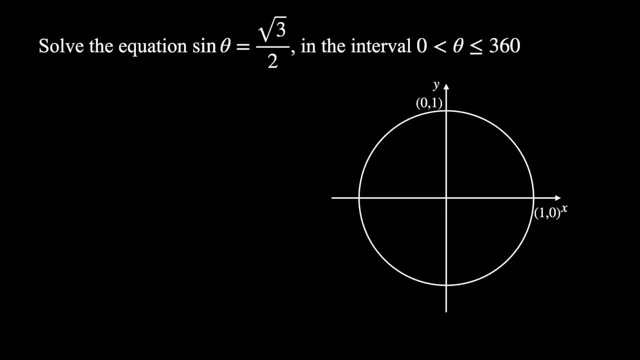 most of these problems, although I will show you an example using the graphs as well, and how to solve equations with graphs. Okay, so remember how we're defining the sine function. Firstly, picture a point on this circle And you can think of cosine theta and sine theta as the coordinates of this. 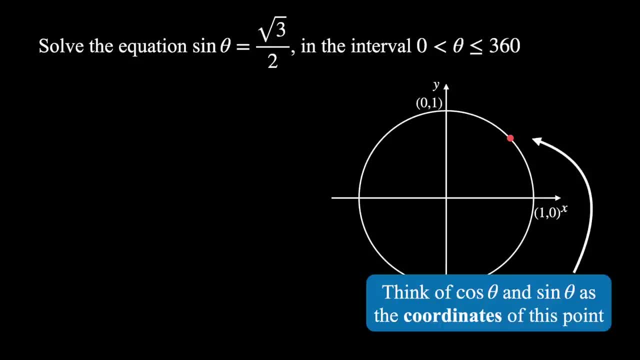 point. Okay, so it has x and y coordinates of cosine theta, sine theta- Again, go back to that video on the unit circle if you're not sure about this. So now what this equation is telling you: if sine theta equals root, three on two, that's saying the y coordinate of this point is root. 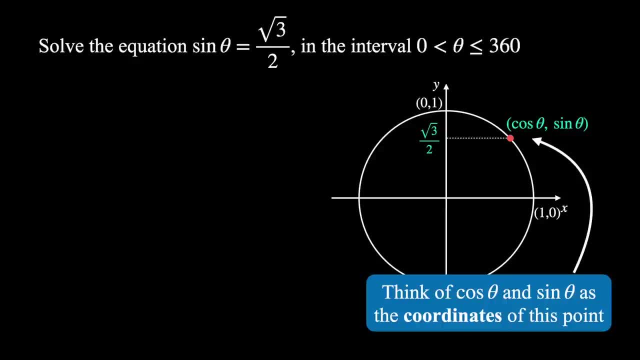 three on two. So that's saying the y coordinate of this point is root three on two. So that's saying the y coordinate of this point is root three on two. We also know there's another point on this circle in the second quadrant that will have this same y coordinate. So we can already see we're. 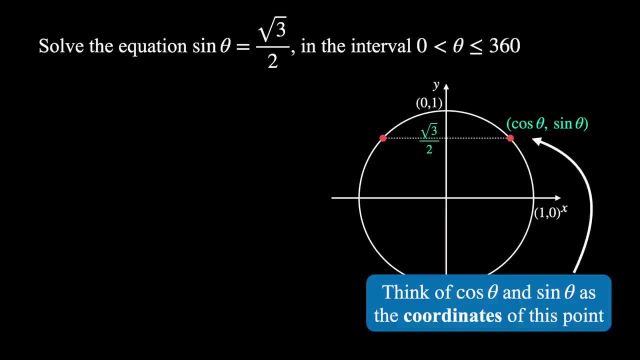 actually going to get at least two answers here. Okay, let's draw our radii in. And the question is: when this question says find theta, it's asking: what is the angle of rotation starting from one zero to this point on the circle? How many degrees have I rotated around the circle to get here? where? 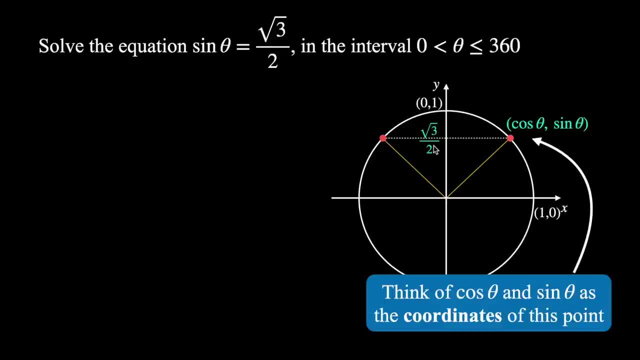 the y coordinate is. So this is actually going to be x, theta sine theta. Again, you have to do that the way I do. Okay, but this is going to be theta sine theta. so I just don't know where the y coordinate here than the. 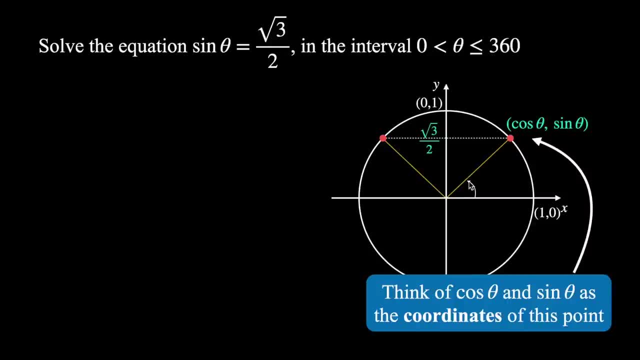 y coordinate here, but this is going to be here or theta on one. So what I'm going to do is I'm going to the spin over here to raise what's equal to theta or the travel here to the the line. I'm going to the the paper there. so now we've circle two. I've placed all the dato on. 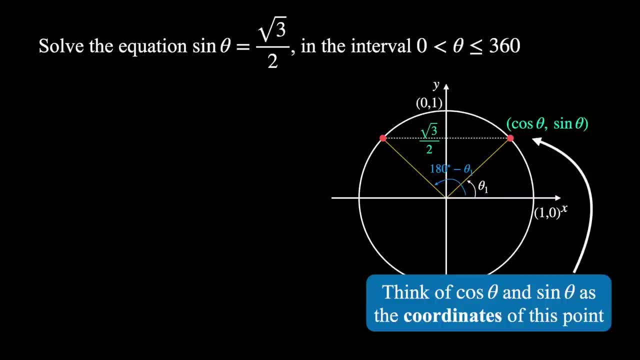 the end of the circle. if I've got the ratio of two to two and 180 to matrix and now we get the bütün, suffix becomes the annealing function And this return is spizing. think of as saying angle i call the reference angle, sometimes also called the base angle or principal value. 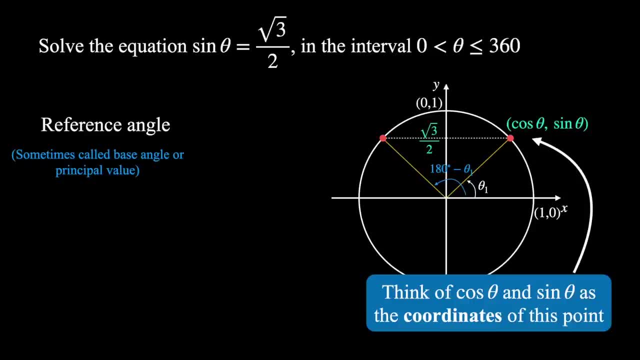 i don't know why it has different names, doesn't really matter what you call it, it's just the idea that we're finding this, this first angle to the first point, and that's going to allow you to find the rest of the solutions. okay, so this reference angle is the inverse sign of the y coordinate. 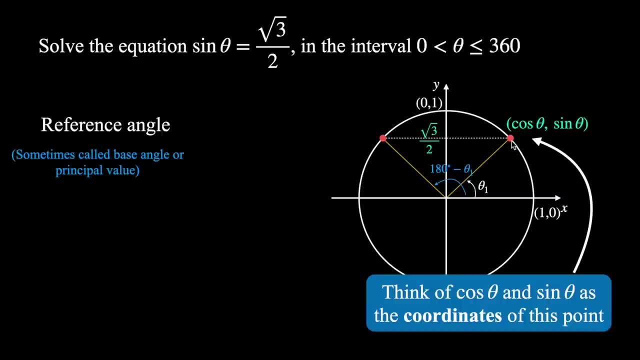 that we're finding this this first angle to the first point and that's going to allow you to find the rest of the solutions okay so this reference angle is the inverse sign of the y coordinate now you may know the exact value of root 3 and 2. i've got a video on how you know how you can 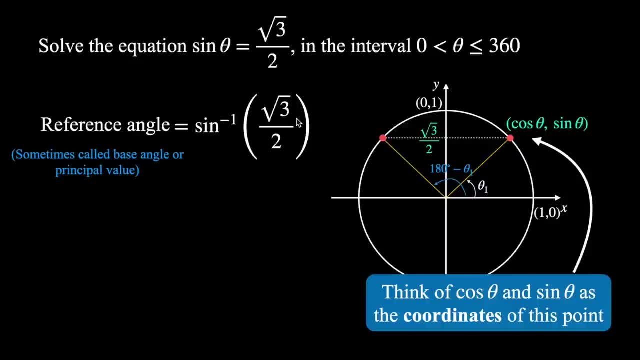 remember exact value to trig functions so check that out if you want but if you take the inverse 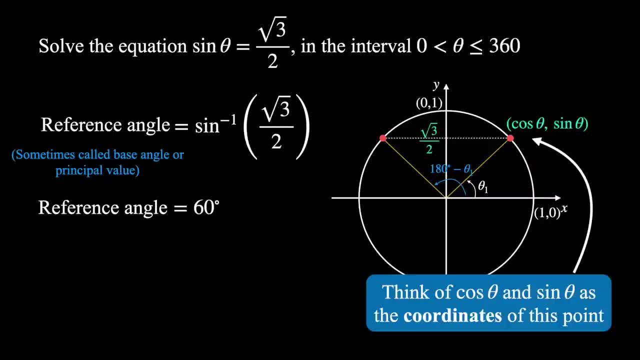 sign of root 3 and 2 then you get the reference angle of 60 degrees what that's telling you is this initial angle to this first point here the angle of rotation is 60 degrees okay so that's actually one solution for our equation here one solution is theta equal to 60 degrees and now that we have that first angle we can work out the second solution the angle of rotation to the second point on the circle 180 take 60 that's 120 degrees and now make sure you check your 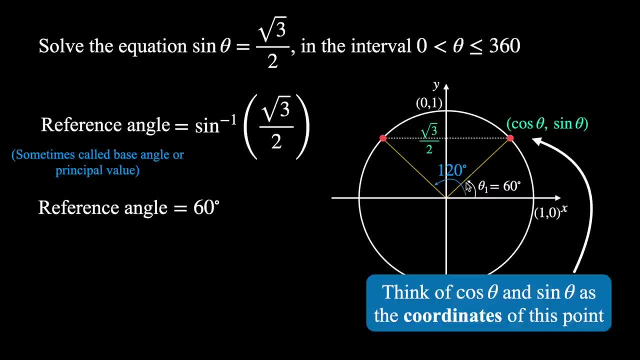 intervals so the next solution would be if we go all of all the way around the circle and get back to this point so it would be 360 plus 60. do i need to include that solution no because it's outside of our interval so the only solutions for theta i get here are 60 degrees and 120 degrees and that's our final 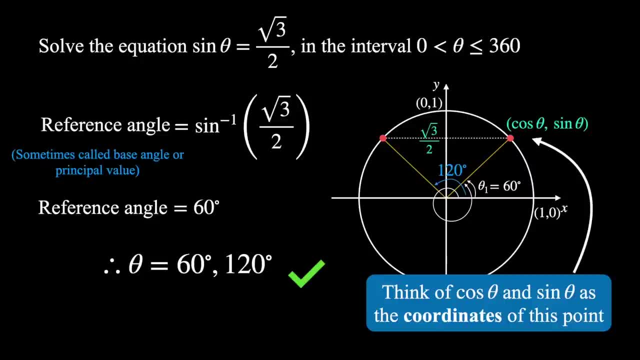 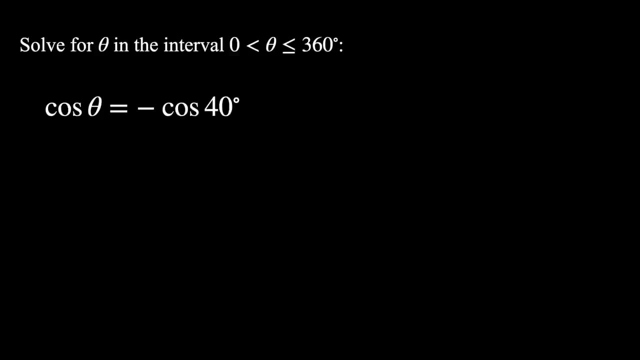 answer okay so this is the basic idea that i'm going to be using to solve the rest of the equations um you know as long as you understand the unit circle uh it all sort of follows from that but let's go through an example using uh the graphs just so maybe you prefer using the the graphs to solve equations okay so this question says solve for theta into in the interval 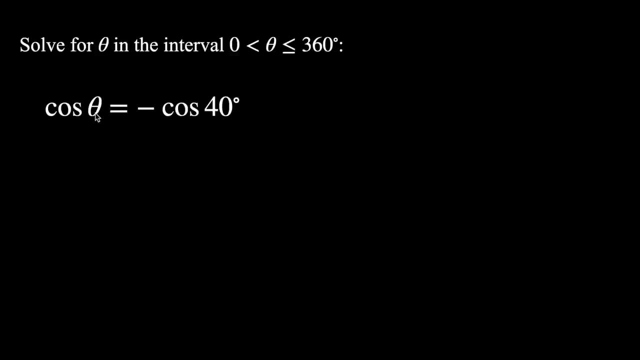 to 360 again and we have the equation cosine theta equals negative cosine of 40 degrees so to solve equations with the graphs firstly you start in this case we're going to start with the the graph 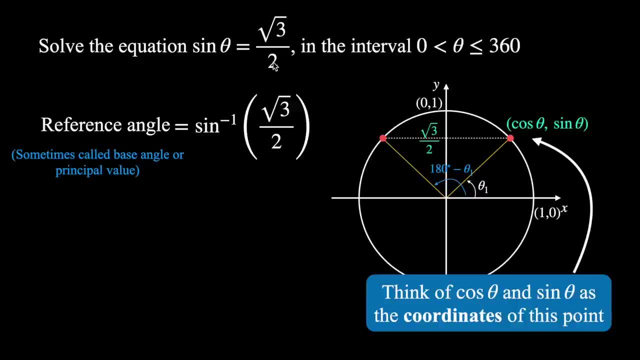 now you may know the exact value of root 3 and 2.. i've got a video on how you know, how you can remember exact value to trig functions, so check that out if you want. but if you take the inverse sign of root 3 and 2, then you get the reference angle of 60 degrees. what that's telling you is: 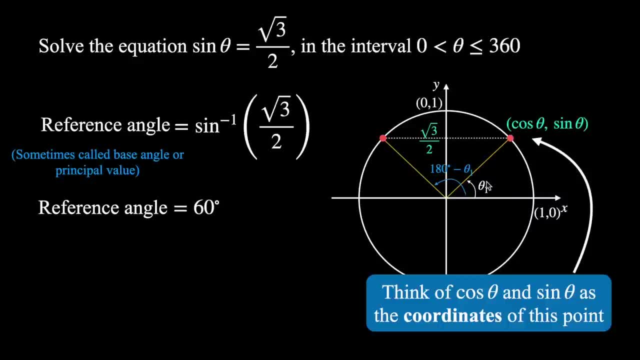 this initial angle to this first point. here the angle of rotation is 60 degrees. okay, so that's actually one solution for our equation here. one solution is theta equal to 60 degrees, and now that we have that first angle, we can work out the second solution, the angle of rotation to 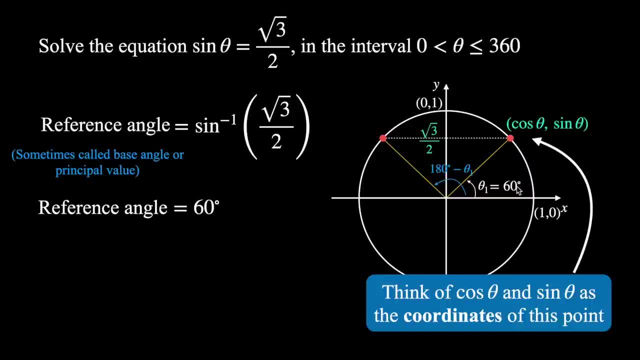 the second point on the circle: 180 take 60, that's 120 degrees, and now make sure you check your intervals. so the next solution would be if we go all of all the way around the circle and get back to this point, so it would be 360 plus 60.. do i need to include that solution? no, because it's outside. 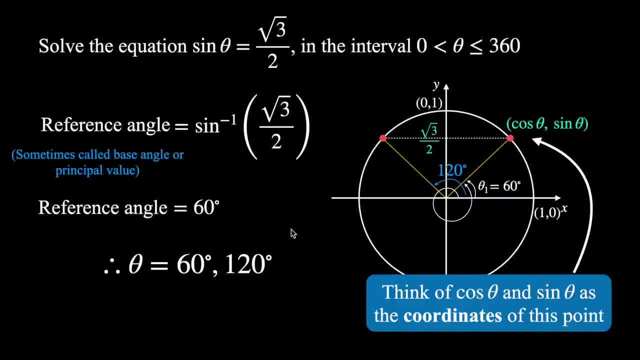 of our interval. so the only solutions for theta i get here are 60 degrees and 120 degrees, and that's our final answer. okay, so this is the basic idea that i'm going to be using to solve the rest of the equations. um, you know, as long as you understand the unit circle, uh, it all sort of follows from: 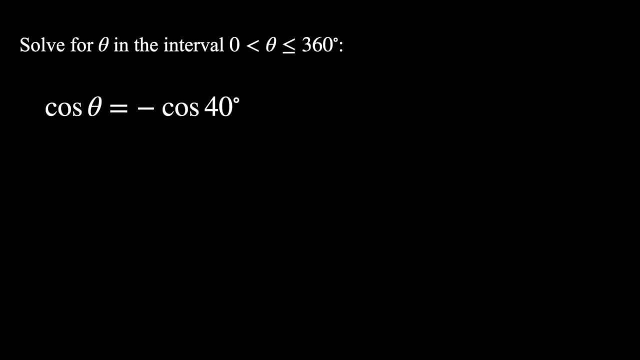 that. but let's go through an example using, uh, the graphs, just so maybe you prefer using the the graphs to solve equations, okay. so this question says: solve for theta into in the interval to 360 again, and we have the equation: cosine: theta equals negative cosine of 40 degrees. so to solve, 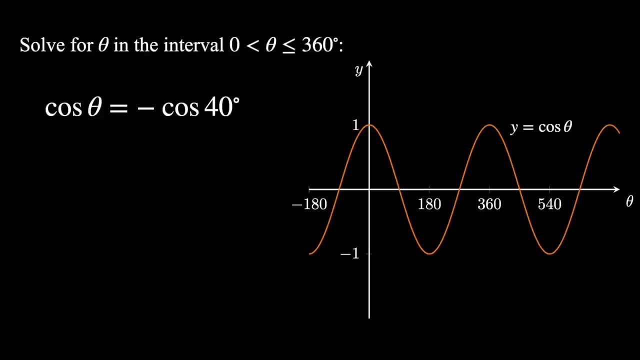 equations with the graphs. firstly, you start- in this case we're going to start- with the, the graph of the cosine function, because we've got cosine theta equal to something and you could get a decimal for this negative cosine 40. if you plug that into a calculator, you get approximately. 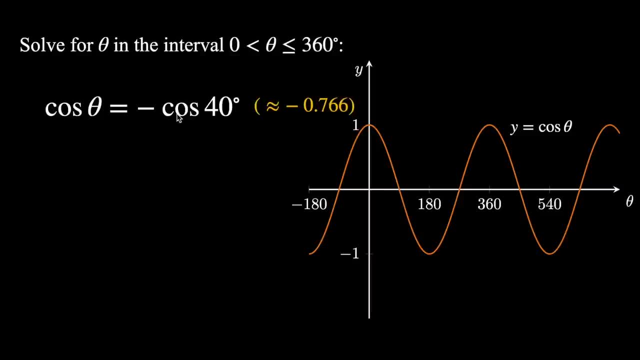 negative point seven, six, six. the next thing you do is to draw a horizontal line at this value. so we're going to draw a horizontal line at negative point seven, six, six, and this is the line with equation. y equals negative cosine 40.. so let's interpret. 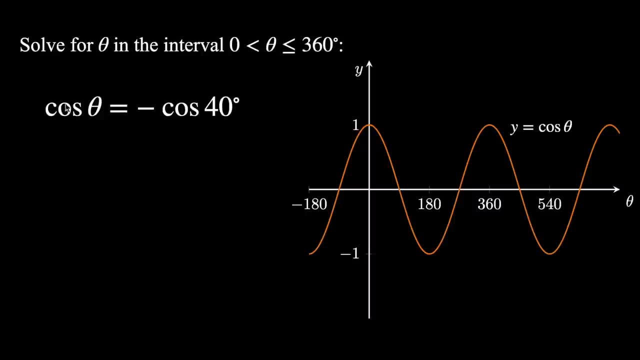 of the cosine function because we've got cosine theta equal to something and you could get a decimal for this negative cosine 40 if you plug that into a calculator you get approximately negative point seven six six the next thing you do is to draw a horizontal line at this value so we're going to draw a horizontal line at negative point seven six six and this is the line with equation y equals negative cosine 40. so let's interpret what this equation says in terms of the graph this is saying the graph of the cosine of theta is equal to negative cosine 40 or is equal to this horizontal line in other words the solutions to this equation will be where this line intersects the graph of cosine theta so what we're looking for is these points of intersection where that horizontal line cuts the graph to find the first point here we take the inverse cosine of negative cosine 40 that gives us our first solution if you put that into your calculator you get 140 degrees so this first point is at an angle of 140 degrees and to find the rest of the solutions you use symmetry because the graph is symmetrical if this angle is 40 degrees less than 180 this point must be 40 degrees more than 180. so yeah basically just using symmetry so this point here is at 180 plus 40 that's 220 degrees and then again check your interval 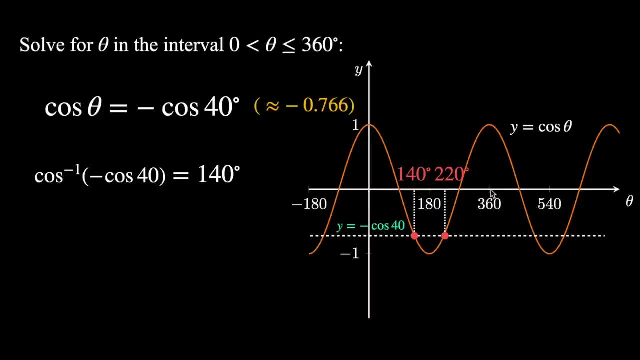 are there any more points of intersection between 0 and 360 we can easily see there are not so these are all of the solutions we need for this equation so we get theta equals to 140 degrees and 220 degrees and we're done so that's using graphing to solve trigonometric equations i prefer using 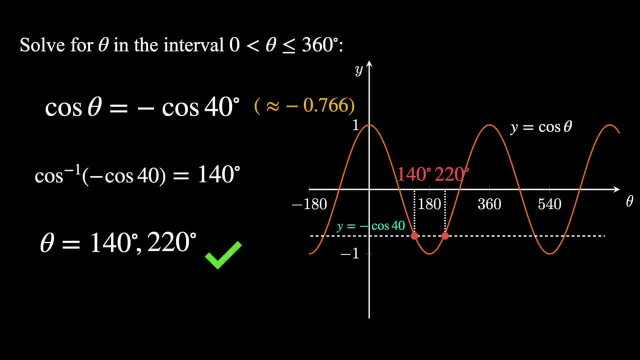 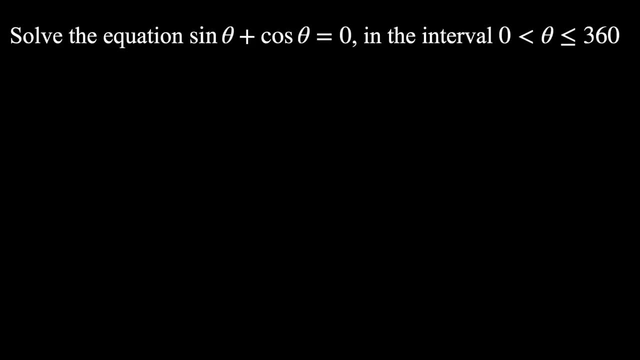 the unit circle um so i'm going to proceed using the unit circle but hopefully you found that useful if you want to use graphing instead okay let's look at another level one example this one says solve the equation sine theta plus cosine theta equals zero in the interval zero to 360. okay how to proceed here? 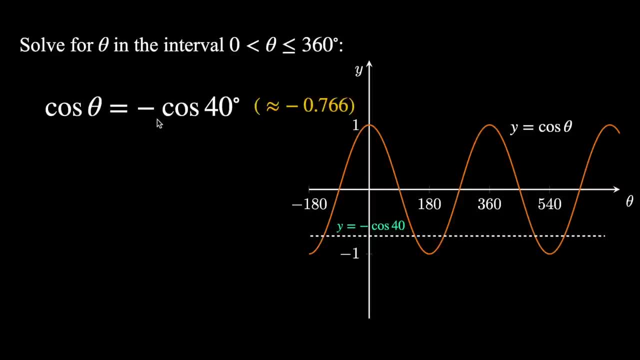 what this equation says in terms of the graph. this is saying the graph of the cosine of theta is equal to negative cosine 40 or is equal to this horizontal line. in other words, the solutions to this equation will be where this line intersects the graph of cosine. 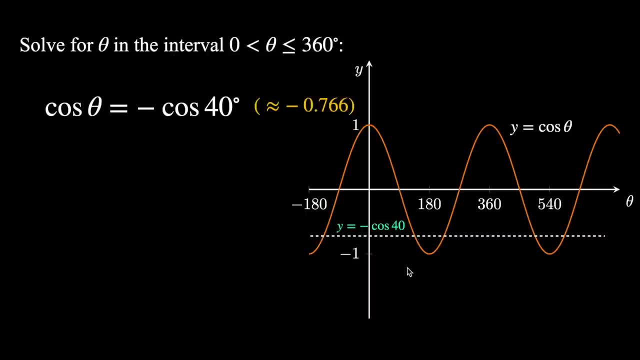 theta. so what we're looking for is these points of intersection where that horizontal line cuts the graph. to find the first point here, we take the inverse cosine of negative cosine 40. that gives us our first solution. if you put that into your calculator you get 140 degrees. so this first point. 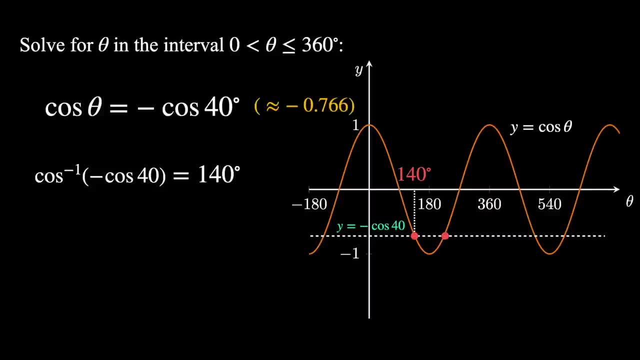 is at an angle of 140 degrees and to find the rest of the solutions you use symmetry, because the graph is symmetrical. if this angle is 40 degrees less than 180, this point must be 40 degrees more than 180.. so yeah, basically just using symmetry. 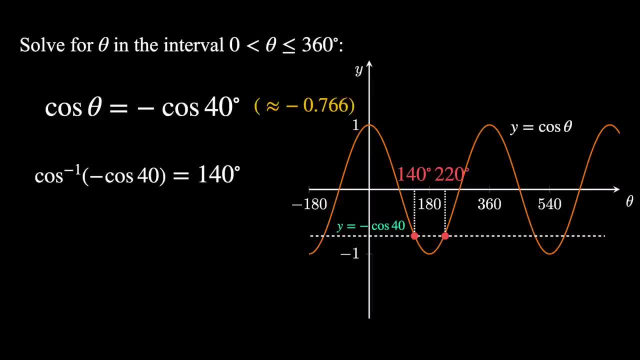 so this point here is at 180 plus 40, that's 220 degrees. and then again check your interval: are there any more points of intersection between 0 and 360? we can easily see there are not. so these are all of the solutions we need for this equation. so we get: theta equals to 140 degrees and 220. 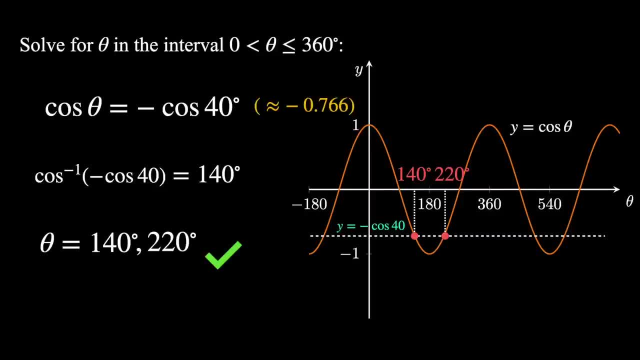 degrees and we're done so. that's using graphing to solve trigonometric equations. i prefer using the unit circle, um, so i'm going to proceed using the unit circle, but hopefully you found that useful. if you want to use graphing instead, okay, let's look at another level. one example: this one: 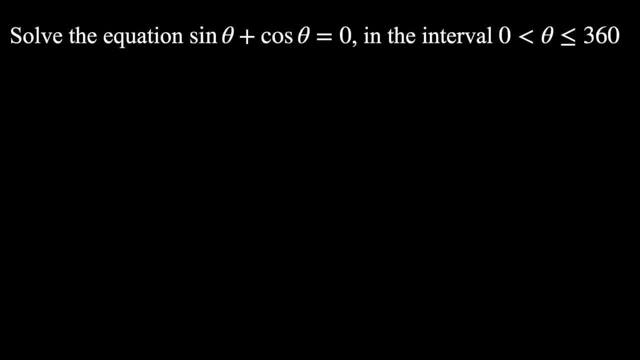 says: solve the equation: sine theta plus cosine theta equals zero in the interval zero to 360.. okay, how to proceed here? well, the main thing you're aiming for in trigonometric equations is to have one function on the left and some a constant on the right. so, for example, i want sine theta equal to two, or 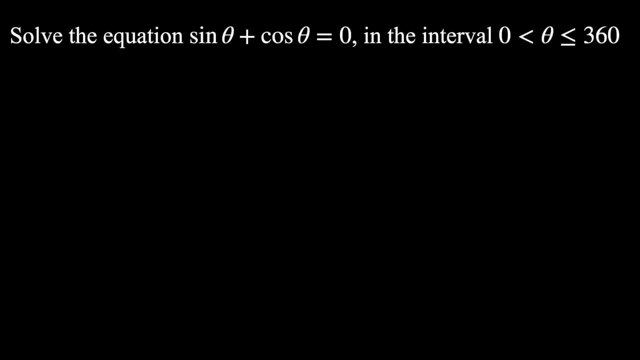 tan theta equal to one. i want some trigonometric function on the left of the equation and a number on the right. at the moment, you know, i don't see any way to find the value of theta when the equation is written like this. so what i can do is to rearrange so that sine theta equals negative. 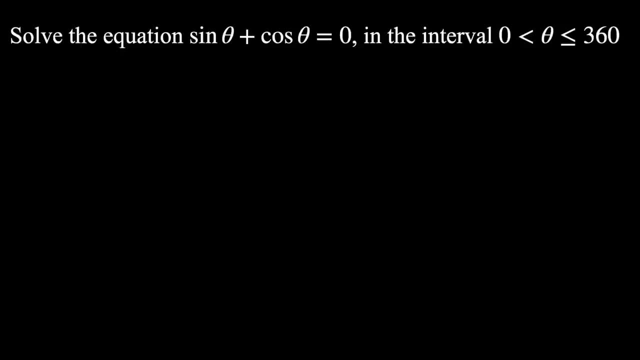 well the main thing you're aiming for in trigonometric equations is to have one function on the left and some a constant on the right so for example i want sine theta equal to two or tan theta equal to one i want some trigonometric function on the left of the equation and a number on the right at the moment you know i don't see any way to find the value of theta when the equation is written like this so what i can do is to rearrange so that sine theta equals negative cosine theta and can you see the next step if i divide by cosine theta i get sine theta over cosine theta equal to negative one so i'd have that negative one left over on the right if i divide it by cosine theta but just be careful when you're doing this because the trigonometric 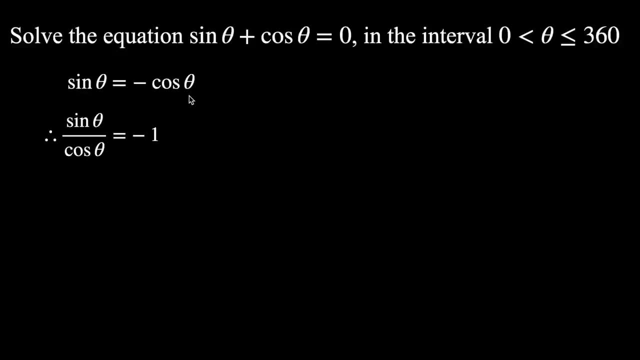 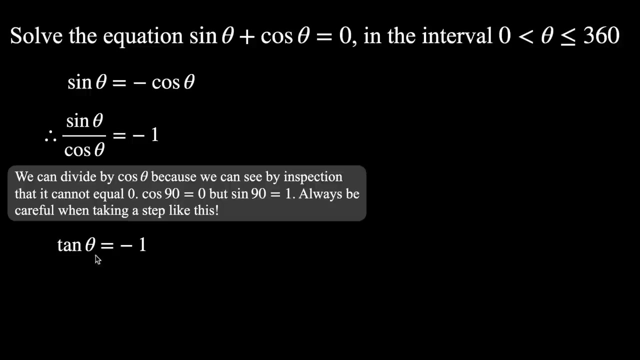 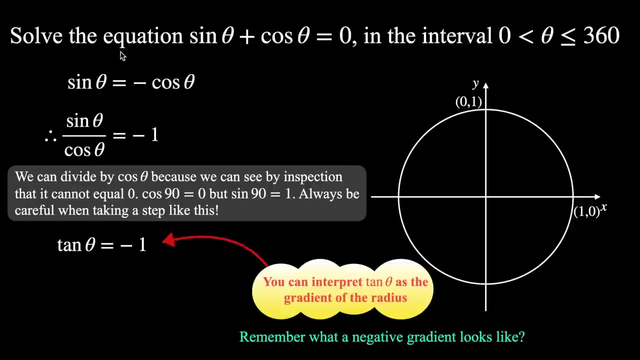 functions can equal zero remember you cannot divide by zero and so you can't divide by zero in this particular case i can divide by cosine theta because we can see by inspection that it cannot equal zero because cosine of 90 is zero but sine of 90 is one we can see that 90 would not be a solution to this equation so there's no way that cosine theta can equal zero and sine theta equal to zero so i can divide by cosine theta but just be careful when taking steps like this when dividing by you know trigonometric functions and dividing by cosine theta and sine theta equal to zero sometimes they can be zero be careful of that okay so sine theta on cosine theta equals negative one therefore tan theta equals negative one this is where now that i have my trig function on the left my number on the right i draw up my unit circle so we're thinking of sine and cosine as the x and y coordinates of the point on the circle how do we think about tan we can interpret tan theta as the gradient of the radius and because tan theta is a negative we interpret this as a negative gradient so do you remember what the negative gradient looks like so one way to remember that is if you're a man walking across the screen are you going downhill are you getting more negative or are you going uphill is the you know are you going up is it positive so down it you know downhill going across the screen is a negative gradient 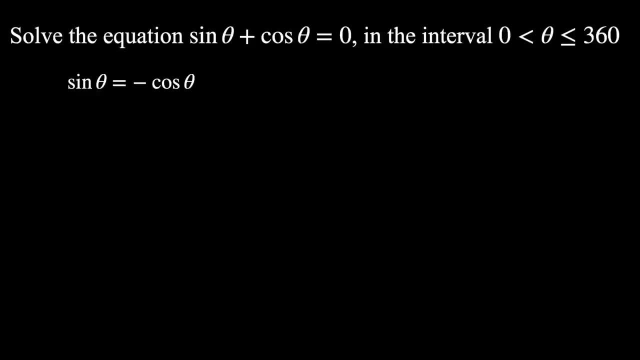 cosine theta. and can you see the next step? if i divide by cosine theta, i get sine theta over cosine theta, equal to negative one. so i'd have that negative one left over on the right if i divide it by cosine theta. but just be careful when you're doing this, because the trigonometric 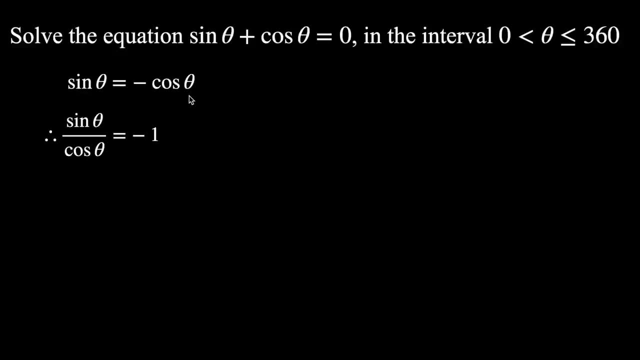 functions can equal zero. remember you cannot divide by zero and so you would want to be careful. In this particular case I can divide by cosine theta, because we can see by inspection that it cannot equal zero, Because cosine of 90 is zero but sine of 90 is one. we can see that 90 would. 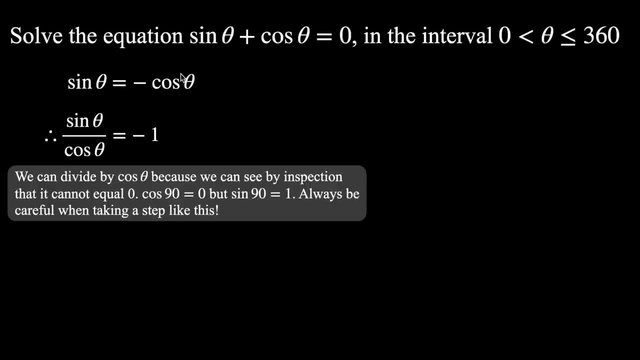 not be a solution to this equation. So there's no way that cosine theta can equal zero and sine theta equal to zero. So I can divide by cosine theta, but just be careful when taking steps like this, When dividing by- you know trigonometric functions- sometimes they can be zero. Be careful. 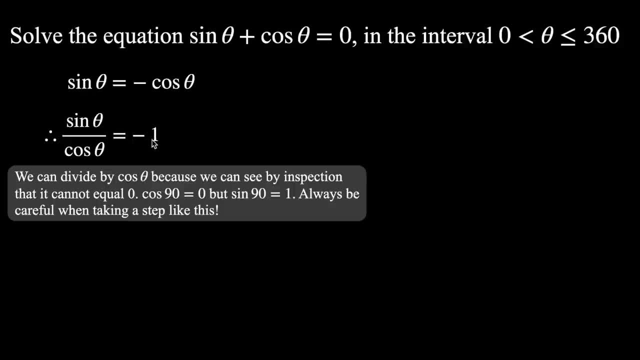 of that. Okay, so sine theta on cosine, theta equals negative one. therefore, tan theta equals negative one. This is where, now that I have my trig function on the left, my number on the right, I draw up my unit circle. So we're thinking of sine and cosine as the x and y coordinates of 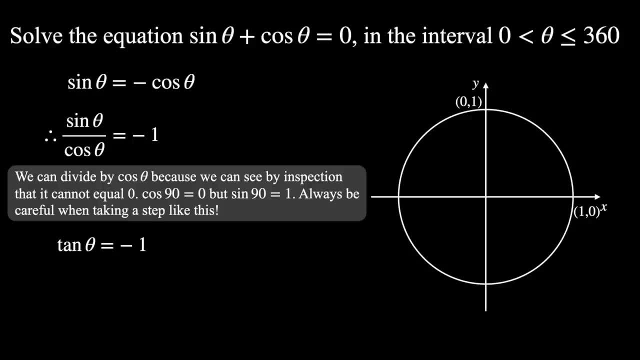 the point on the circle. How do we think about tan? We can interpret tan theta as the gradient of the radius, And because tan theta is a negative, we interpret this as a negative gradient. So do you remember what the negative gradient looks like? So one way to remember that is if you're a man walking. 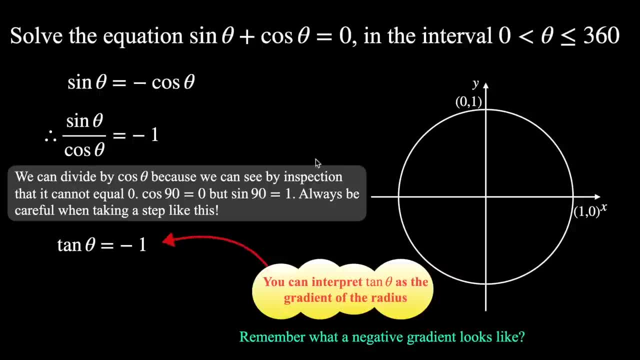 across the screen. are you going downhill? Are you getting more negative or are you going uphill? Is the you know? are you going up? Is it positive? So down, you know. downhill, going across the screen is a negative gradient. So when the radius has a negative gradient, 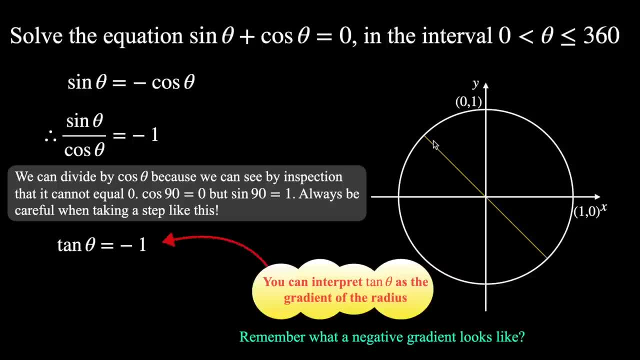 it's in the second quadrant and the fourth quadrant. Okay, If the radius is in the first or the third quadrant, it has a positive gradient. So that's how we know where the solutions will be. It'll be in the second or the fourth quadrants, And the first thing we need to figure out is this angle. 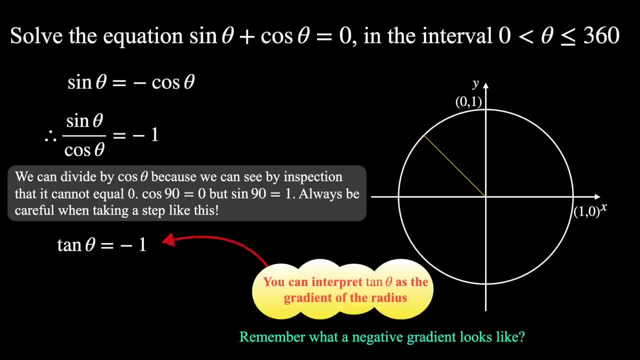 so when the radius has a negative gradient it's in the second quadrant and the fourth quadrant okay if the radius is in the first or the third quadrants has a positive rating a positive gradient so that's how we know where the solutions will be it'll be in the second or the fourth quadrants and the first thing we need to figure out is this angle in here the reference angle the 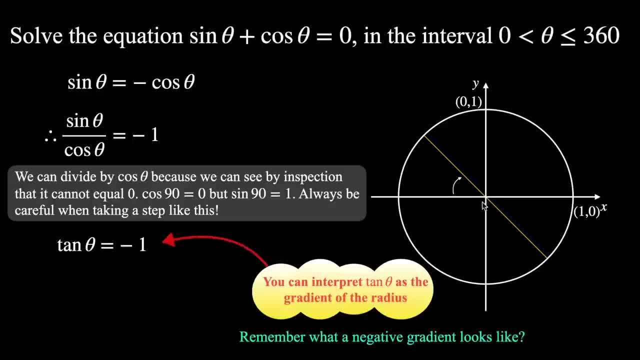 angle between the x-axis and the radius to do that we want you know the the angle when tan of the e equals negative 1. 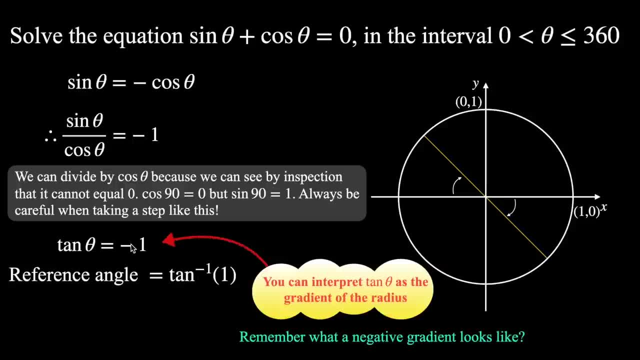 we take the inverse tan of one ignore the signs when you're finding the reference angle again i hate to keep bringing it up but go back to my video on the unit circle i talk about how you can imagine a right triangle in here and the sign of this number doesn't matter when you're trying to figure out that angle in there so anyway it's inverse tan of one remember your exact values is 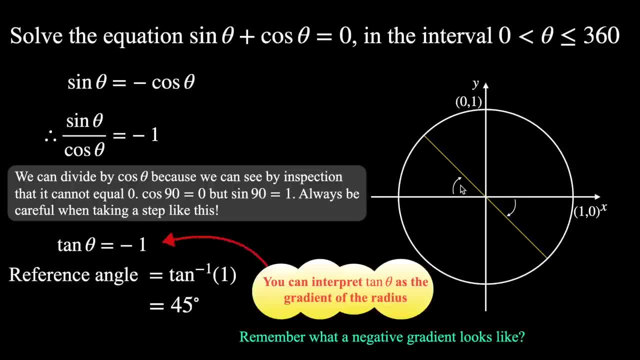 going to be 45 degrees so this angle in here is 45 but remember the angle of rotation we care about is anti-clockwise starting at one zero so we actually want this angle that's going to be 180 take 45 that's 135 degrees also we want this angle going around to the second radius that we've drawn in that's going to be 360 take 45 that's 315 degrees and check your interval you 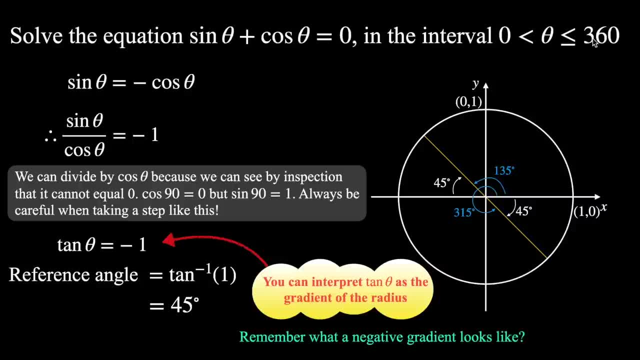 going to be 45 is that all of the solutions between zero and 360 yes it is so we get theta equal to 135 degrees and 315 degrees 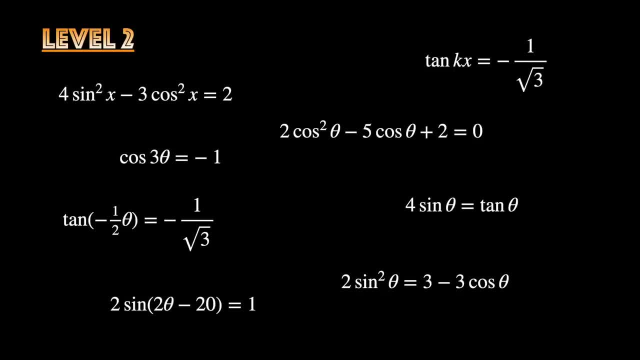 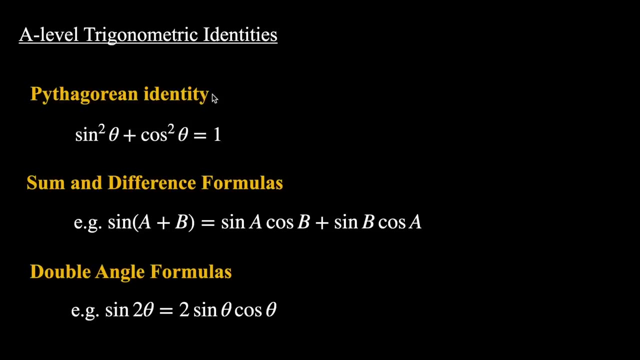 let's move on to some level two equations these are going to involve you can see we've got some squared terms we're going to be factorizing we've got some we're going to have a quadratic equation in here and we're going to use one of our identities the pythagorean identity which says the piggy��고 of problemsidi形 also we're going to we're going to use one of our identities the that sine squared theta plus cosine squared theta equals one. 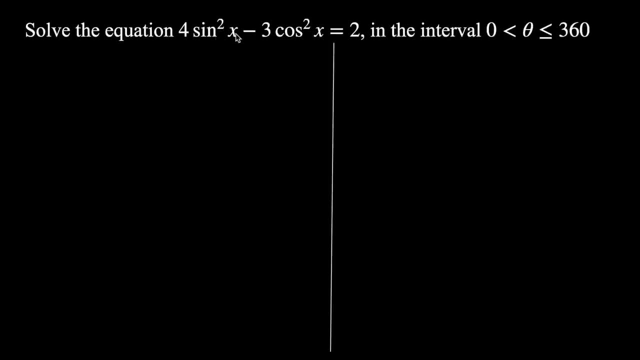 Okay, so let's start with this problem. It says solve the equation for sine squared x take three cosine squared x equals two in the interval zero to 360 degrees. 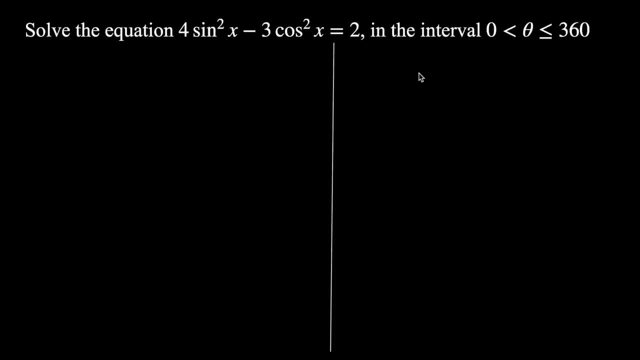 Okay, remember we want one function on the left and a number on the right. 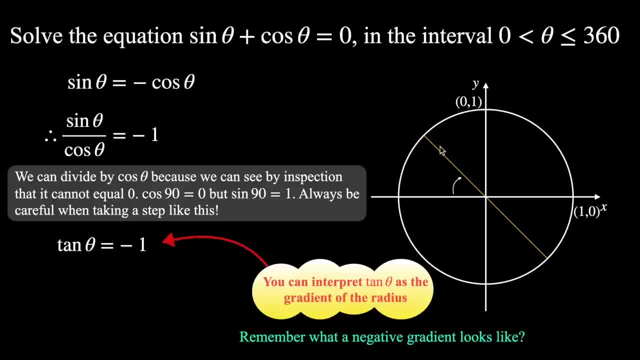 in here the reference angle, the angle between the x-axis and the radius. To do that we want you know the angle when tan. tan of theta equals negative one. So we take the inverse tan of one. ignore the signs when you're. 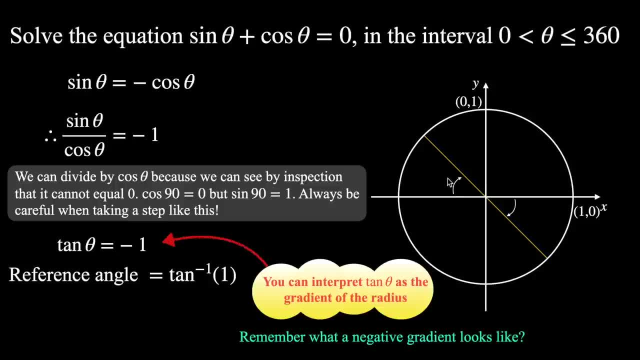 finding the reference angle. Again, I hate to keep bringing it up, but go back to my video on the unit circle. I talk about how you can imagine a right triangle in here, and the sign of this number doesn't matter when you're trying to figure out that angle in there. So anyway, it's inverse tan. 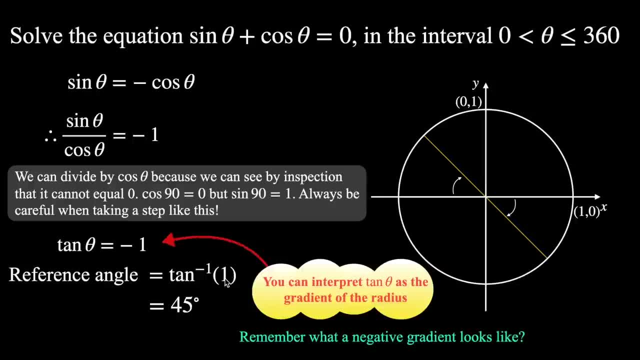 of one. Remember your exact values is going to be 45 degrees. So this angle in here is 45.. But remember, the angle of rotation we care about is anti-clockwise, starting at one zero. So we actually want this angle. That's going to be 180. take 45.. That's 135 degrees. Also, we want this. 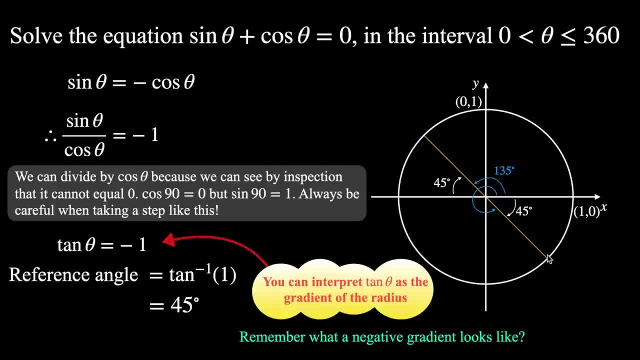 angle going around to the second radius that we've drawn in, That's going to be 360. take 45. That's 315 degrees, And check your interval. Is that all of the solutions between zero and 360? Yes, it is. 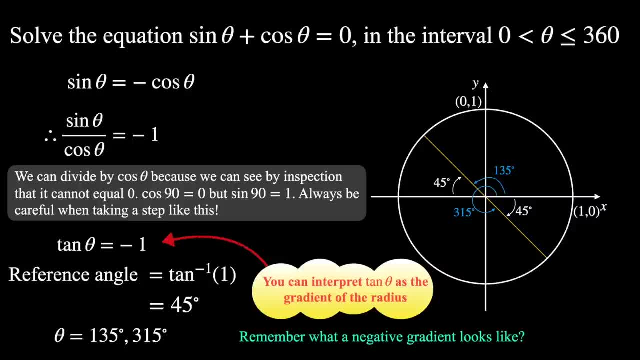 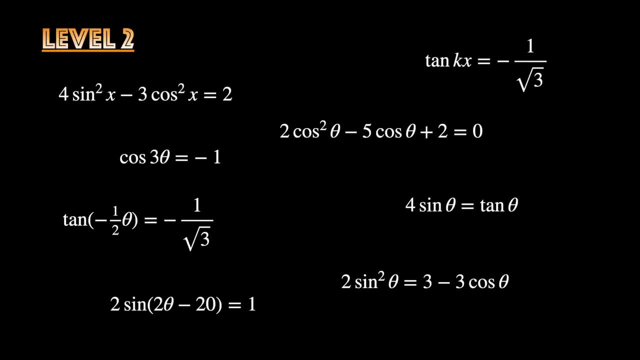 So we get theta equal to 135 degrees and 315 degrees. Let's move on to some level. two equations These are going to involve. you can see, we've got some squared terms, We're going to be factorizing. We've got some, we're going to. 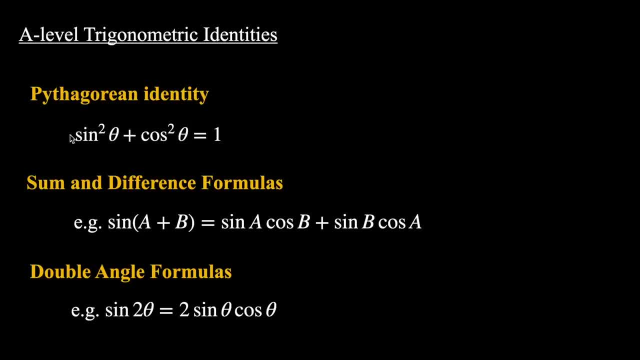 have a quadratic equation here, And we're going to use one of our identities, the Pythagorean identity, which says that sine squared theta plus cosine squared theta equals one. Okay, let's start with this problem. It says: solve the equation for sine squared x, take three cosine. 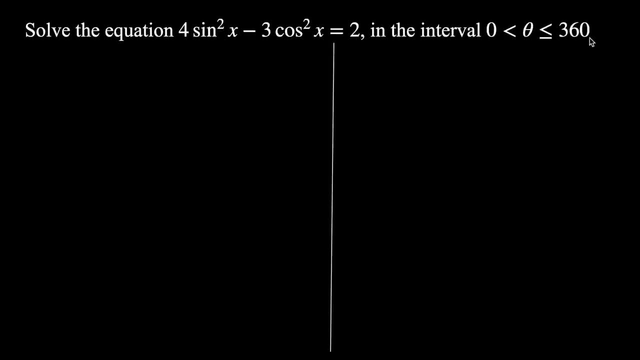 squared, x equals two in the interval zero to 360 degrees. Okay, remember, we want one function on the left and a number on the right. At the moment, I have sine and cosine and they're both squared. The first question you can ask yourself is how can I have this equation all in terms of one? 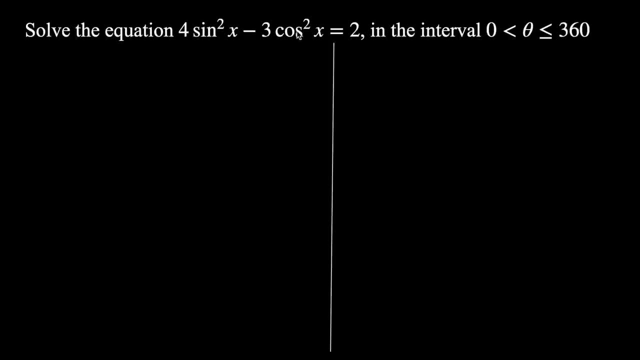 At the moment I have sine and cosine and they're both squared. The first question you can ask yourself is how can I have this equation all in terms of one trig function? So how can I have it in terms of either sine or cosine? Well, we can use that Pythagorean identity. 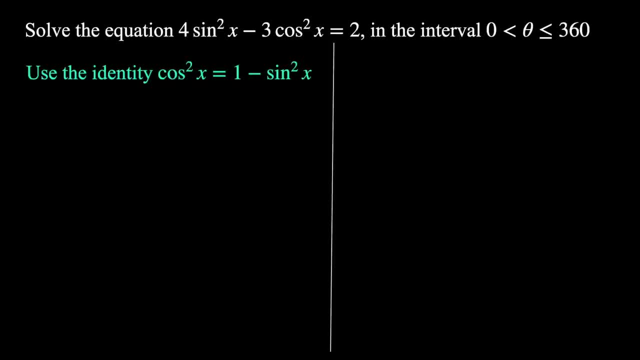 So use the identity cosine squared x equals one take sine squared x. You could also use sine squared x equals one take cosine. 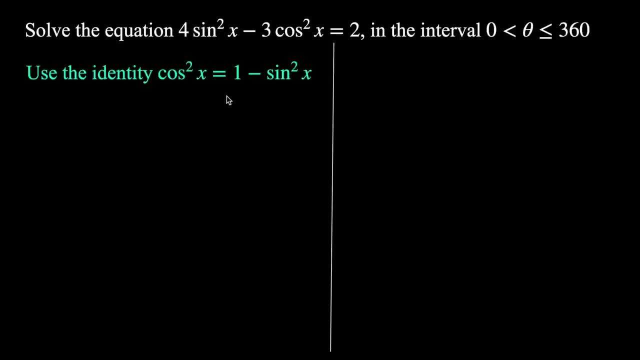 I think it would still work. I'm just going to choose to use this one. So I'm going to plug in one take sine squared x for cosine squared. And then I'll have it all in terms of sine squared x. Okay, so plug that in for cosine squared x then expand these brackets. 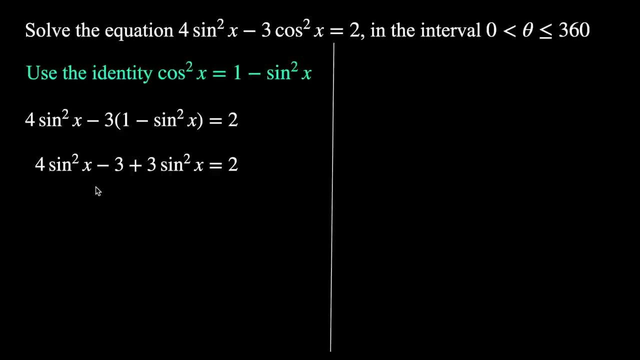 So we get four sine squared x take three plus three sine squared x equals two. Then four sine squared x plus three sine squared x is seven squared x. And I can also add that negative three to the right hand side. So I get seven squared x equals five, then divide by seven sine squared x equals five and seven. Then take the square root of both sides and I get sine x equals plus or minus the square root of five on seven. 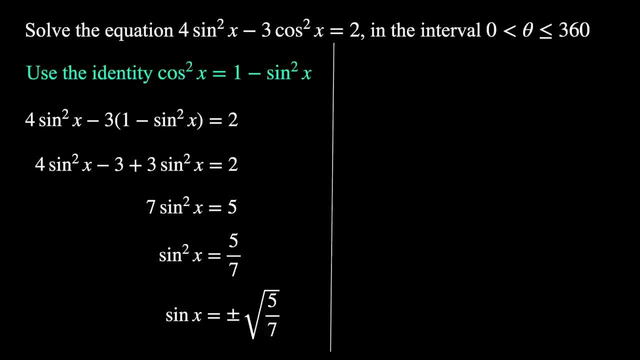 Okay, now we have that trig function on the left, the constant on the right. 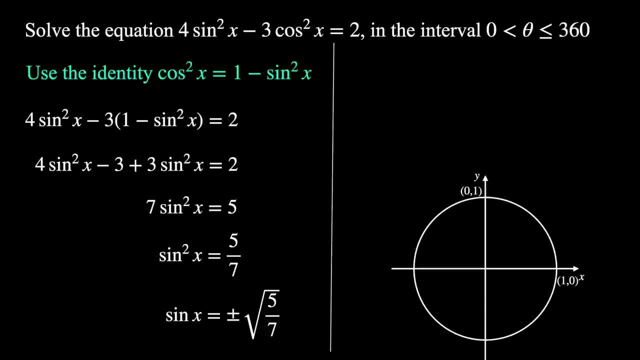 This is where we go to our unit circle. And remember how we're interpreting this. Imagine the point on the circle. 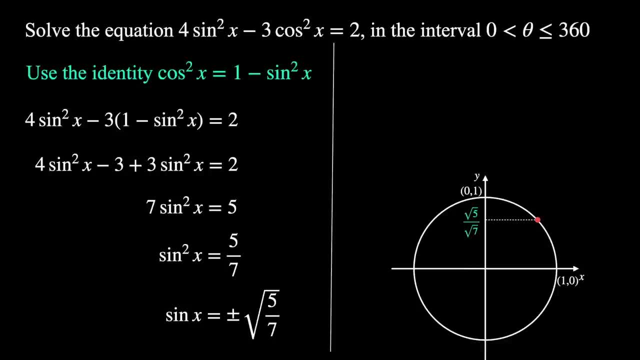 That point there is going to have a y coordinate of positive root five on root seven. Then we have another point as well with that same y coordinate. 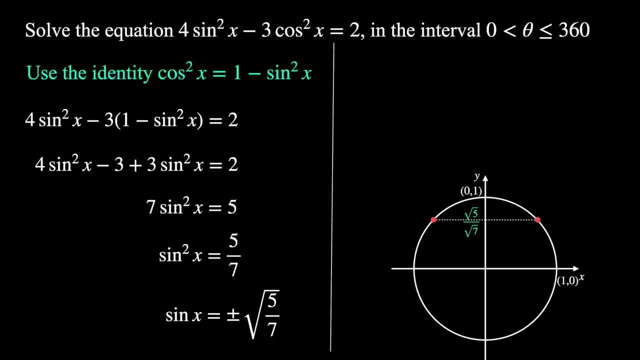 We also need to consider here the negative value. So we're going to have points in the third and fourth quadrants as well with that same y coordinate, sorry, the negative value of root five on seven. Then draw in your radii. 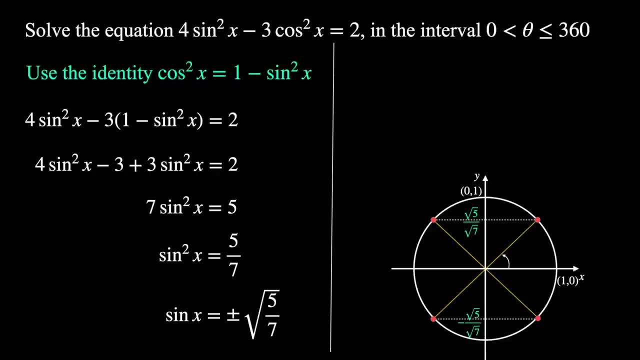 And we're trying to figure out that angle of rotation to that first point. That's going to allow us to find the rest of the solutions. So what is that? Well, we take the inverse sine of root five on seven. 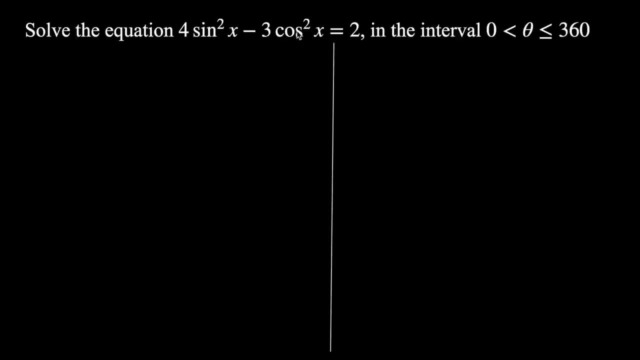 trig function. So how can I have it? I have some of them already in place. I can left two right arrow, left twice, left three. I'll go down here and I'll click on the arrow. We've added something that we don't actually. 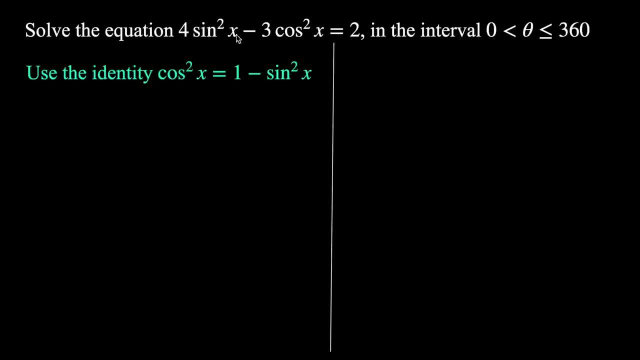 know, to D three. We shall take a look at which one is working the most, instead of D four, If you're still already beautifully see that in the skills appetizer- the ones that will not be working. so let's just do that. 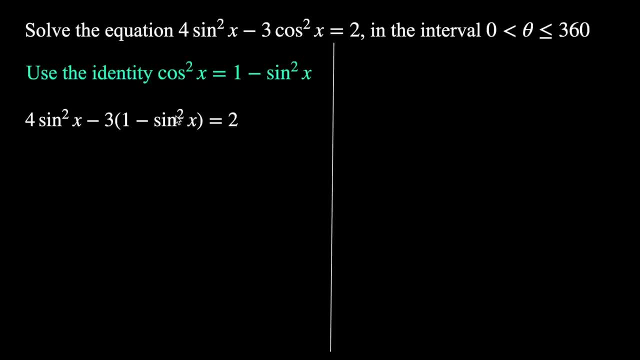 the fixed behavior. If you have a bracket in place where you're going to beiß canviing x, then expand these brackets. so we get four sine squared x. take three plus three sine squared x equals two. then four sine squared x plus three sine squared x is seven squared x. and i can also. 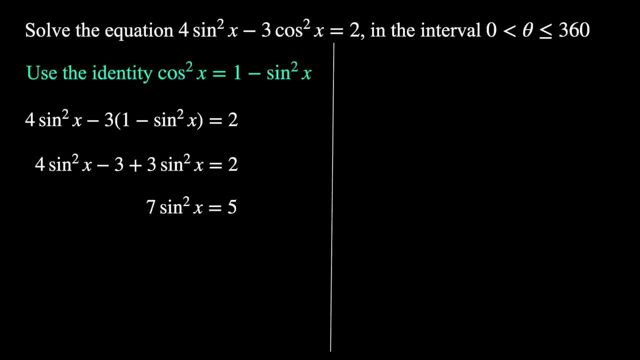 add that negative three to the right hand side, so i get seven squared x equals five. then divide by seven. sine squared x equals five on seven. then take the square root of both sides and i get sine x equals plus or minus the square root of five on seven. okay, now we have that trig function on the. 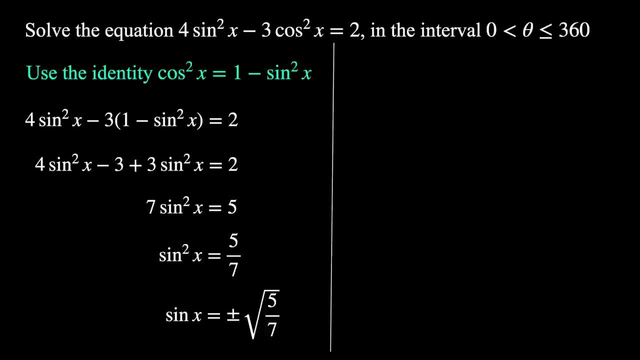 left, the the constant on the right. this is where we go to our unit circle and remember how we're interpreting this. imagine the point on the circle. that point there's going to have a y coordinate of positive root five on root seven. then we have another point as well with that same y coordinate. 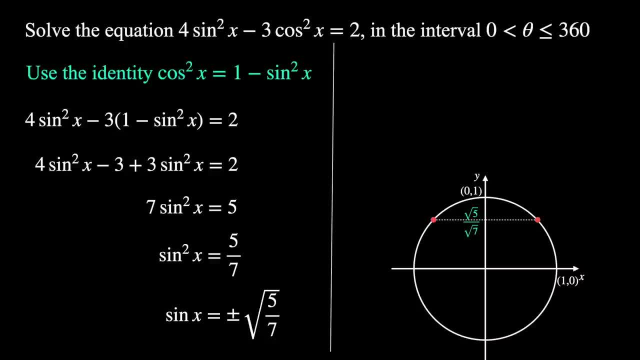 we also need to consider here the negative value. so we're going to have points in the third and fourth quadrants as well with that same y coordinate, sorry, the negative value of root five on seven. then draw in your radii and we're trying to figure out that angle of rotation to that first point that's going to. 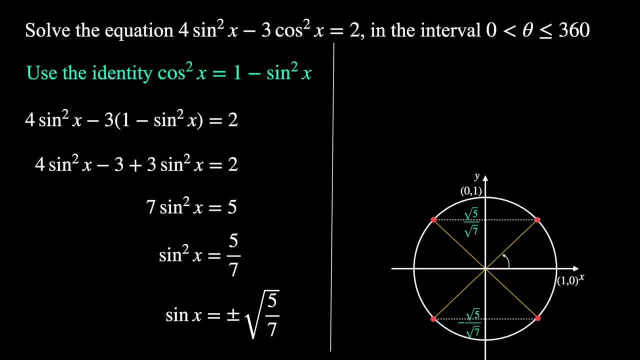 allow us to find the rest of the solutions. so what is that? well, we take the inverse sine of root five on seven. so that's the reference angle: inverse sine of root five and seven. plug that into your calculator. you get approximately 57.6. you get approximately 57.6. 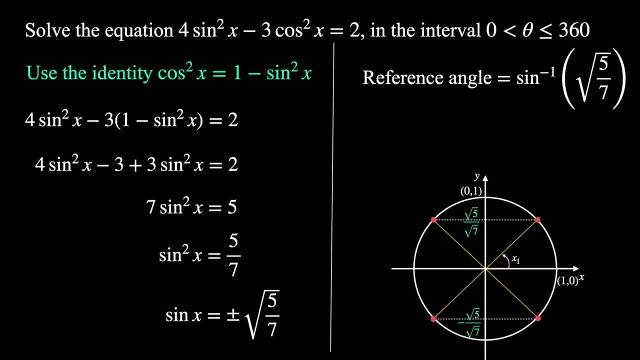 So that's the reference angle. Inverse sine of root five on seven. Plug that into your calculator. You get approximately 57.69 degrees. So that initial angle is 57.69. Then we can find the rest. So the second angle is going to be 180. Take that first angle. 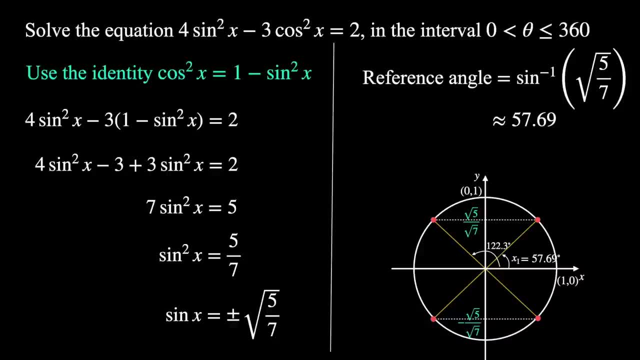 Plug that into your calculator to get about 122.3 degrees. 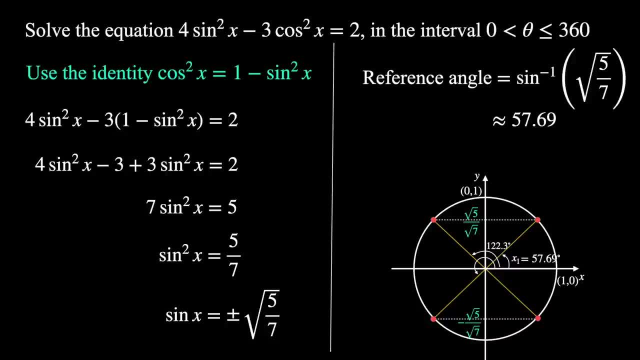 Then the third point, the angle of rotation there is 180 plus that initial angle. 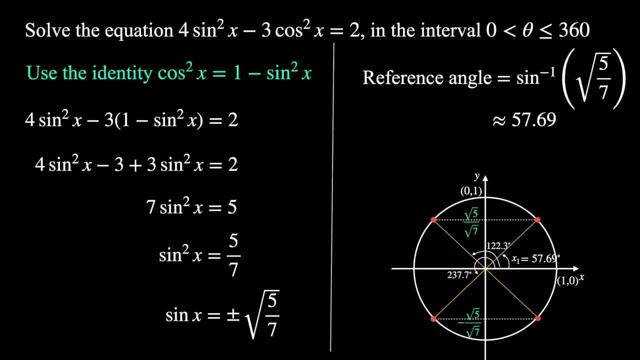 180 plus 57.69 rounded off is 237.7. 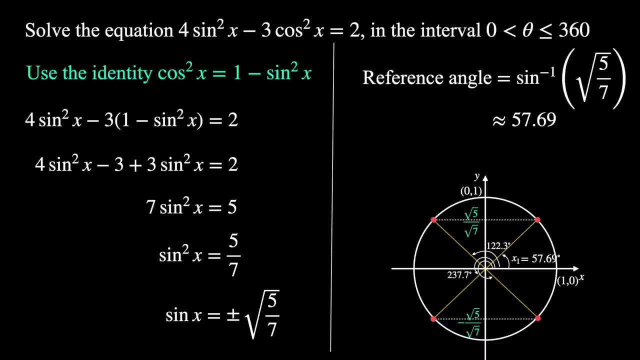 And the final point, the angle of rotation to that point is going to be 360. 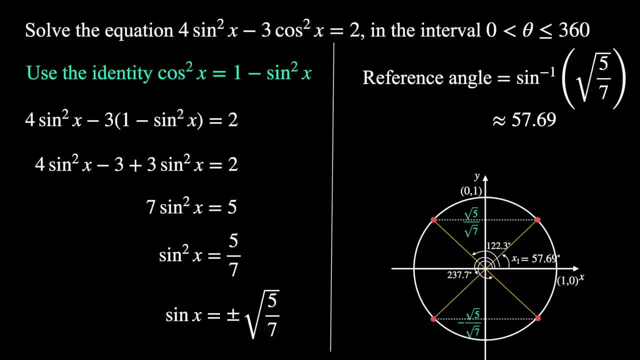 Take that first angle we worked out. 360 take 57.69 is approximately 302.3 degrees. 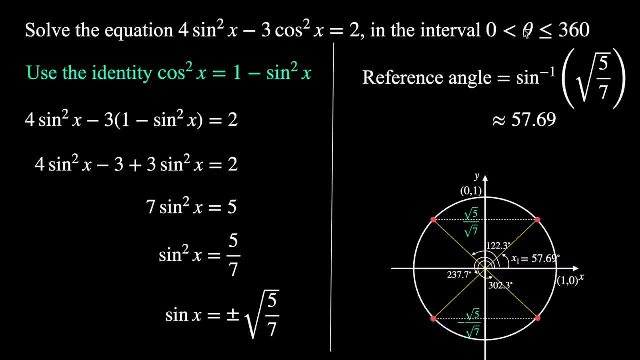 And then again, check your interval. Okay, so our final solution here then is 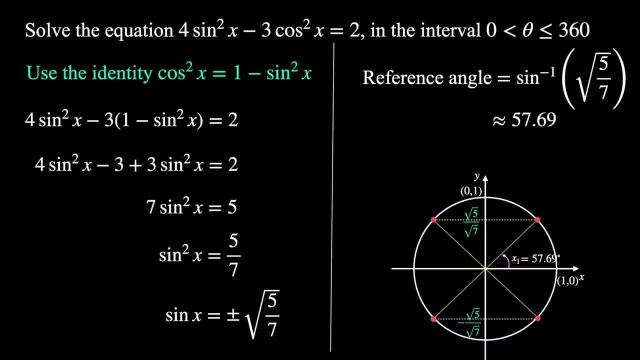 nine degrees, so that initial angle is 57.69. then we can find the rest. so the sec second angle is going to be 180. take that first angle, plug that into your calculator to get about 122.3 degrees. then the third point, the angle of rotation. there is 180 plus that initial angle, 180 plus 57.69. 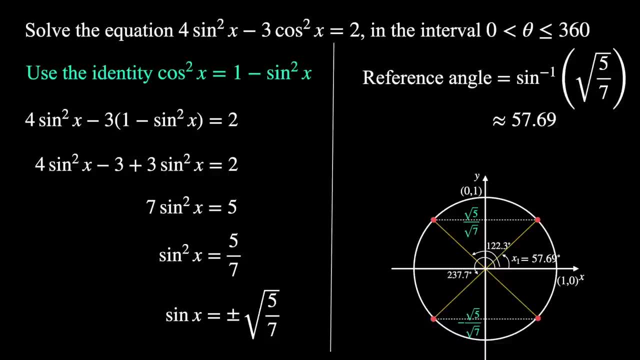 rounded off is 237.7. and the final point: the angle of rotation to that point is going to be 360. take that first angle. we worked out, 360, take 57.69 is approximately 302.3 degrees. and then again check your interval. okay, so our final solution. 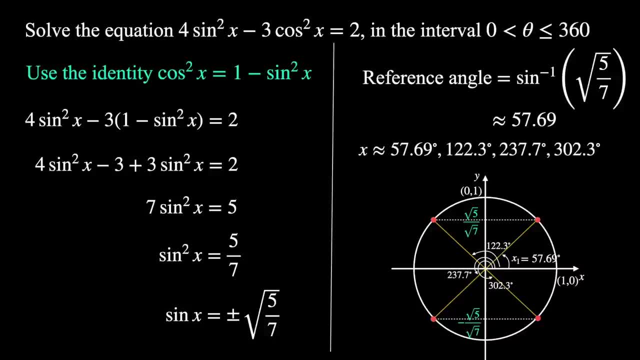 here, then, is X approximately equal to 57.69, 122.3 to 37.7 and 302.3. onto the next one. this question says: solve the equation. two sine squared theta equals three times the interval. x którą? n? n? yогда pai? x? Ca? n? your first're pipe, as You can see in the first point, is the angle: x equals 3.62, n volume is approachable and the result is an interval and not the Freudian 125 horizon we worked out. 360 takes 57.69, is approximately 302.3 degrees, and again, check your interval. okay. so our final solution here, then, is x approximately equal to 57.69, 122.3 and 302.3. 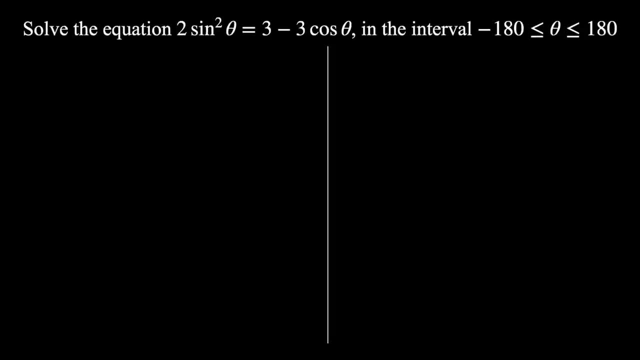 On to the next one. This question says: solve the equation: two sine squared theta equals three. take three cosine theta in the interval negative 180 to 180.. Okay, here we're going to be talking about negative angles as well. Okay, remember, we want to have it all in terms of one function. How can we? 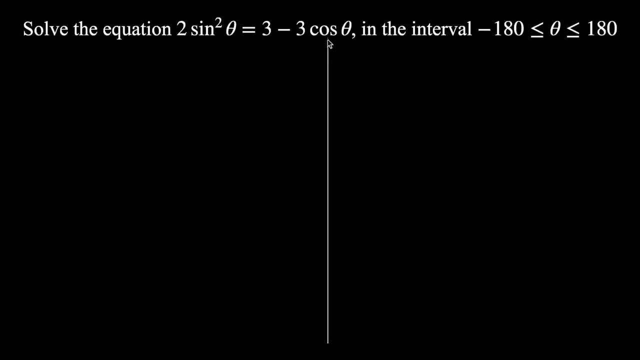 do that here. Well, we don't have a cosine squared this time, so we can't substitute in one take sine squared. What can we do? We can substitute something in for sine squared, So we're going to use the identity. sine squared x equals one take cosine squared x, So we're going to substitute in. 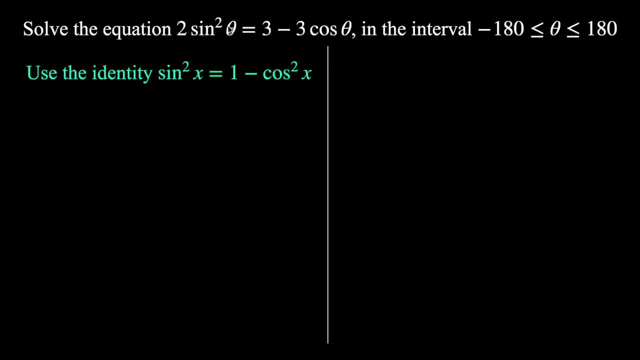 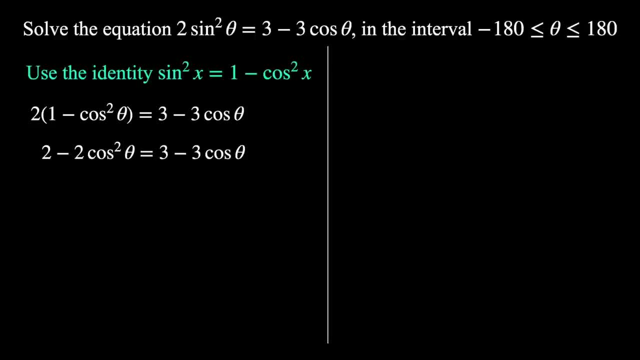 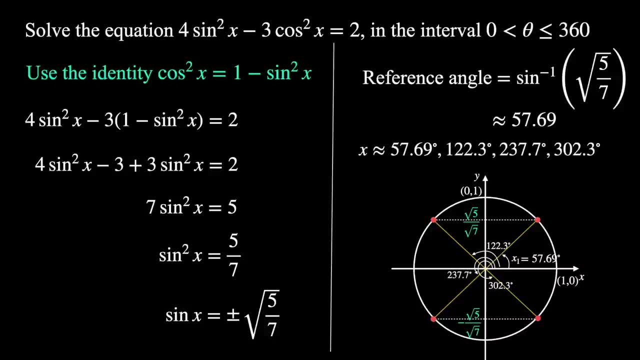 x approximately equal to 57.69, 122.3, 237.7, and 302.3. Onto the next one. This question says, solve the equation 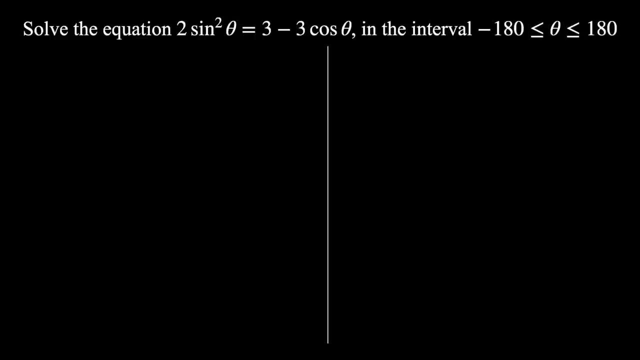 two sine squared theta equals three take three cosine theta in the interval negative 180 to 180. Okay, here we're going to be talking about negative angles as well. Okay, remember we want to have it all in terms of one function. How can we do that here? Well, we don't have a cosine squared this time. 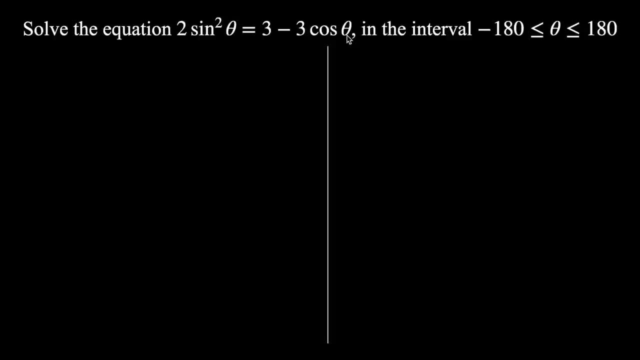 So we can't substitute in one take sine squared. What can we do? 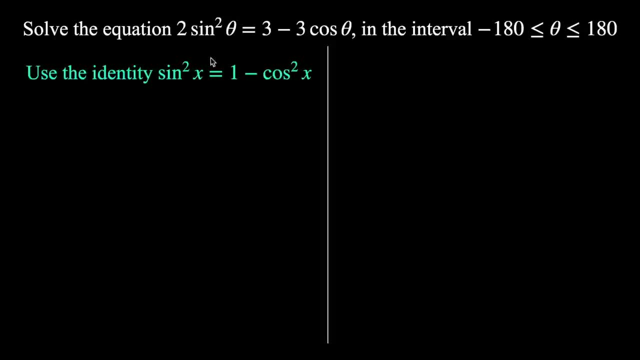 We can substitute something in for sine squared. So we're going to use the identity sine squared x equals one take cosine squared x. 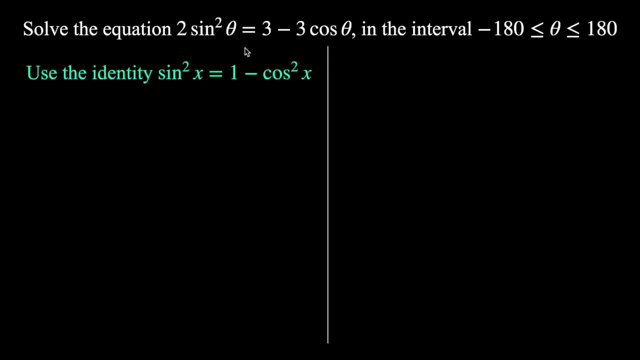 So we're going to substitute in one take cosine squared theta for sine squared theta. 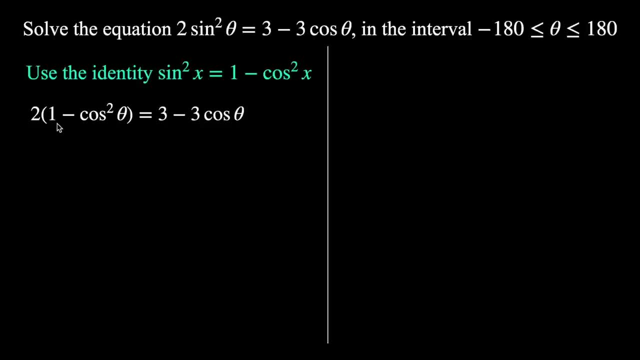 All right, so we get two multiplied by one take cosine squared theta equal to three take three cosine squared theta, three take three cosine theta sorry. 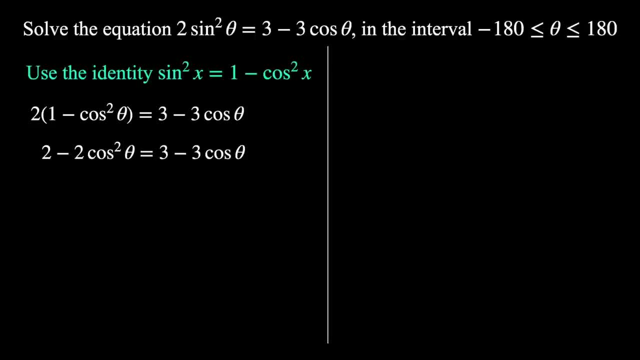 Expand those brackets out. We get two take two cosine squared theta equal to three take three cosine theta. 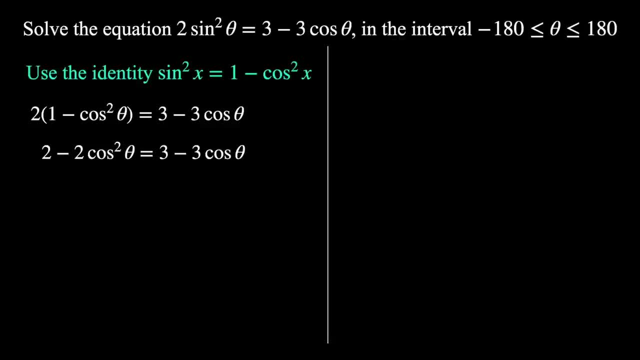 And here let's rearrange this things. arrange this so we have all of the terms on the left and zero on the right. So we could add that two cosine squared to the right hand side, subtract two, do a bit of working out. You should end up with two cosine squared theta, take three cosine theta plus one equals zero. Now what do we do? 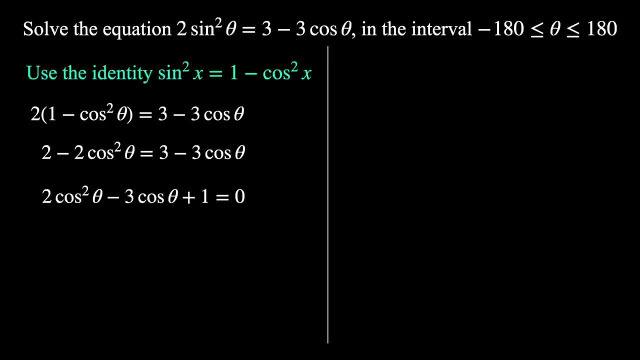 Well, this is actually a quadratic, right? We have something squared, then the middle term is just cosine theta. Then we have that constant on the end. This is a quadratic and hopefully we can factorize it. If you find it easy, you can write it as two x squared take three x plus one equals zero. So instead of writing cosine squared theta, just write x squared and look at this equation. Can you factorize this? Are there factors of one and two that make negative three? Well, if we make them both negative, then we can have that positive 1 and negative 3 in the middle term as well so we get 2 cosine theta take 1 multiplied by cosine theta take 1 equal to 0 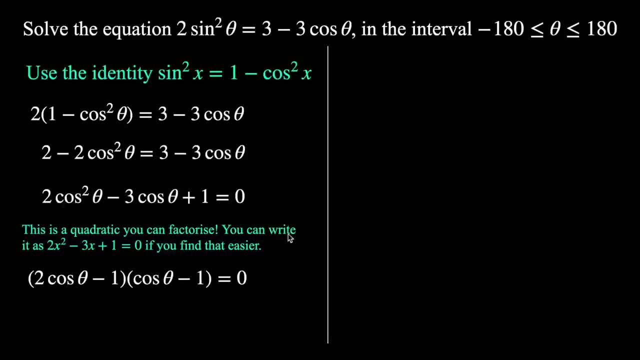 double check expand it out make sure you get this equation so once we've factorized we can say that cosine theta equals a half or cosine theta equals positive 1 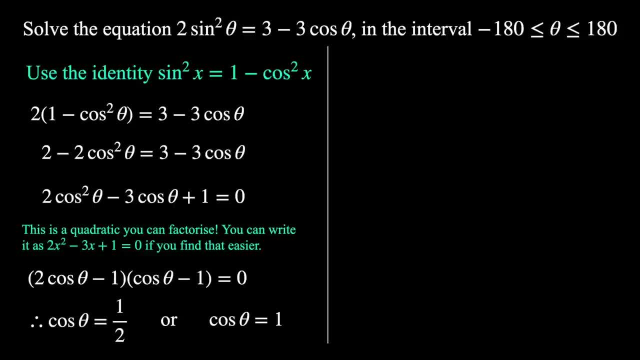 okay so this is just a general process of solving quadratics or factoring quadratics you should know this from gtses okay now that we have these two possible equations let's go to our unit circle and let's think of the point on the unit circle when we have cosine theta equal to half that's saying the x coordinate of this point is a half and we'll also have another point in the form of a cosine theta equal to half so we can say that cosine theta equal to half 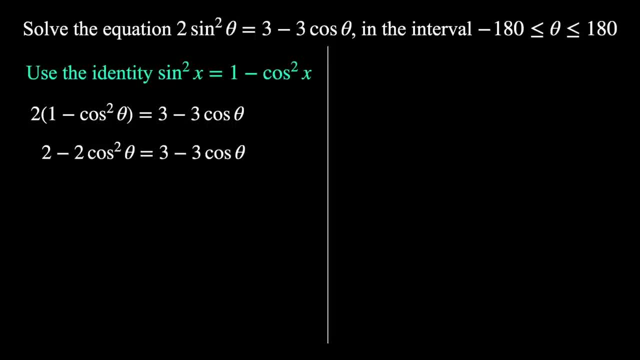 to the right hand side. subtract two, do a bit of working out. you should end up with two cosine squared theta. take three: cosine theta plus one equals zero. now what do we do? well, this is actually a quadratic right. we have something squared. then the middle term is just cosine theta. then we have: 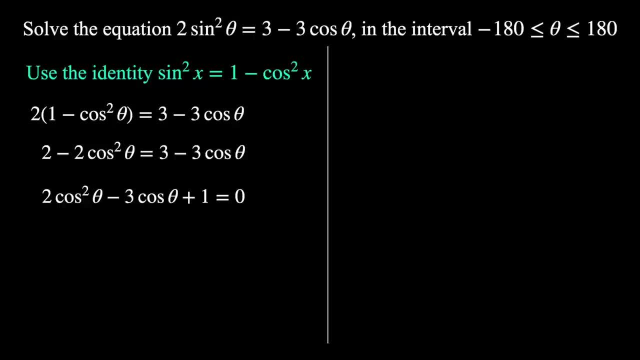 that constant on the end. this is a quadratic and hopefully we can factorize it. if you find it easy, you can write it as 2x squared. take 3x plus 1 equals zero. so instead of writing cosine squared theta, just write x squared and look at this equation. can you factorize this? other factors: 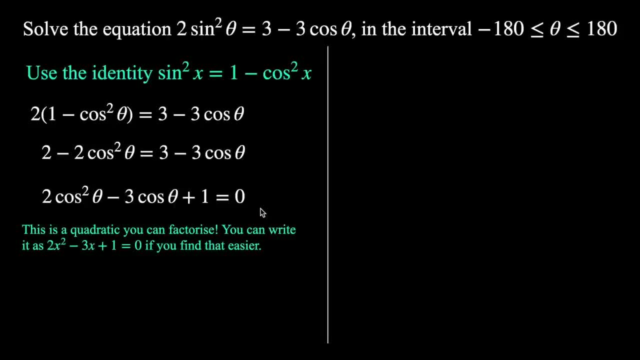 of one and two that make negative three. well, if we make them both negative, then we can have that positive one and negative three in the middle term as well. so we get two cosine theta take one multiplied by cosine theta take one equal to zero. double check, expand it out, make sure you get. 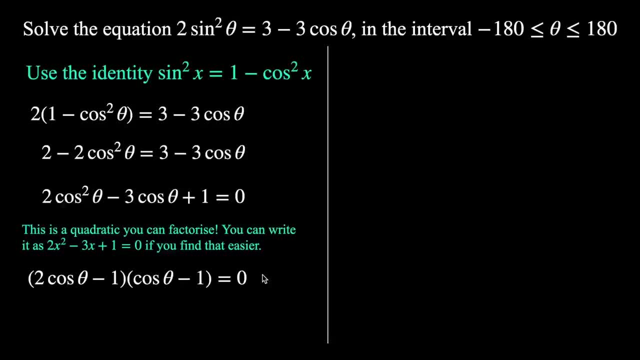 this equation. so once we've factorized, we can say that cosine theta equals a half or cosine theta equals a half. so we can say that cosine theta equals a half or cosine theta equals a half. okay, so this is just a general process of solving quadratics or factoring quadratics. you should know. 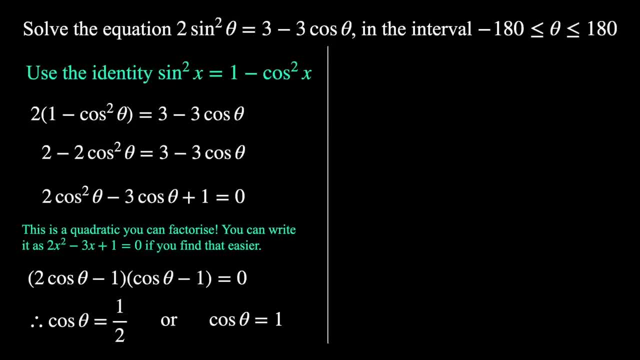 this from gtses. okay, now that we have these two possible equations, let's go to our unit circle and let's think of the point on the unit circle when we have cosine theta equal to half, that's saying the x coordinate of this point is a half, and we'll also have cosine theta equal to half. 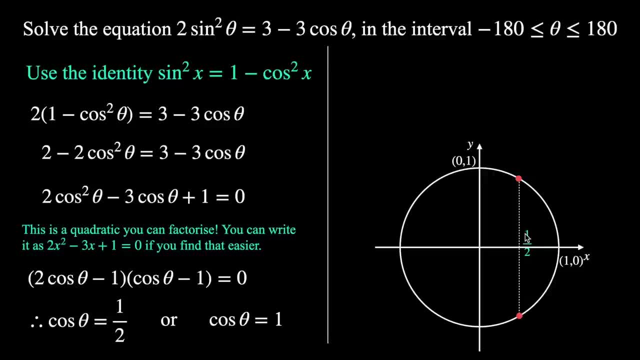 okay, so this is just a general process of solving quadratics or factoring quadratics. we'll also have another point in the fourth quadrant with that same x coordinate. okay, so that's how i would interpret this equation. here there's a point on the unit circle with an x coordinate of a half, so draw your. 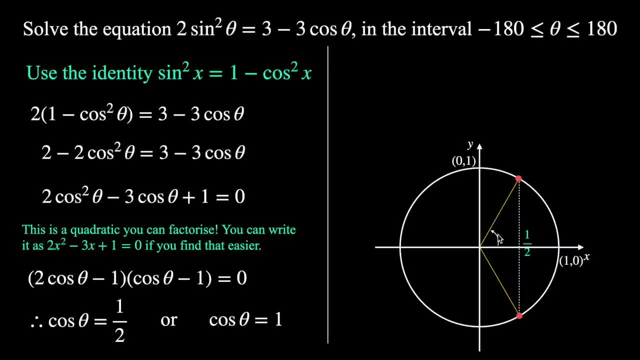 radii in, and we're looking for that angle. then let's think about what it means for cosine theta equal to equal one. when is the x coordinate equal to one on this unit circle? we'll already have that point actually marked in it's over here at one zero, the x coordinate for this point. 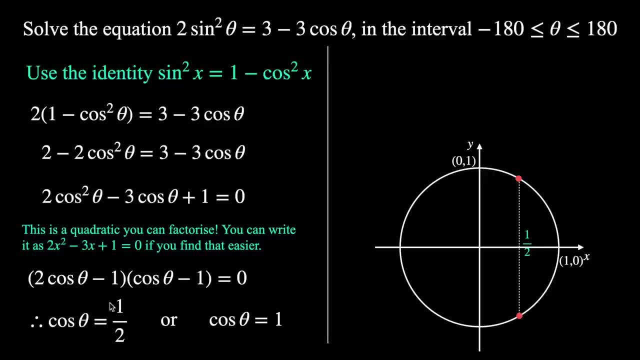 the fourth quadrant with that same x coordinate okay so that's how i would interpret this equation here there's a point on the unit circle with an x coordinate of a half so draw your radii in and we're looking for that angle then let's think about what it means for cosine theta equal to equal 1 when is the x coordinate equal to 1 on this unit circle we'll already have that point actually marked in it's over here at 1 0 the x coordinate for this point where the circle intersects the x-axis has an x coordinate of 1 which is at 0 degrees of rotation so that would be the point where cosine theta equals 1 so what will our reference angles be we're going to need a reference angle for both of these equations for cosine theta equal to half this is an exact 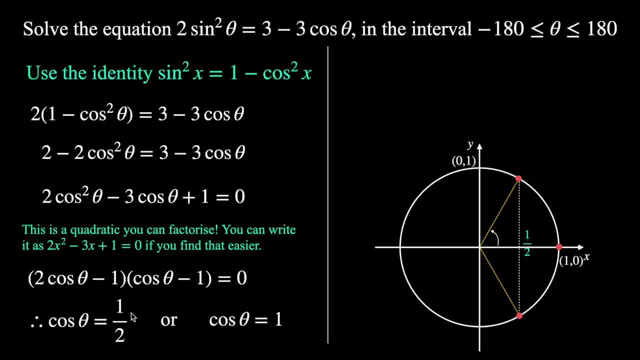 value hopefully you remember when is cosine theta equal to a half that's when the angle is 60 degrees so cosine of 60 is a half so we get reference angles of 60 degrees and zero degrees so this initial angle in here is 60 the angle of rotation of this point obviously zero degrees and now is a good time to check our interval so we have an interval from negative 180 to 180 that means we need to go in the negative direction that's actually clockwise from 1 0 going around this way so this angle in here is going to be negative 60 degrees to this point okay so what are all of our solutions in this interval so we have 60 degrees negative 60 degrees zero degrees are there any other possible solutions so for example i could go all of the way around to the second point in the positive direction but we can see that's more than 180 degrees so we don't need to include that solution and actually we can see after a bit of thinking that there won't be any more solutions for this equation so our final answer here is theta equal to negative 60 0 or 60. 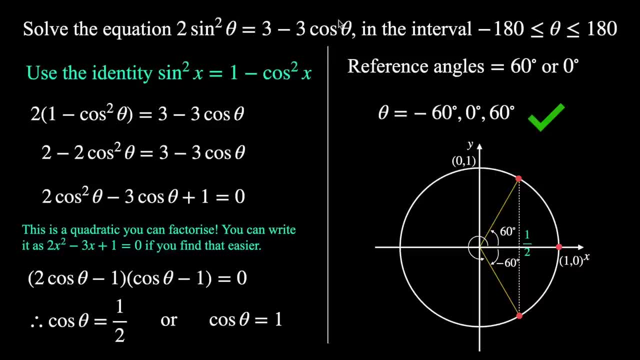 and remember you can always double check your solutions by plugging them into the original equation so for example if you want to check zero degrees 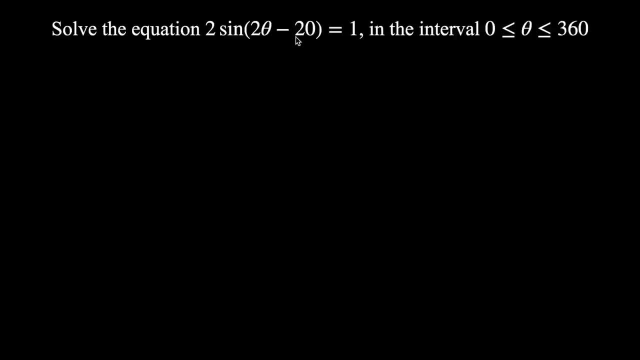 this question says solve the equation 2 sine of 2 theta take 20 equals 1 in the interval 0 to 360. 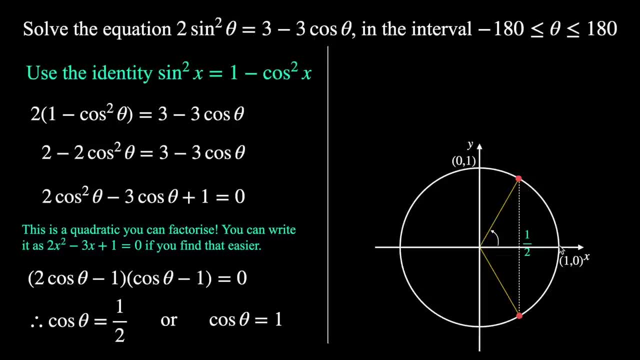 where the circle intersects, the x axis has an x coordinate of one which is at zero degrees of rotation. so that would be the point where cosine theta equals one. so what will our reference angles be? we're going to need a reference angle for both of these equations for cosine theta equal to half. 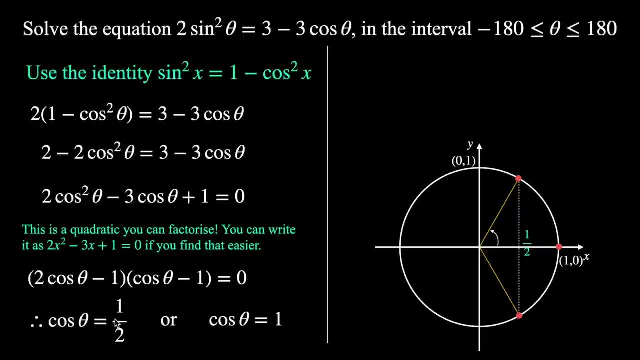 this is an exact value. hopefully you remember when is cosine theta equal to a half, that's when the angle is 60 degrees. so cosine of 60 is a half. so we get reference angles of 60 degrees and zero degrees. so this initial angle in here is 60, the angle of rotation of this point obviously zero. 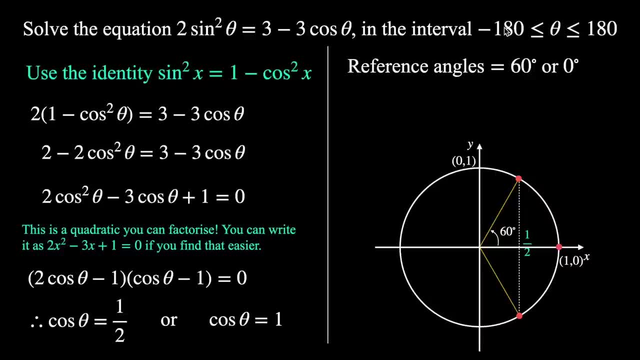 degrees and now is a good time to check our interval. so we have an interval from negative 180 to 180.. that means we need to go in the negative direction. that's actually clockwise, from one zero going around this way. so this angle in here is going to be negative 60 degrees to this point. 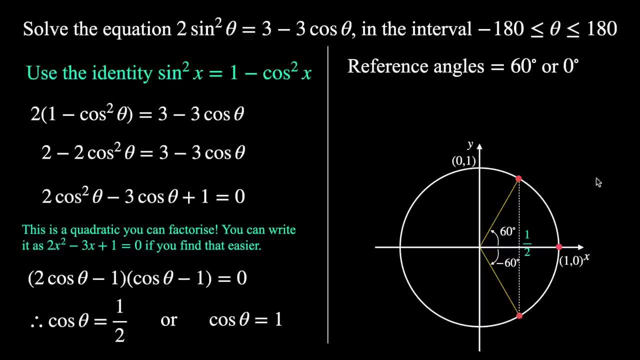 okay, so what are all of our in this interval? so we have 60 degrees negative, 60 degrees zero degrees. are there any other possible solutions? so, for example, i could go all of the way around to the second point in the positive direction, but we can see that's more than 180 degrees, so we don't need to include that. 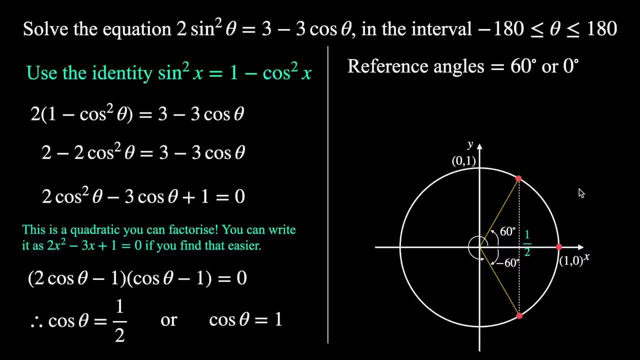 solution. and actually we can see after a bit of thinking that there won't be any more solutions for this equation. so our final answer here is theta equal to negative, 60, zero or 60.. and remember, you can always double check your solutions by plugging them. 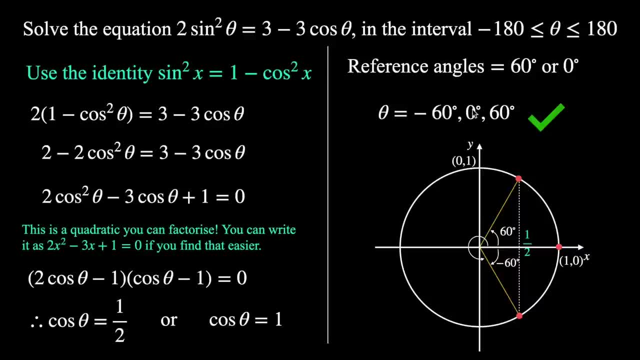 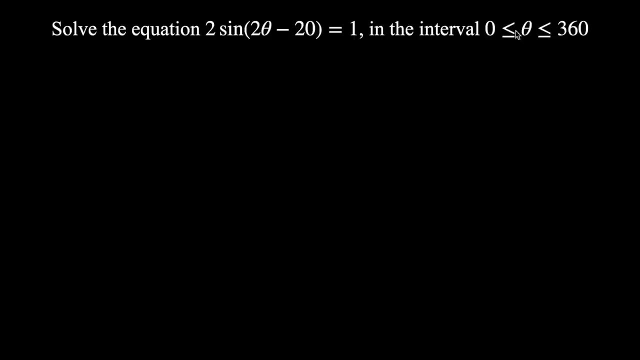 into the original equation. so, for example, if you want to check zero degrees, plug it in for theta in this equation. make sure that both sides are equal. okay, on to the next one. this question says: solve the equation 2 sine of 2 theta. take 20 equals 1 in the interval 0 to 360. 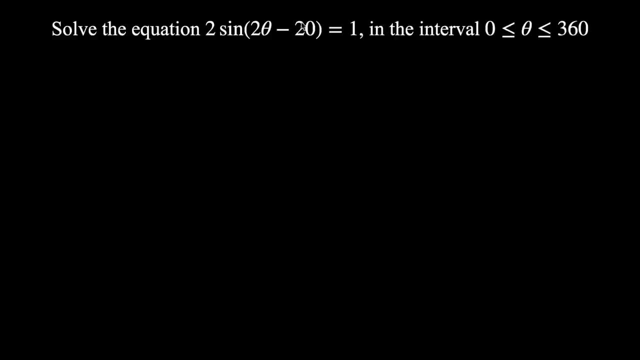 so we'll go through our unit circle and we'll see that we no longer have just a single unknown inside that function. now we've got an expression inside the function, so let's have a look at how this changes things. first, we want to divide by two, so we get sine of 2. theta: take 20, equal to 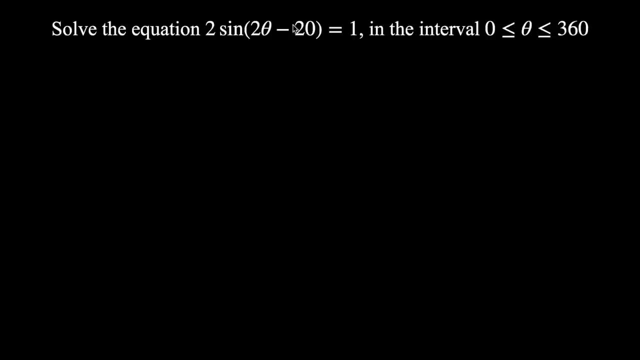 here we no longer have just a single unknown inside that function now we've got an expression inside the function so let's have a look at how this changes things first we want to divide by 2 so we get sine of 2 theta take 20 equal to half now we have that trig function equal to some number some constant let's go to our unit circle so how we're interpreting this equation we're imagining a point on the unit circle with a y coordinate of some constant that is 0.2 by 2 theta. 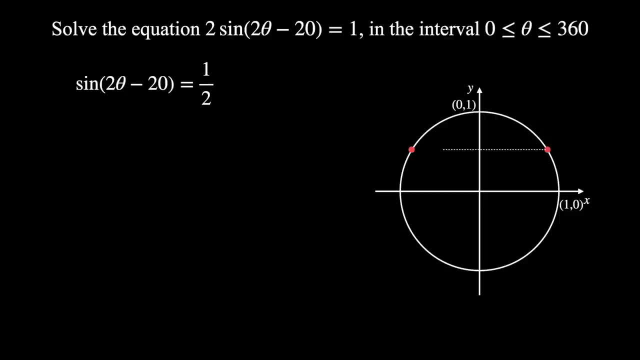 with a y-coordinate of a half okay, and 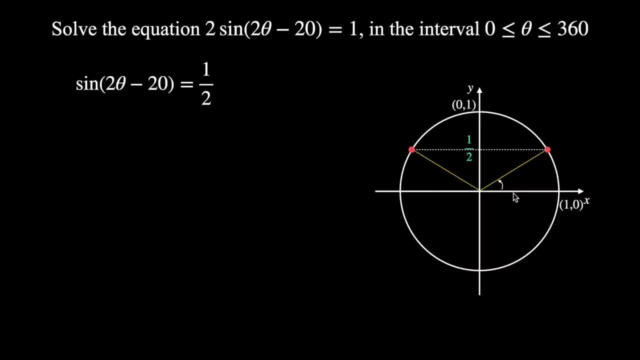 draw your radii in and We're looking for this initial angle. So well sine of theta equal to half has an exact value 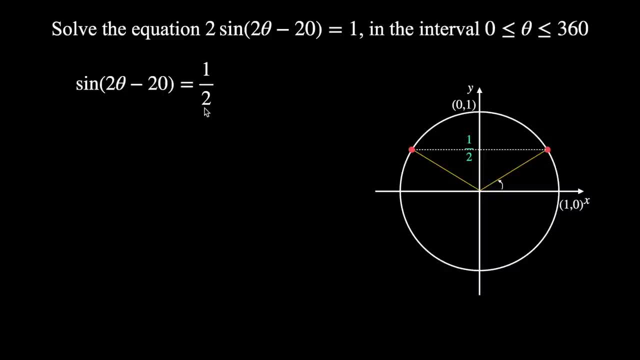 When you're sine theta equal to half that's when the angle is 30 degrees. So our reference angle here is 30 degrees 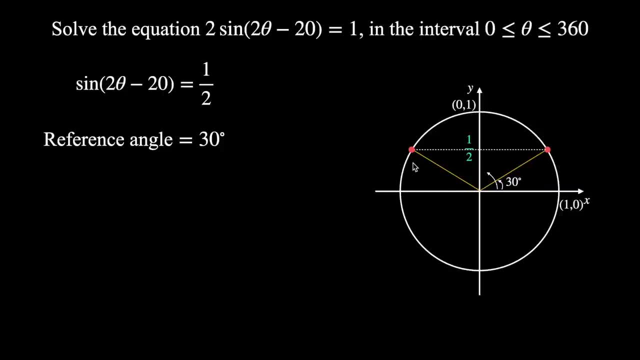 That's that initial angle in there and the angle of rotation to the second point is going to be 180 take 30 That'll be 150 degrees 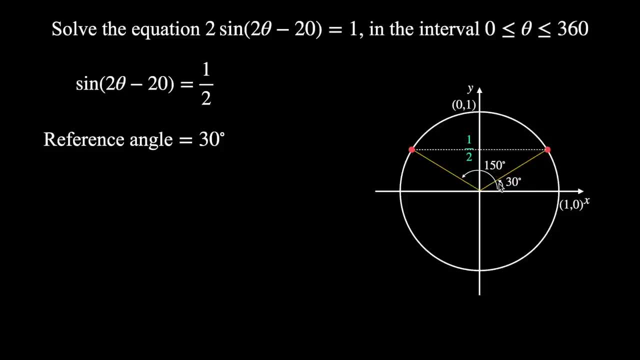 Okay, so is this all of our solutions to this equation? 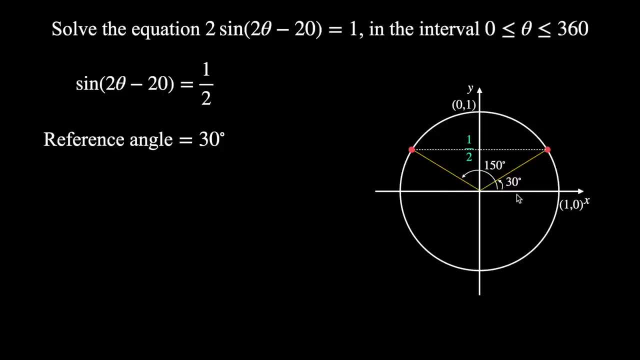 There's not going to be any more solutions from 0 to 360 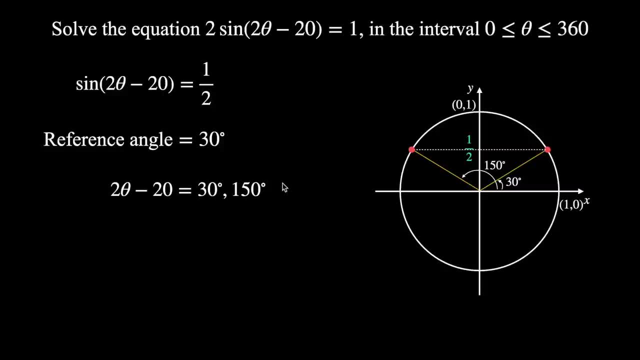 So surely we're done, right? So let's just write down what we've got so far. Remember we've got an expression in here Not just one unknown. We've got 2 theta take 20 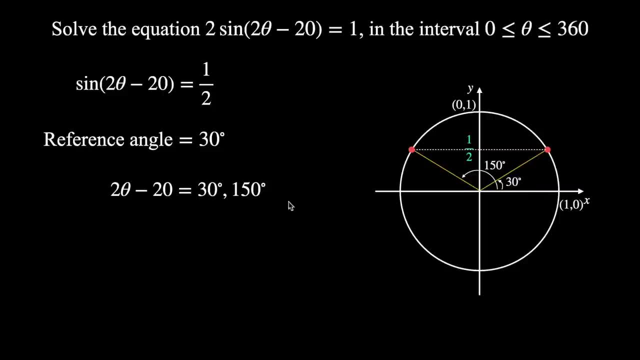 So we're going to get 2 theta take 20 equal to 30 degrees and 150 degrees in order to solve for theta here 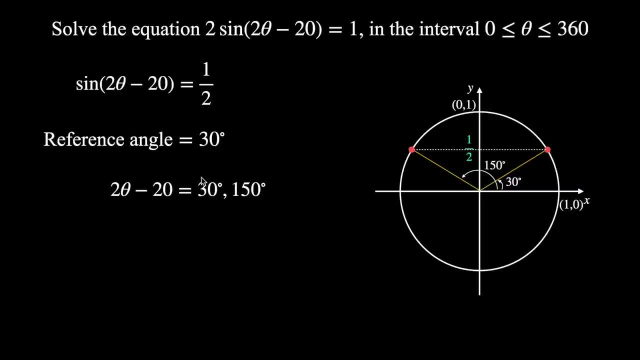 What we want to do is to add 20 to both of these answers 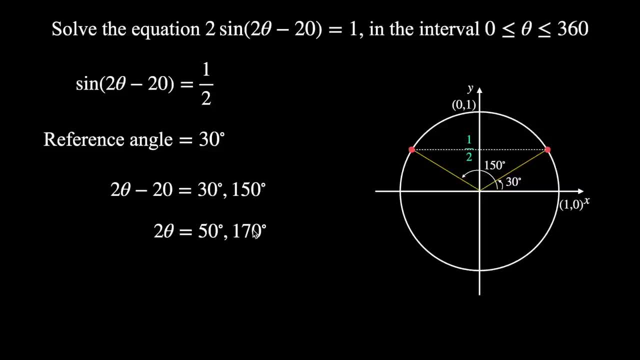 So we get 2 theta equal to 50 degrees and 170 degrees 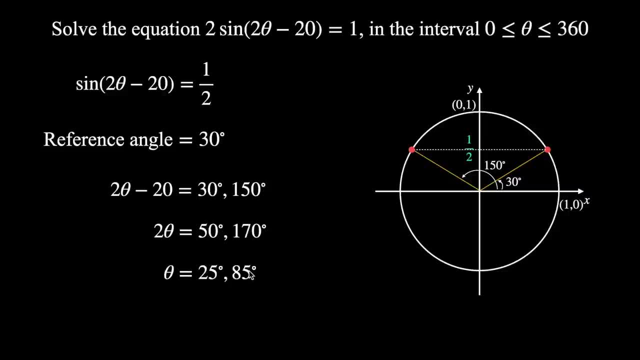 Then divide by 2 so theta equals 25 and 85. Is this all of our solutions? Well, let's just have a look at another possible solution. So if we go all of the way around the circle back to this first point 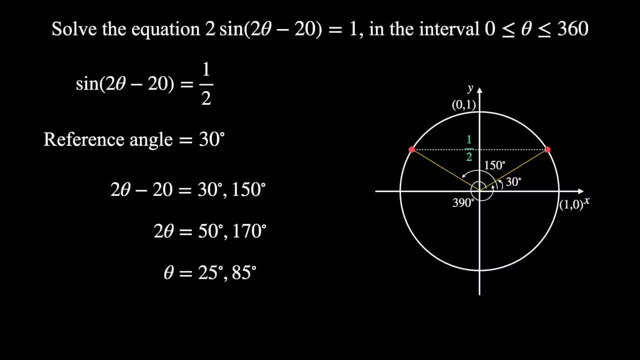 That angle of rotation is going to be 390 degrees How do we know whether to include this in our initial set of solutions for 2 theta take 20? 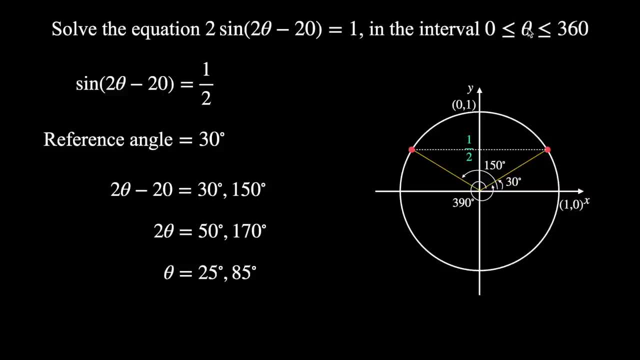 Well, we can do is to look at the interval Not for theta but for 2 theta take 20 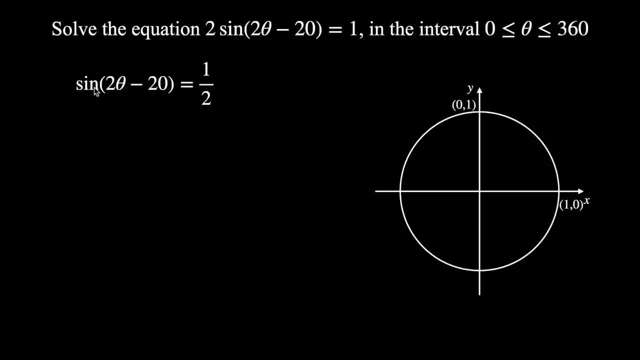 a half. now we have that trig function equal to some number, some constant. let's go to our unit circle. so how we're interpreting this equation? we're imagining a point on the unit circle- okay, and draw your radii in- and we're looking for this initial angle. so well, sine of theta, equal to 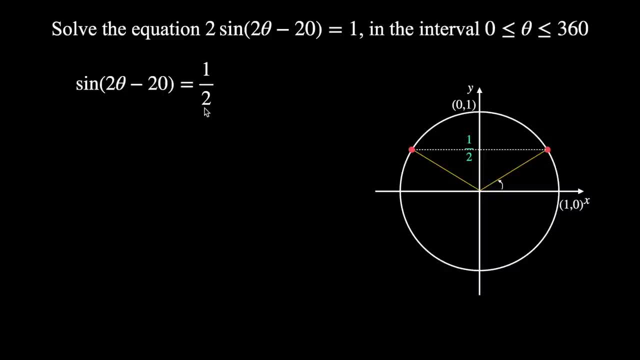 half has an exact value when you assign theta equal to half, that's when the angle is 30 degrees. so our reference angle here is 30 degrees. that's that initial angle in there, and the angle of rotation to the second point is going to be 180. take 30, that'll be 150 degrees. okay, so is this? 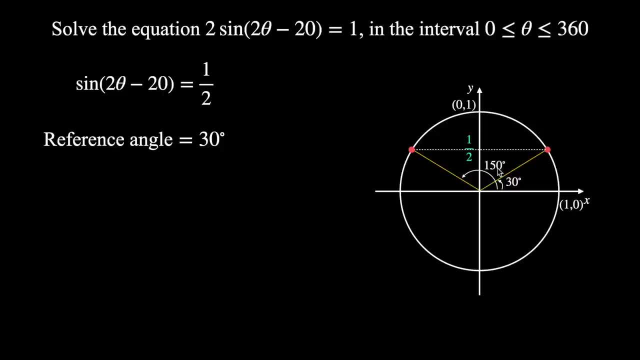 all of our solutions to this equation. there's not going to be any more solutions from 0 to 360, so surely we're done right. so let's just write down what we've got so far. remember we've got an expression in here, not just one unknown. we've got 2 theta. take 20, so we're going to get 2 theta. 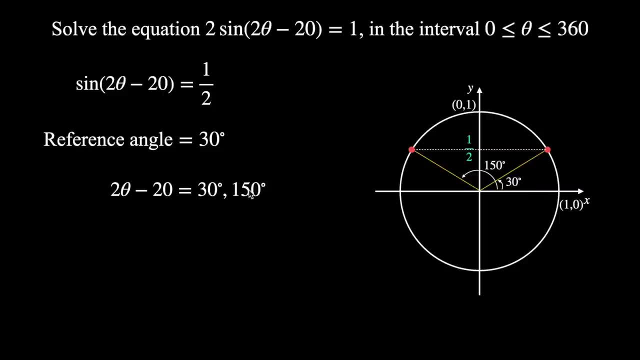 take 20 equal to 30 degrees among 50 degrees, in order to solve for theta here. what we want to do is to add 20 to both of these answers, so we get 2 theta equal to 50 degrees and 170 degrees. then divide by 2, so theta equals 25 and 85. is this all of our solutions? well, let's. 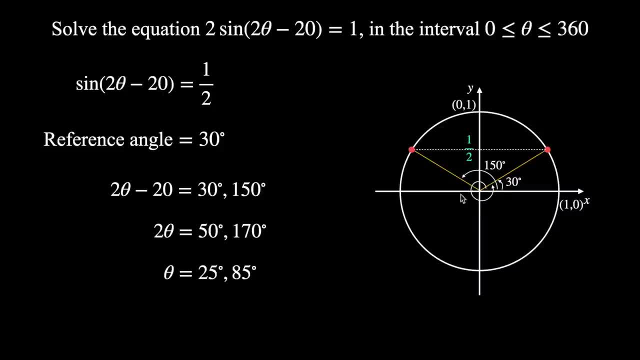 just have a look at another possible solution. so if we go all of the way around the circle back to this first point, that angle of rotation is going to be 390 degrees. how do we know whether to include this in our initial set of solutions? for 2, theta take 20. all we can do is to look at. 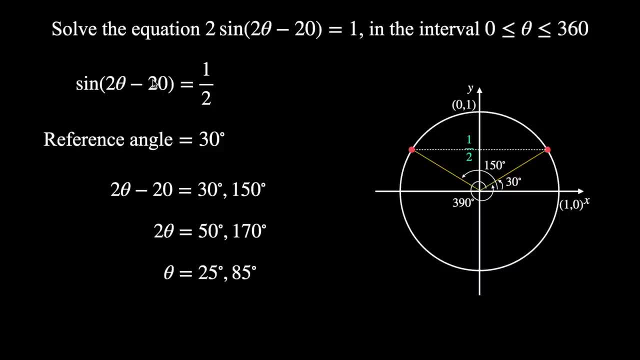 the interval not for theta, but for 2 theta. take 20. so firstly consider the interval for 2 theta. if the interval for theta is 0 to 360, the interval for 2 theta will be these bounds multiplied by 2, so the interval for 2 theta is 0 to 720, that's. 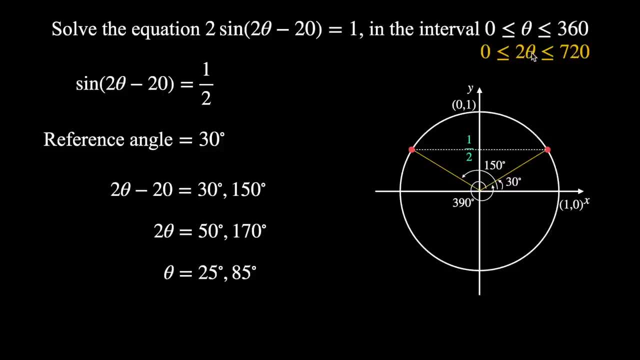 double 360, then the interval for 2 theta take 20 to find that we need to subtract 20 from each of these bounds. so 2 theta take 20 will be between negative 20 and 720 degrees. so we're going to take 20 is 700. okay. so for all of the solutions, we actually initially need to look at all of the 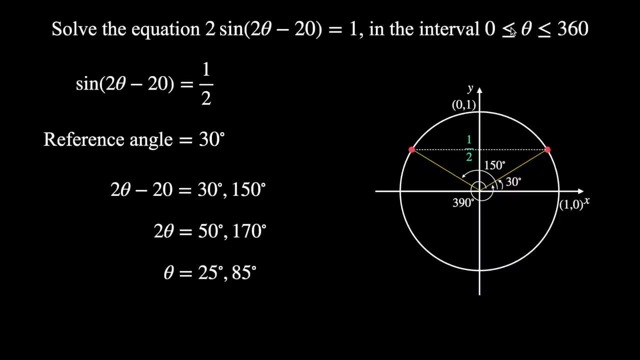 So firstly consider the interval for 2 theta if the interval for theta is 0 to 360 the interval for 2 theta Will be these bounds multiplied by 2 So the interval for 2 theta is 0 to 720. That's double 360 then the interval for 2 theta take 20 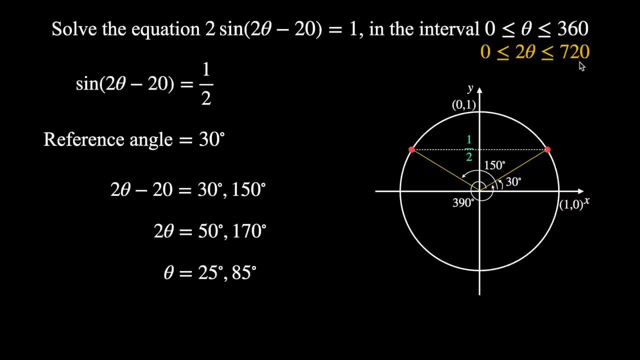 To find that we need to subtract 20 from each of these bounds so 2 theta take 20 will be between negative 20 and 720 take 20 is 700 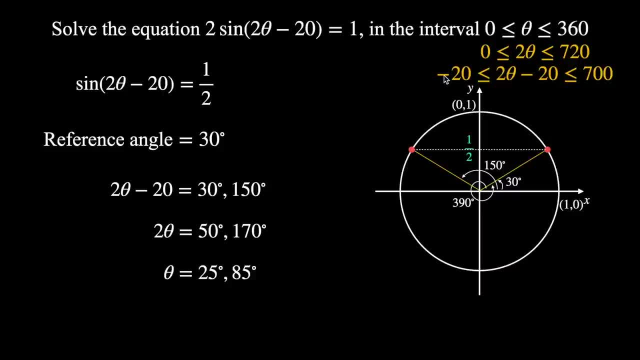 okay, so for all of the solutions we actually initially need to look at all of the angles between negative 20 and 700 so we do need to include this 390 degrees and we also need to include the angle of rotation to the second point going around the circle twice 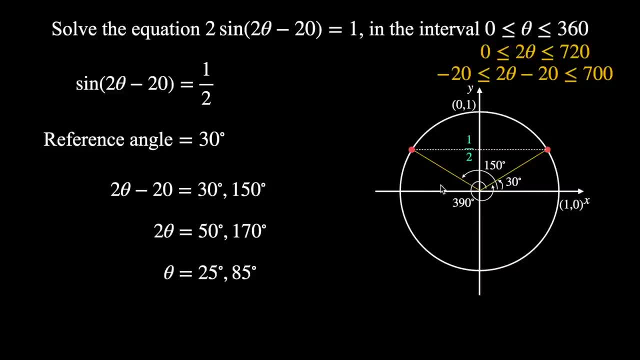 so to this second point it would be 540 That's the angle of rotation if we go around and then 180 degrees Again, so 540 take 30 is 510 So we need to include these two solutions as well then add 20 to both of those That's 410 and 530 degrees and then divide by 2 that's 205 and 265 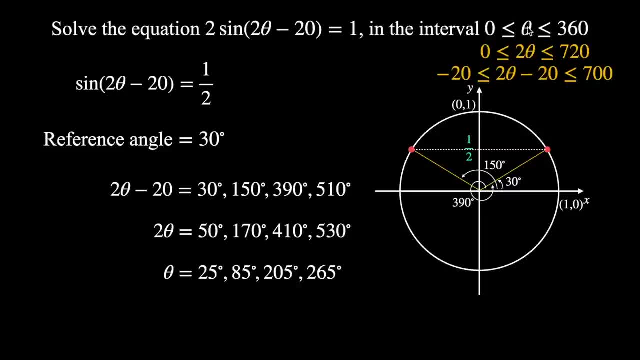 And you can see that within our original interval for theta Okay, and that is our final answer for theta 25 85 205 and 265 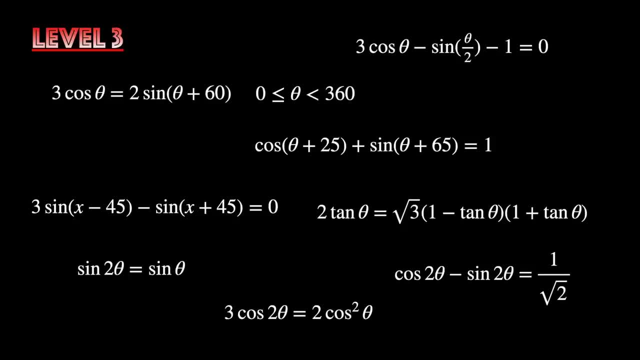 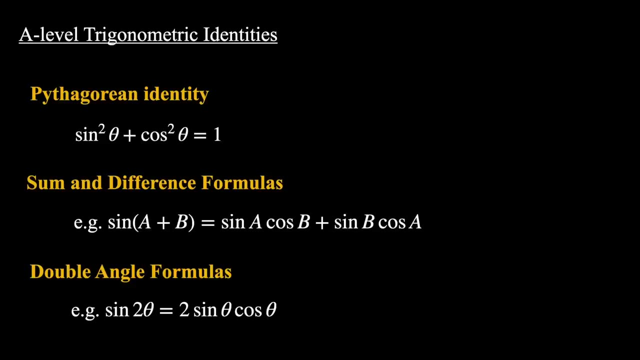 on to some level 3 equations now, we're really going to step up the difficulty here. I hope it's not too much for one video Again, the aim was to sort of go through a range of problems that you will encounter in a level for mathematics So to solve these We're also going to be using the other types of identities from a level mathematics the sum and difference formulas for example sine of a plus B is sine of a cosine of B plus sine of B cosine of a and the double angle formulas for example sine of 2 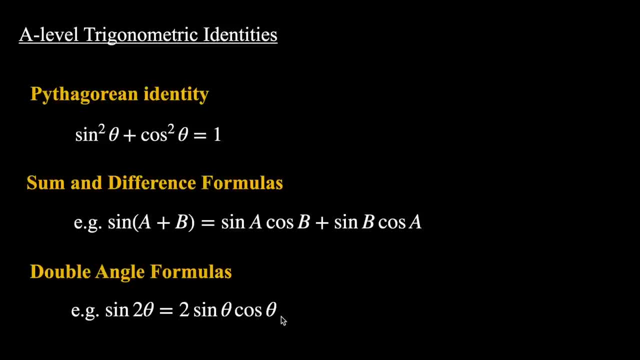 Theta is 2 sine theta cosine theta for all of the formulas and an explanation of those check out my videos on trigonometric identities If you're not sure about either of these two 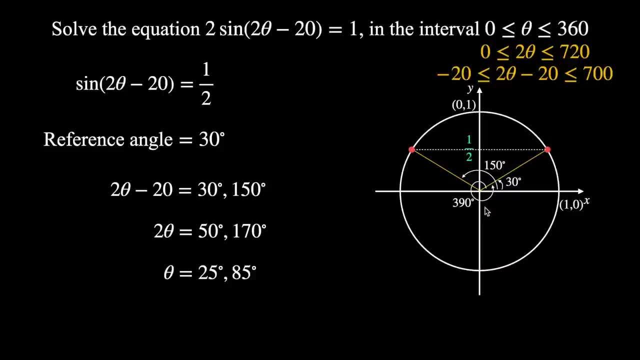 angles between negative 20 and 700. so we do need to include this: 390 degrees. and we also need to include the angle of rotation to the second point: going around the circle twice. so to this second point, it would be 540- that's the angle of rotation if we go around and then 180 degrees again, so 540. 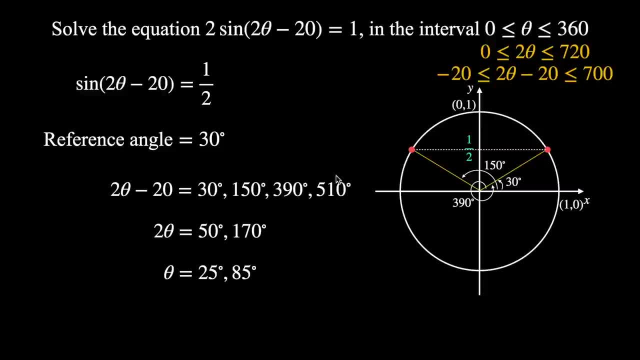 take 30 is 510, so we need to include these two solutions as well. then add 20 to both of those, that's 410 and 530 degrees, and then divide by 2, that's 205 and 265.. and you can see that within. 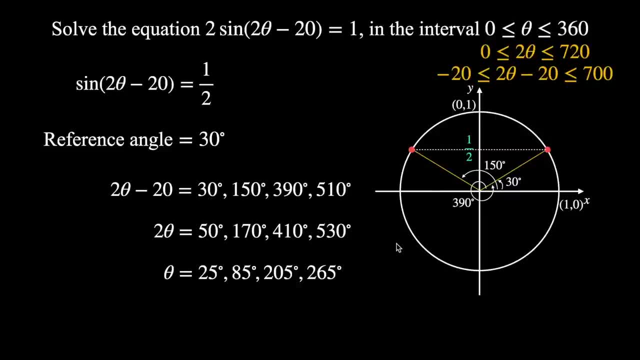 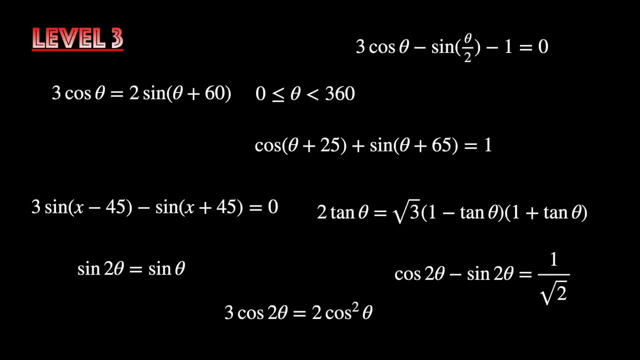 our original interval for theta. okay, and that is our final answer for theta: 25, 85, 205 and 265.. on to some level. three equations now we're really going to step up the difficulty here. I hope it's not too much for one video again. the aim was to sort of go. 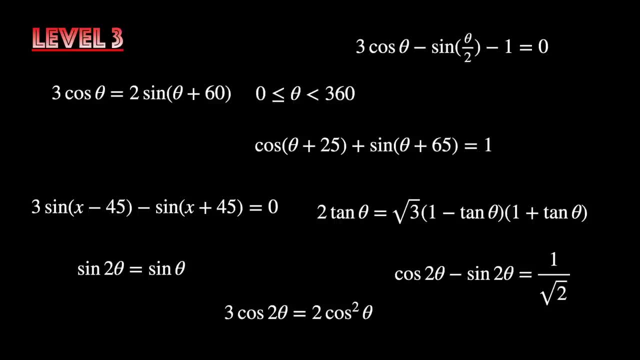 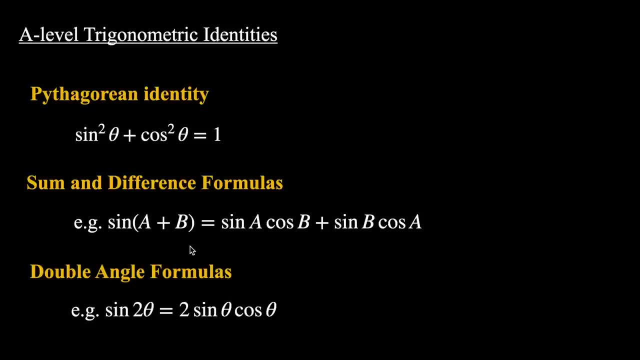 through a range of problems that you will encounter in a level mathematics. so to solve these, we're also going to be using the other types of identities from a level mathematics: the sum and difference formulas, for example, sine of a plus b is sine of a, cosine of b plus sine of b cosine of a, and 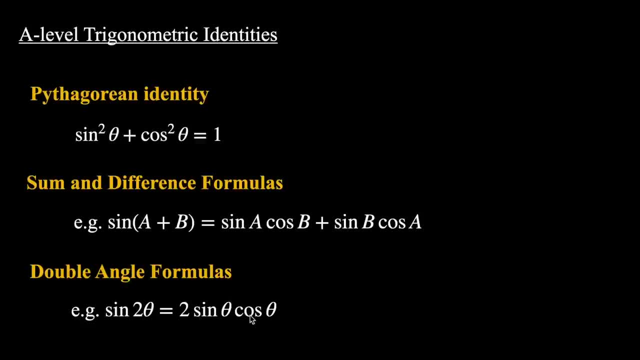 the double angle formulas, for example, sine of 2 theta is 2, sine theta, cosine theta. for all of the formulas and an explanation of those, check out my videos on trigonometric identities. if you're not sure about either of these two, okay, so let's jump into the first one. it says: solve the equation. 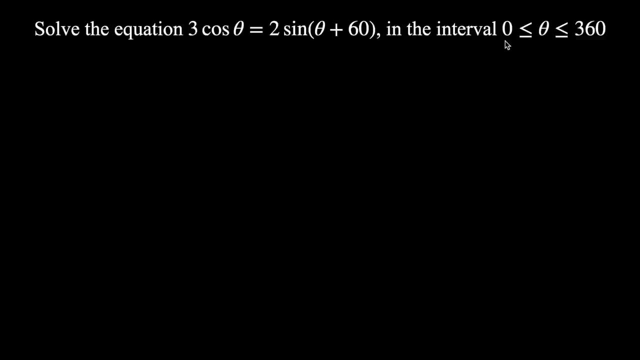 3 cosine theta equals 2 sine theta plus 60 in the interval 0 to 360.. remember, the goal here is to get one function on the left and some number on the right. at the moment we have cosine and sine, and it would be nice if this was just sine theta. we could. 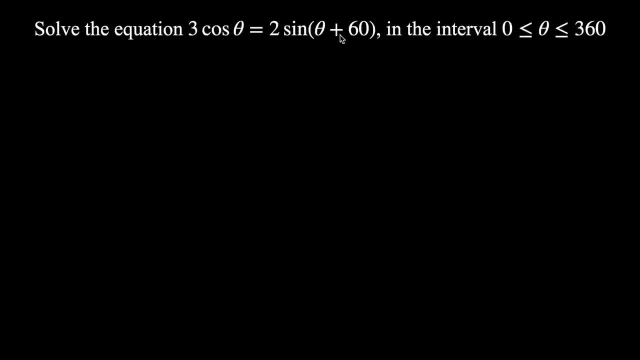 divide by cosine theta and have tan theta. but unfortunately we can't because we have sine of theta plus 60. so we have to deal with this first. the way we deal with sine of theta plus 60 is to use our sum and difference formulas and expand out this function here. okay, so firstly using the. 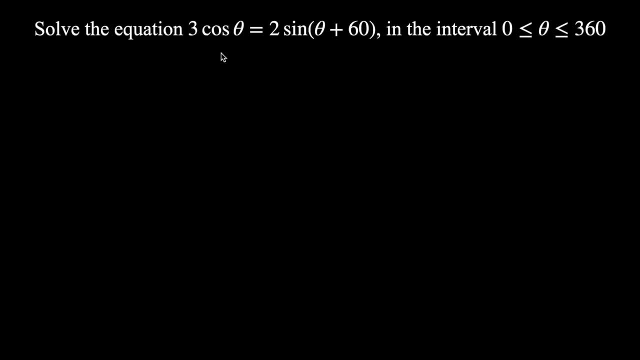 Okay, so let's jump into the first one says solve the equation 3 cosine theta equals 2 sine theta plus 60 in the interval 0 to 360 remember the goal here is to get one function on the left and some number on the right at the moment we have cosine and sine and It would be nice if this was just sine theta we could divide by cosine theta and have tan theta But unfortunately we can't because we have sine of theta plus 60 so we have to deal with this first the way we deal with Sine of theta plus 60 is to use our sum and difference formulas and expand out This function here. Okay. So firstly using the sum formula for sine We're going to have 3 cosine theta equal to 2 sine theta cosine 60 Cosine theta these are in your formula booklet for a level mathematics So it's not something you need to remember, which is nice So now that we have used that formula we can expand out these brackets So we need to divide multiply both by 2 and also we can use the exact values for cosine 60 and sine 60 So let's plug those in as well. So we're going to have 3 cosine theta equal to 2 multiplied by 1st half. That's cosine 60 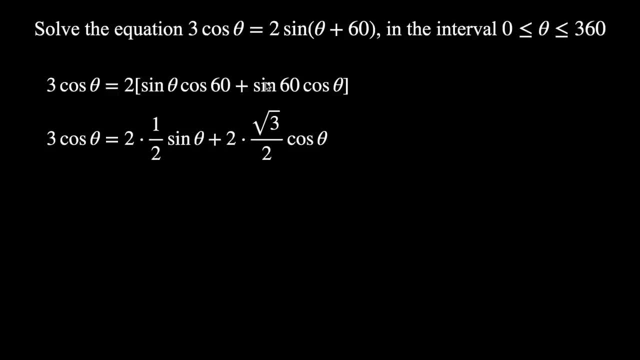 sine Theta plus two multiplied by root three on two, that's sine 60 cosine theta. 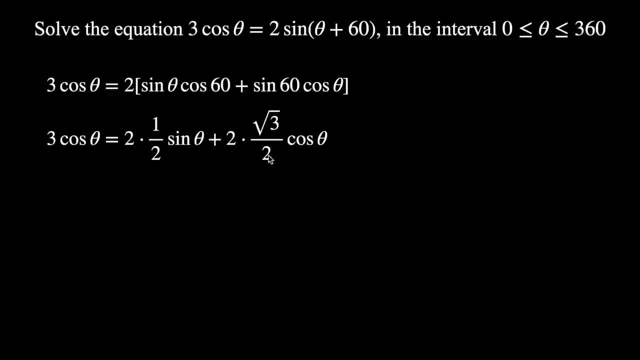 Two times a half is just one, two times root three on two is just root three. So then we get three cosine theta. 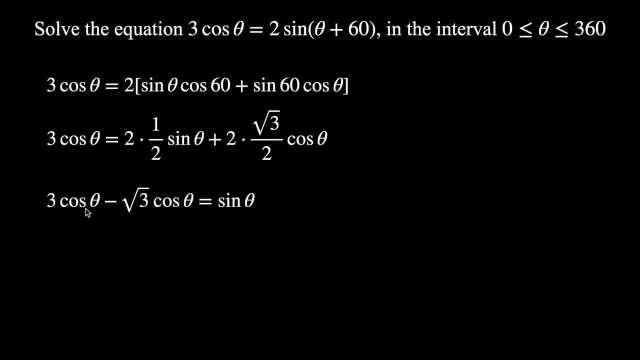 Also I've subtracted this from the left hand side so we get three cosine theta, take root three cosine theta equal to sine theta. 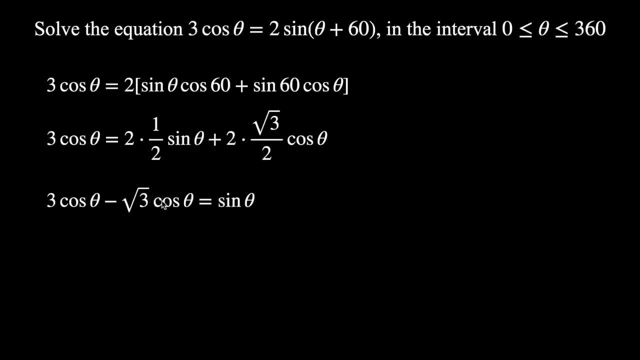 And then we can factorize the cosine theta and divide by cosine theta. 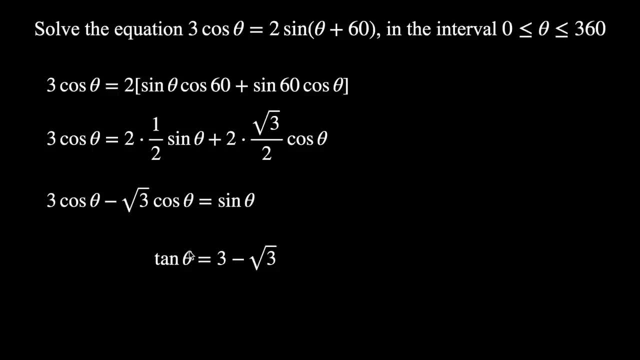 I'm going to take a few steps in one go here. So I get tan theta equal to three take root three. Again, I'm using the fact that cosine theta cannot equal zero in this case. 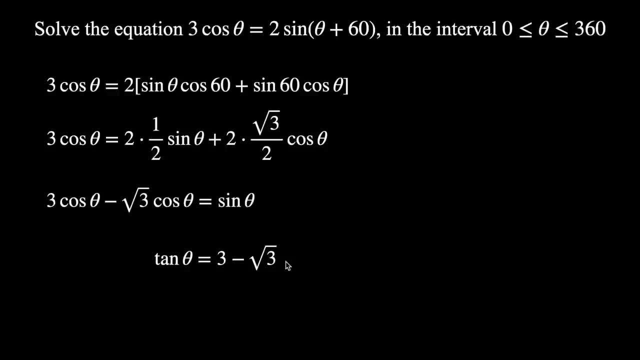 So we get tan theta equal to three take root three. Now we have that trig function on the left, the numbers on the right, so we go to our unit circle now. 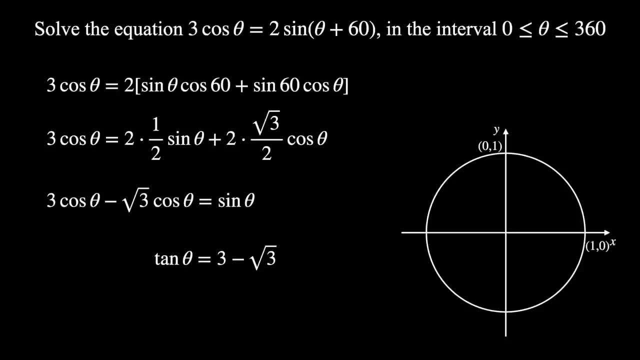 Remember how we're interpreting tan, that's the gradient of the radius. 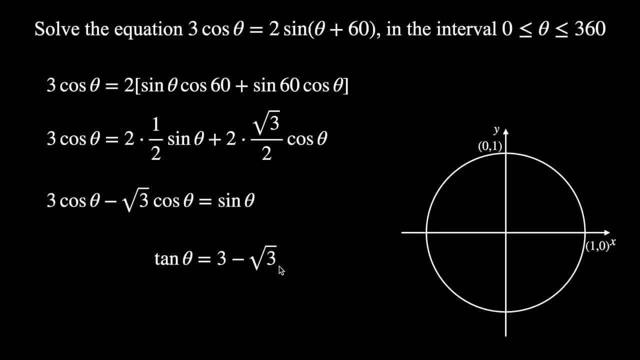 This is a positive number. So gradient of the radius is going to be positive, it's positive in the first and the third quadrant. 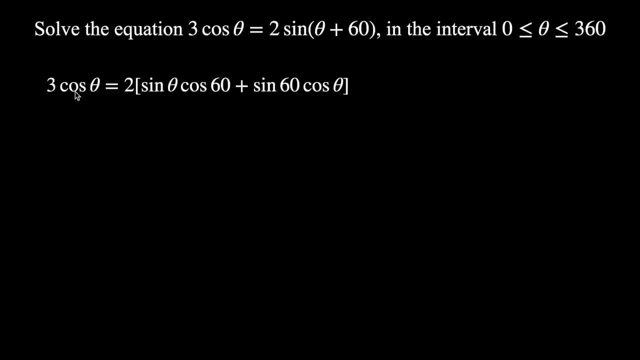 sum formula for sine. we're going to have three cosine theta equal to two sine theta: cosine 60 plus sine 60 cosine theta. these are in your formula booklet, so we need to multiply both by two and also we can use the exact values for cosine 60 and sine 60.. 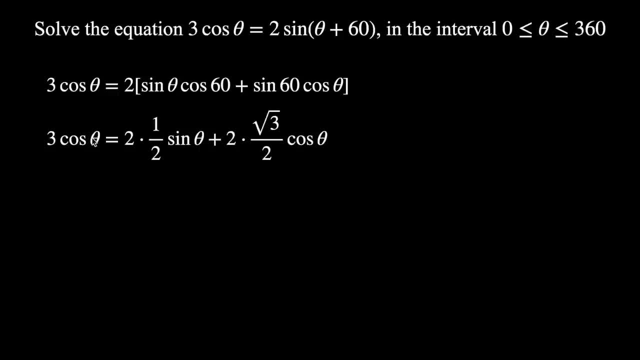 so let's plug those in as well. so we're going to have 3 cosine theta equal to 2 multiplied by a half, that's cosine 60. sine theta plus 2 multiplied by root 3 on 2, that's sine 60.. cosine theta two times a half is just one. two times root 3 on 2 is just root three. so then we 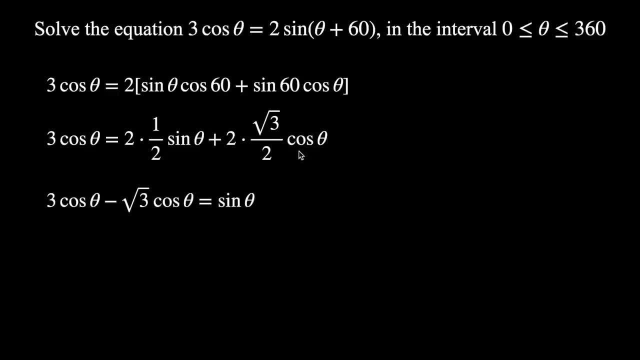 get 3 cosine theta also. I've subtracted this from the left hand side so we get 3 cosine theta take root, 3 cosine theta equal to sine theta. and then we can factorize the cosine theta and divide by cosine theta. I'm going to take a few steps in one go here. so I get tan theta equal to three take root. 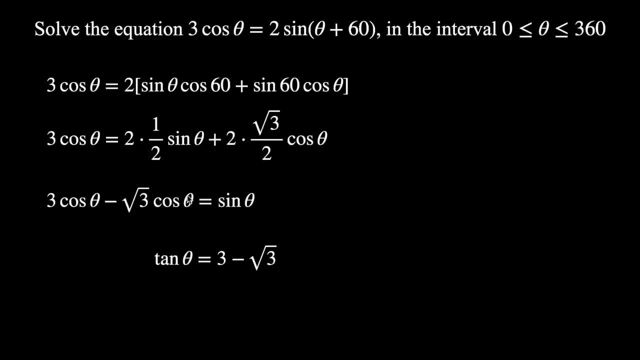 three. I'm using the fact that cosine theta cannot equal 0 in this case. So we get tan theta. could 3 take root 3? now We have that trig function on the left, The numbers on the right, so we go to our unit circle. now remember how we're interpreting tan. That's the, the gradient of the radius. 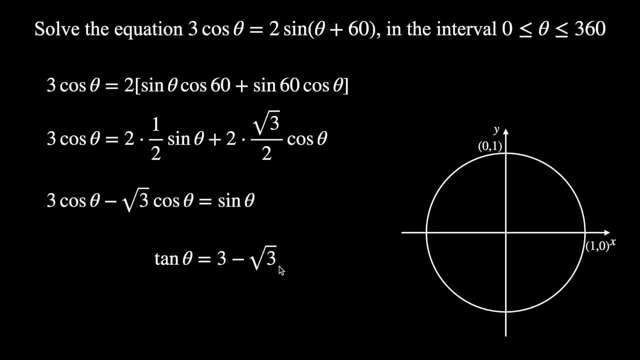 This is a positive number. so a gradient of the radius going to positive is positive in the first and the third quadrants. So we have our radii in the first and third quadrants. Then we're looking for this initial angle to that first radius, to find that issue initial angle. 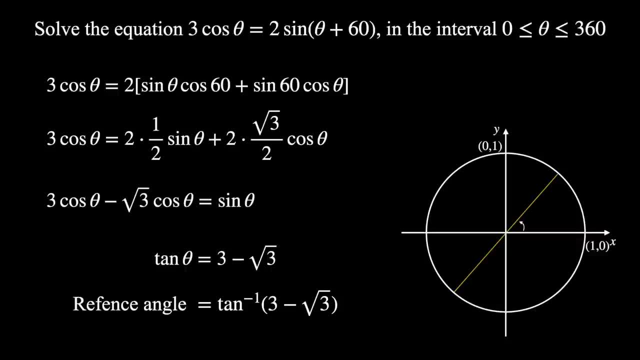 We take the inverse tan of 3, take root 3. That's our reference angle. plug that into a calculator. you get approximately 51.7, so that angle in there is. we can round off to 51.7, for That's one of our solutions. and then in this interval, 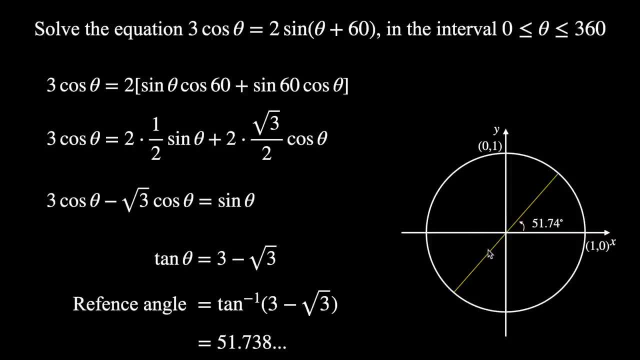 We're going to have a Another solution: the angle of rotation to the second radius, that's going to be 180 plus 51.7, for which is about 231 point seven. So we get solutions for theta over approximately fifty one point seven. four and two hundred thirty one point seven. 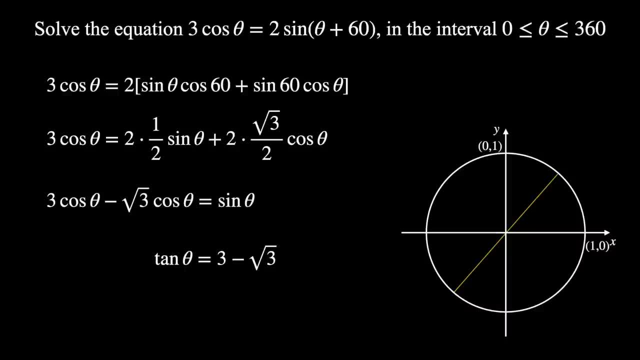 So we have our radii in the first and third quadrants. Then we're looking for this initial angle to that first radius. 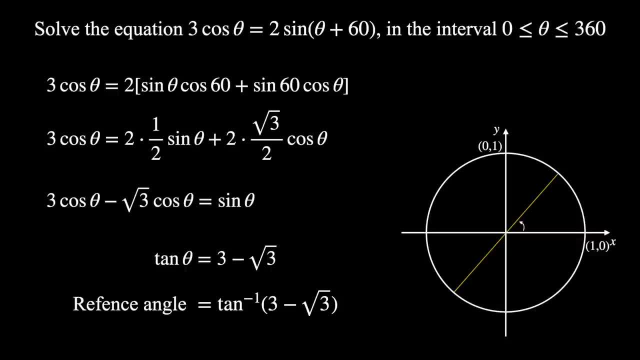 To find that initial angle, we take the inverse tan of three take root three. That's our reference angle. 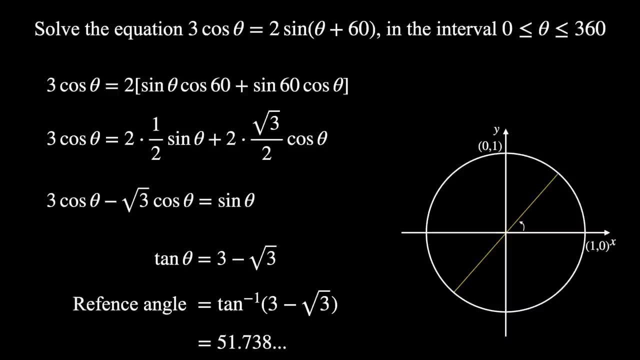 Plug that into a calculator, you get approximately 51.7. So that angle in there is, we can round off to 51.74. 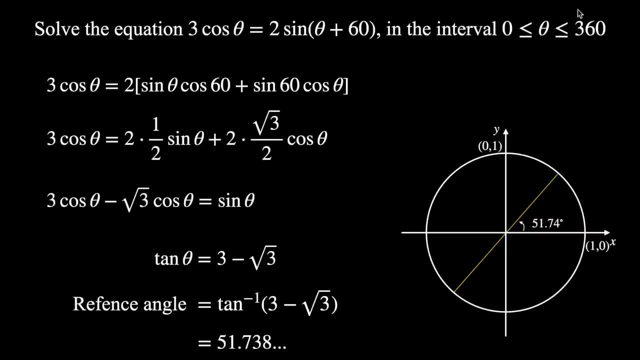 That's one of our solutions. And then in this interval, we're going to have another solution, the angle of rotation to the second radius. 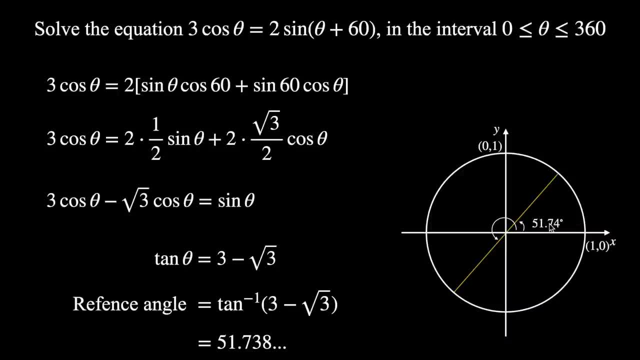 That's going to be 180 plus 51.74, which is about 231.7. 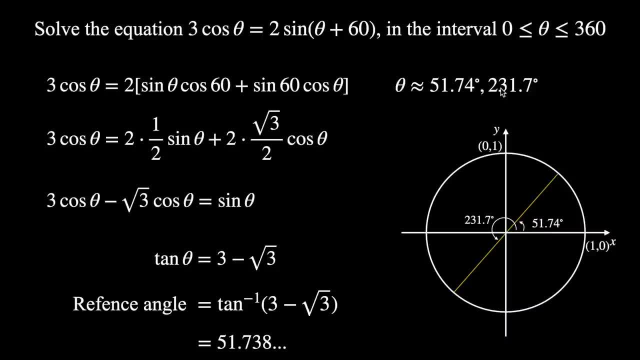 So we get solutions for theta of approximately 51.74 and 231.7. 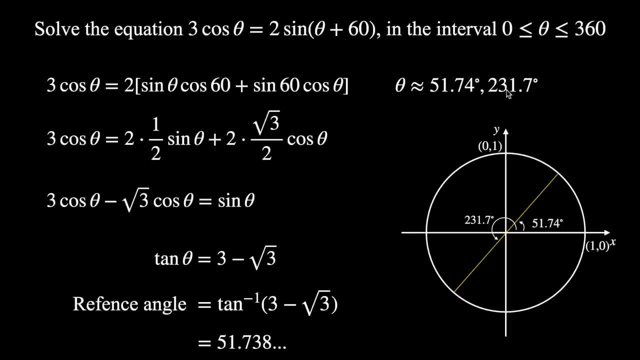 Just to note here that often it's the case that you want to give your answers to the same number of significant figures. 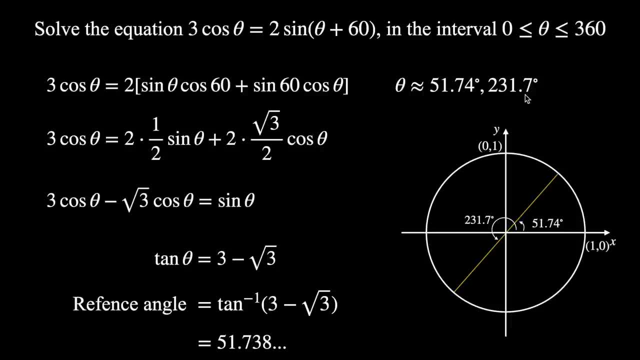 Sometimes it'll be two decimal places or one decimal place, but sometimes it will be, say, three or four significant figures. So anyways, they're your final solutions for that question. 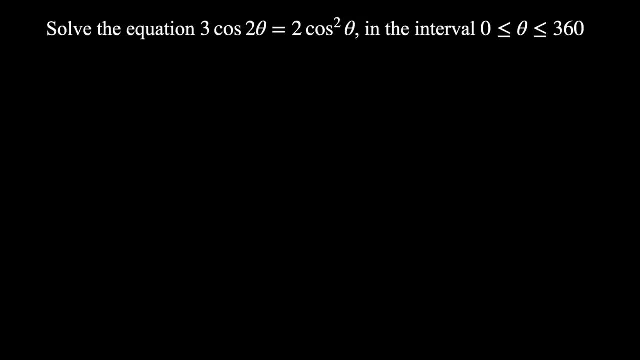 The next one says, solve the equation three cosine two theta equals two cosine squared theta in the interval zero to 360. Here we have a double angle. So we're going to be using our double angle formulas, but which one should we use? So we're going to use the double angle formula. What one should we use? 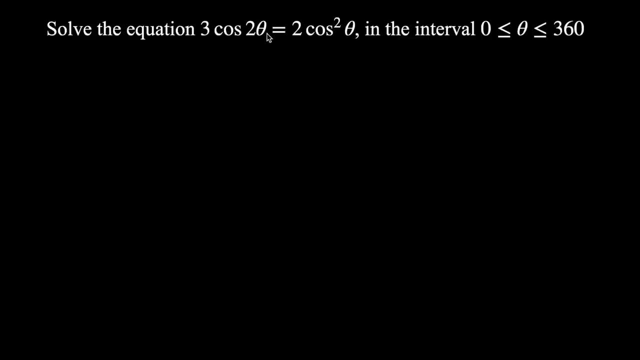 Remember, cosine two theta has three possibilities. There's cosine squared take sine squared, or two cosine squared take one, or one take two sine squared, if you remember those three. So which one should I use? Well, we want all of this in terms of one trig function. So I'm not going to use one take two sine squared, or cosine squared take sine squared. 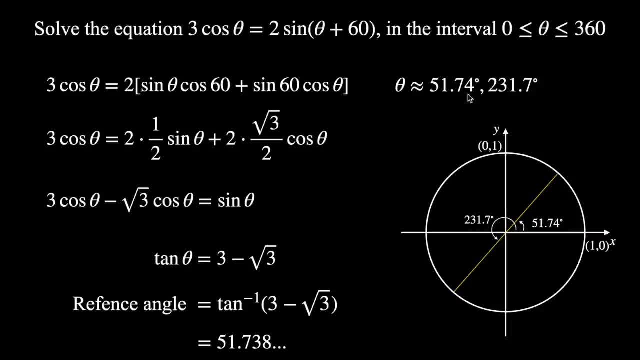 Just to note here that often is the case that you want to give your answers to the same number of significant figures. So here I've used four Significant figures for both answers. sometimes it'll be, you know, two decimal places or one decimal place, But sometimes it will be, say, three or four significant figures. 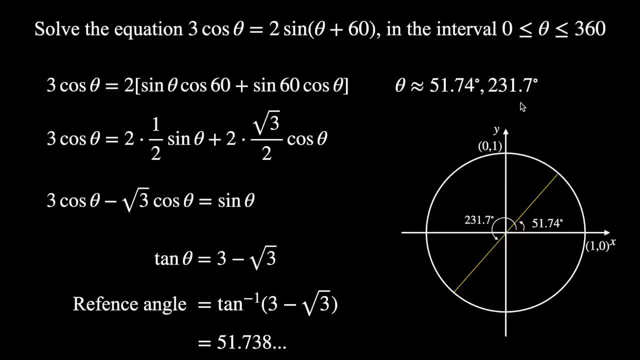 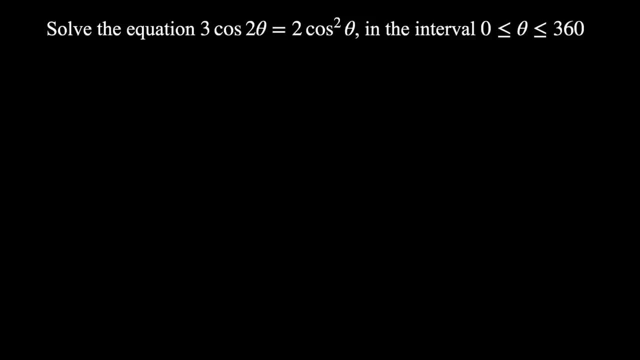 So anyways, they're your final solutions for that question. The next one says: solve the equation: three cosine two theta equals two cosine squared theta in the interval zero to 360. Here we have a double angle, So we're going to be using our double angle formulas. 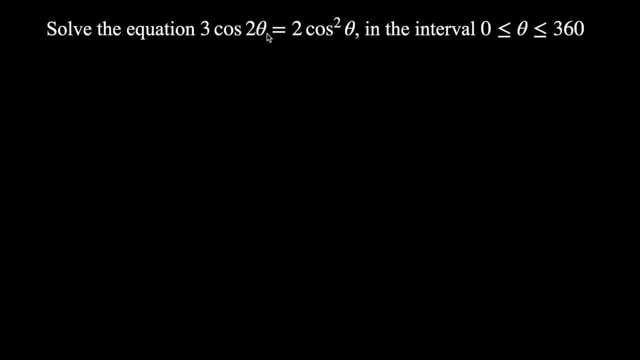 But which one should we use? Remember cosine two. theta has three possibilities. there's cosine squared, take sine squared, or Two cosine squared, take one. or one, take two sine squared, If you remember those three. so which one should I use? well, We want all of this in terms of one trig function, So I'm not going to use one, take two, sine squared, or 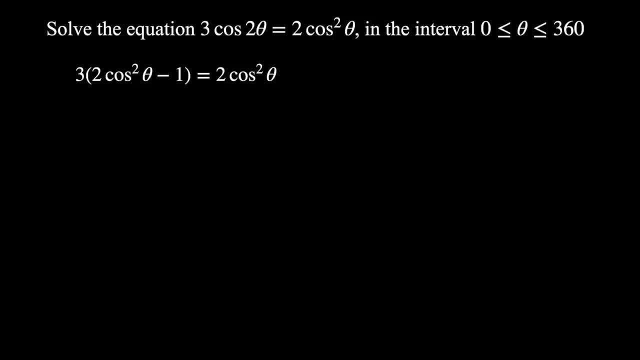 cosine squared, take sine squared, or The one I'm going to use is two cosine squared, take one, So plugging that in. then for cosine two, theta, Then it will all be in terms of cosine squared. Expand out the brackets Three times two. cosine squared is six. cosine squared three times negative one is negative three. 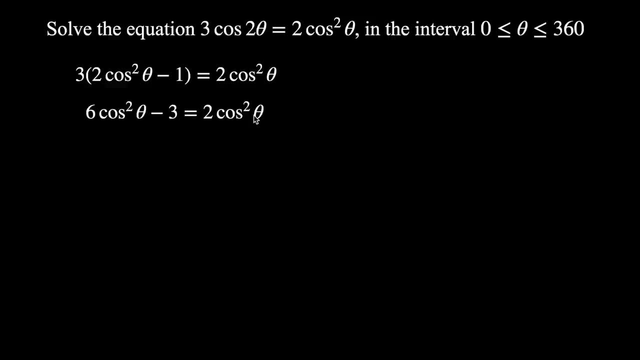 So we get six cosine squared. take three equal to two cosine squared theta. then subtract two cosine squared from the from the left hand side, six take two is. So we get four cosine squared. take three equal to zero, and then rearrange in terms of cosine theta. So add three divided by four, we'll get cosine theta equals plus or minus root three on two. 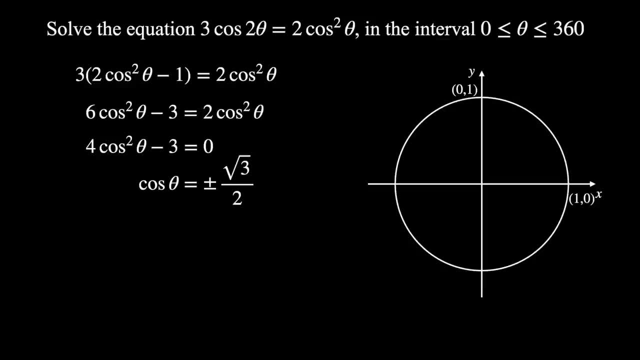 This is the point where we draw up our unit circle During a point. now we have positive and negative solutions for cosine, So we're going to have points in the first and fourth quadrants That's going to have a value of root, positive root. three on two. 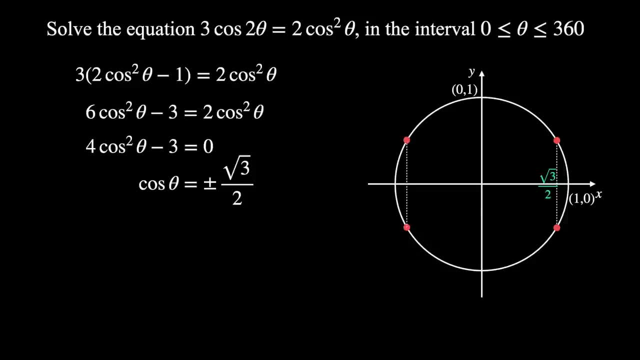 Then we also have points in the second and the third Quadrants. that's going to have an x-coordinate of negative root three on two during your radii, And then all we need is this initial angle here to find that Take the inverse cosine of root three on two. That's one of the exact values. Hopefully you remember. 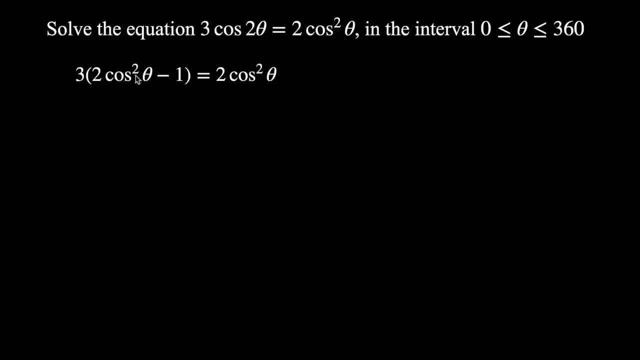 The one I'm going to use is two cosine squared take one. So plugging that in then for cosine two theta, then it will all be in terms of cosine squared. Expand out the brackets. Three times two cosine squared is six cosine squared. Three times negative one is negative three. So we get six cosine squared take three equal to two cosine squared theta. 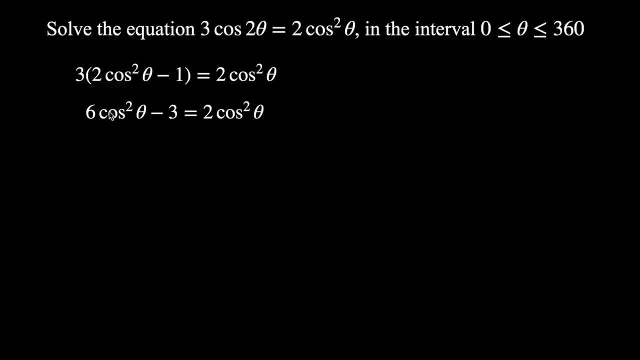 Then subtract two cosine squared from the left-hand side. 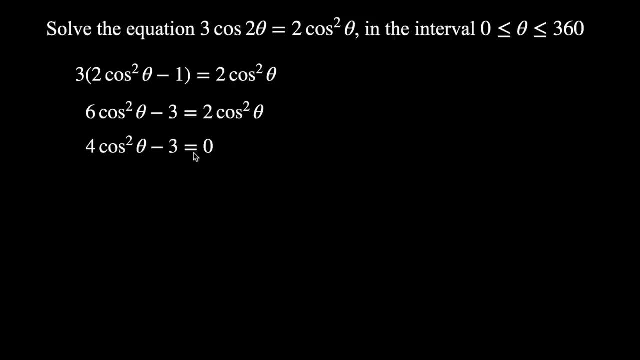 side six take two is four so we get four cosine squared take three equal to zero and then rearrange in terms of cosine theta so add three divide by four we'll get cosine theta equals plus or minus root three on two this is the point where we draw up our unit circle drawing a point now we have positive and negative solutions for cosine so we're going to have points in the first and fourth quadrants that's going to have a value of root positive root three on two then we also have points in the second and the third quadrants that's going to have an x-coordinate of negative root three on two during your radii and then all we need is this initial angle here to find that take the inverse cosine of root three on two that's one of the exact values hopefully you remember so the reference angle here is going to be 30 degrees that initial angle is 30 degrees using that we can find the rest of the square root of cosine theta so that's going to be 30 degrees so the second solution is going to be 180 take 30 150 degrees third point angle rotation is 180 plus 30 210 degrees and the fourth point 360 take 30 that's 330 degrees and then check your interval is that all of the solutions in our interval because the unknown the subject of the function is just theta it's not an expression it's not two theta or whatever we don't have to mess with this interval we can see that's all of the solutions so we get theta 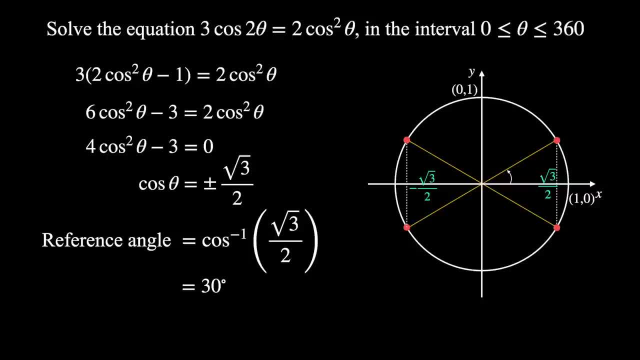 So the reference angle here is going to be 30 degrees. That initial angle is 30 degrees. using that we can find the rest of the solution. So this second solution is going to be 180. take 30: 150 degrees. third point: angle of rotation is 180 plus 30, 210 degrees. and the fourth point: 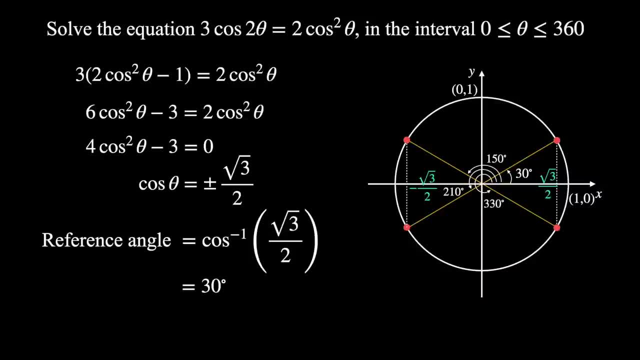 360, take 30, that's 330 degrees, And then check your interval. Is that all of the solutions in our interval? because the unknown, the subject of the function, is just theta. It's not an expression, It's not 2 theta or whatever. We don't have to mess with this interval. 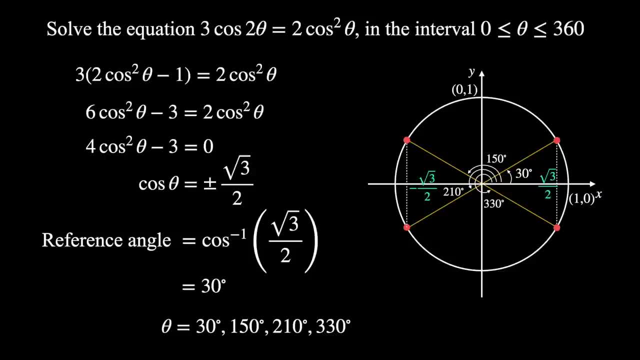 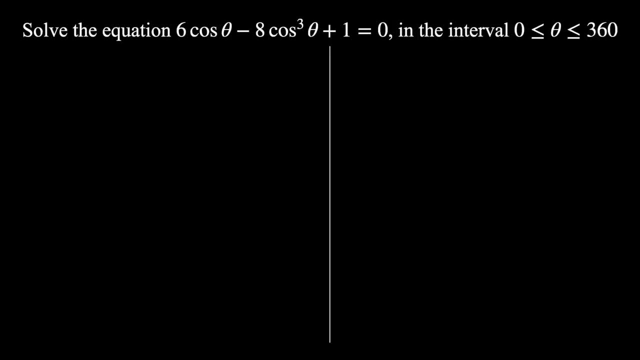 We can say that's all of the solutions. So we get theta equal to 30, 150, 210 and 330. The final question: this is really a step up in difficulty. I wanted to stick a harder problem in here. I hope it's not too different from the rest. 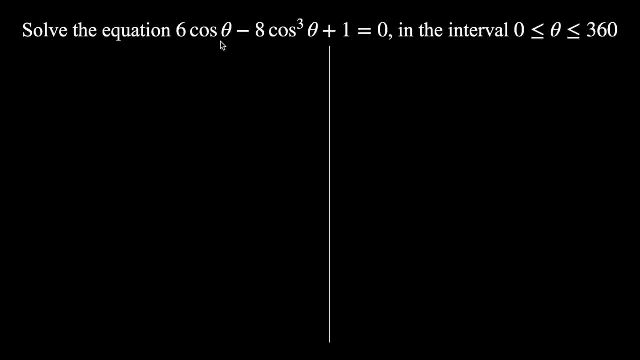 But let's get into this one. So it says: solve the equation 6 cosine theta. take 8 cosine cubed theta plus 1 equals 0 in the interval 0 to 360. Okay, what to do here? Well, it's tricky to say. 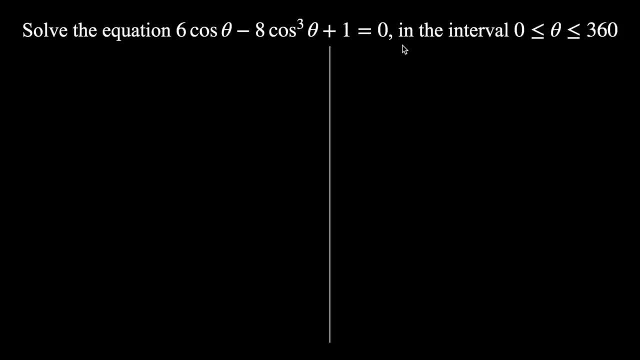 How to begin. I guess my focus will be on what to do about this cosine cubed. Well, One thing I can try first is I can see that can factor as a cosine 0, So that's something I might try initially, so 1.1. 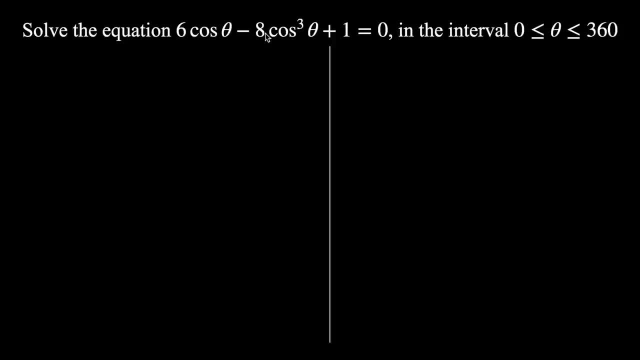 1.1. So the first thing I would try for this equation is Actually factor as a negative 2 And then divide by negative 2. so subtracted that one from the right-hand side, divided by negative 2, we get 4 cosine cubed. take 3 cosine theta equal to 1 half. then I'm going to factorize. 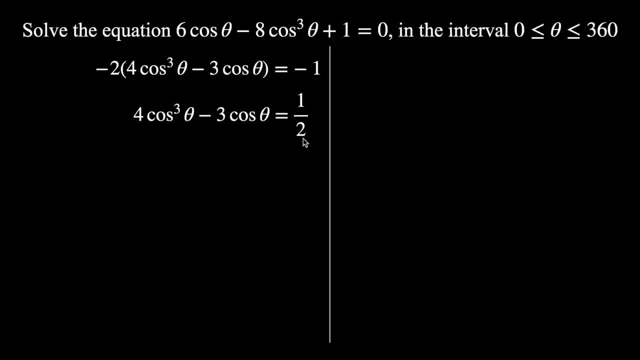 the cosine theta. I could have done it in the previous step as well. let's try that. so we get factorizing cosine theta out of those two terms. we get cosine theta multiplied by 4. cosine squared theta take 3, equal to 1 half. now what can I? 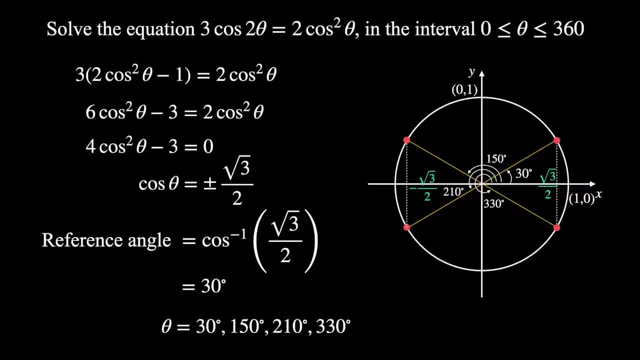 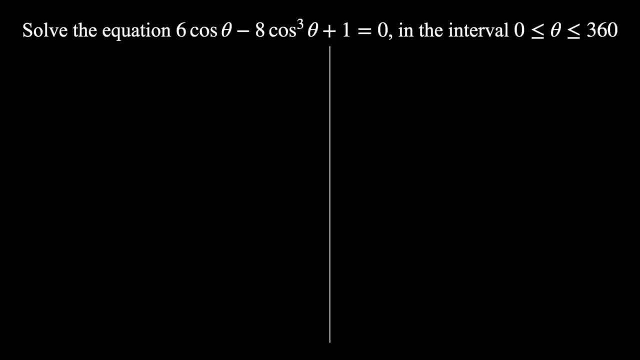 equal to 30 150 210 and 330. the final question this is really a step up in difficulty um i wanted to stick a harder problem in here um i hope it's not too different from the rest uh but let's get into this one so it says solve the equation six cosine theta take eight cosine cube theta plus one equals zero in the interval and we get theta equal to 30 150 degrees and we get theta equal to 30 0 to 360. okay what to do here um well it's tricky to say how to begin um i guess my focus will be on what to do about this cosine cubed well one thing i can try first is i can see that i can factorize a cosine here so that's something i might try initially so the first thing i would try for this equation is actually factorize the negative two um and then divide by negative two so i've subtracted that one from the right hand side divide by negative two we get four cosine cube take three cosine theta equal to a half then i'm going to factorize the cosine theta i could have done it in the previous step as well but let's try that so we get factorizing cosine theta out of those two terms we get cosine theta multiplied by four cosine squared theta take three cosine theta and we're left with cosine theta equal to two and a half and i've basicallyorialized something famous when it came to the integrate organic managing of phi in another way so if we look 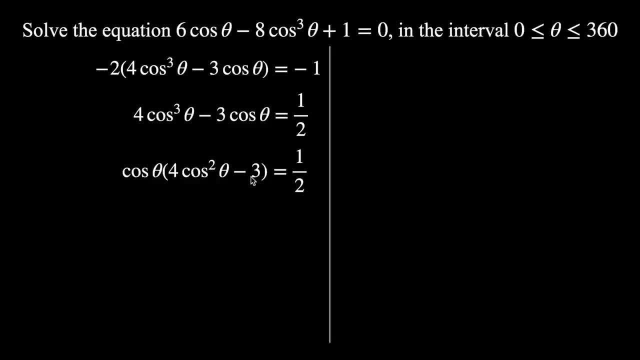 at a volcano for for the well this expression here is four cosine squared theta take three kind of reminds me of one 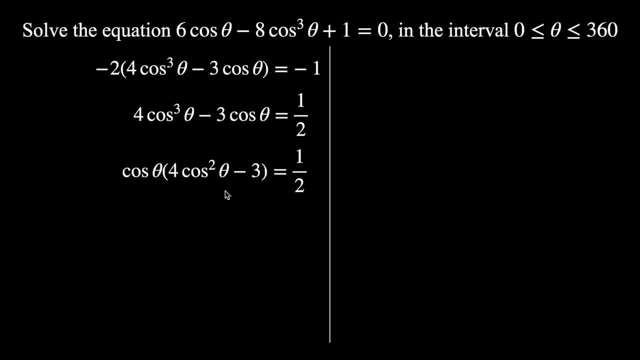 try. well, this expression here- 4- cosine squared theta, take 3- kind of reminds me of one of the identities for cosine 2 theta, one of the double angle identities. so the next thing: I might try to see if I can somehow rearrange this so I get 2. 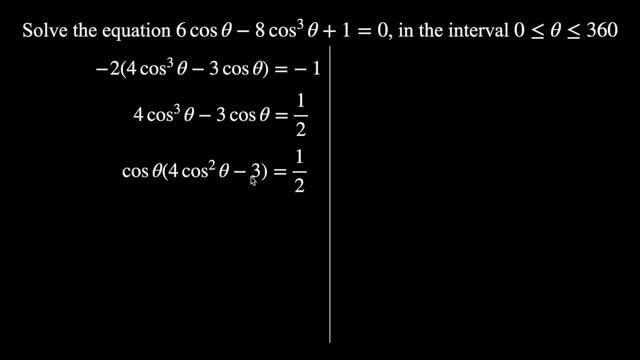 cosine squared theta. take 1. is it possible to get that from this expression? well, well, yeah, right. if I split this 4 cosine squared into 2 plus 2 cosine squared theta, then maybe I can get this double angle identity for cosine theta. okay, so. 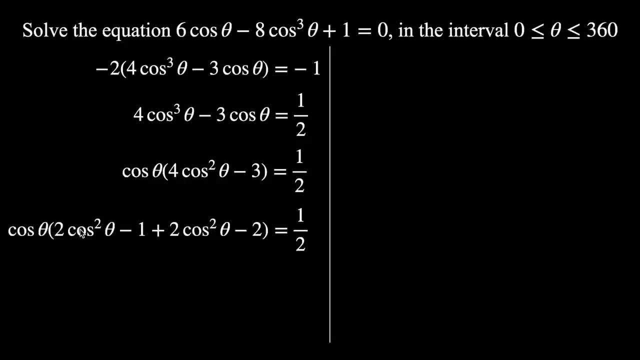 let's try that. we've got cosine theta equal to 2 cosine squared theta take 1 plus 2 cosine squared theta take 2. so here I've split the 4 cosine squared into 2 cosine squared and 2 cosine squared and I've 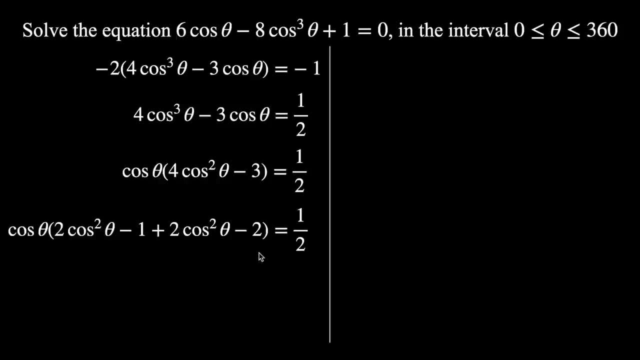 also split the negative 3 into negative 1 and negative 2.. So now I can substitute in cosine 2 theta for 2 cosine squared theta- take 1. but what am I going to do about this? 2 cosine squared theta- take 2? hmm, okay, so I'm going to substitute in 1. 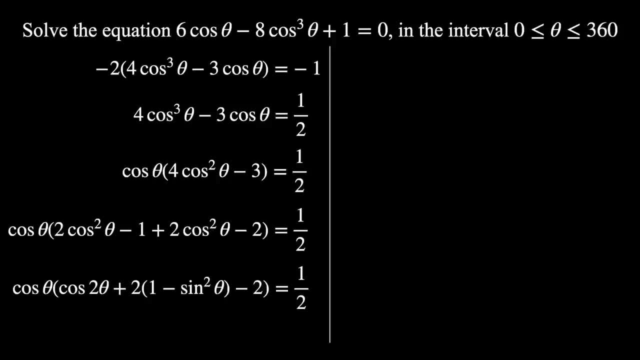 take sine squared. 4: cosine squared. so my next line is cosine theta equal to cosine 2, theta that substituted for all of this, and then cosine squared. of substituting 1. take sine squared for cosine squared. so two times that take two equals a half. expand these brackets. this would be two take two. so we're going to end up with: 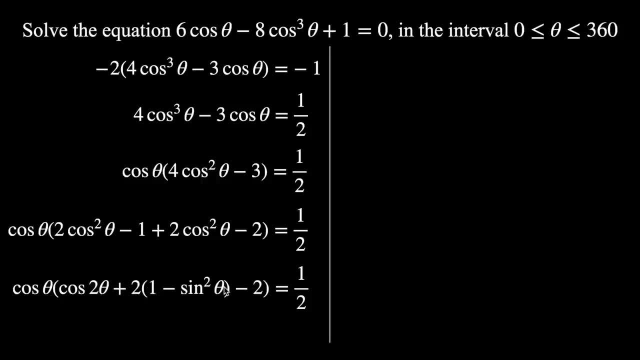 here is negative two sine squared theta. so my next line is: cosine theta multiplied by cosine two theta. take two sine squared theta equal to a half. my next thought is: this is kind of looking like one of my sum and difference formulas. ok, so let's expand these brackets and see where we can go from. 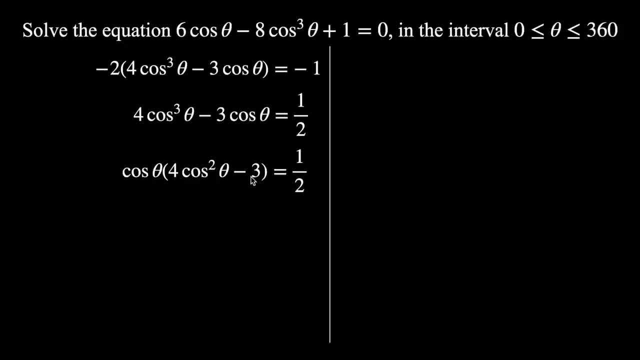 of the identities for cosine two theta one of the double angle identities so the next possible to get that from this expression? Well, yeah, right? If I split this 4 cosine squared into 2 plus 2 cosine squared theta, then maybe I can get this double angle identity for cosine theta. Okay, so let's try that. We've got cosine theta equal to 2 cosine squared theta take 1 plus 2 cosine squared theta take 2. So here I've split the 4 cosine squared into 2 cosine squared and 2 cosine squared. And I've also split the negative 3 into negative 1 and negative 2. So now I can substitute in cosine 2 theta for 2 cosine squared theta take 1. But what am I going to do about this 2 cosine squared theta take 2? Okay, so I'm going to substitute in 1 take sine squared for cosine squared. So my next line is cosine theta equal to cosine 2 theta. That's substituted for all of this. 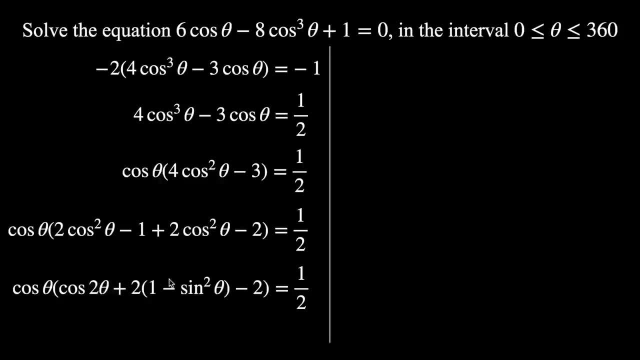 And then cosine squared, I've substituted 1 take sine squared for cosine squared. So 2 times that take 2 equals a half. Expand these brackets. This will be 2 take 2. So all we're going to end up with 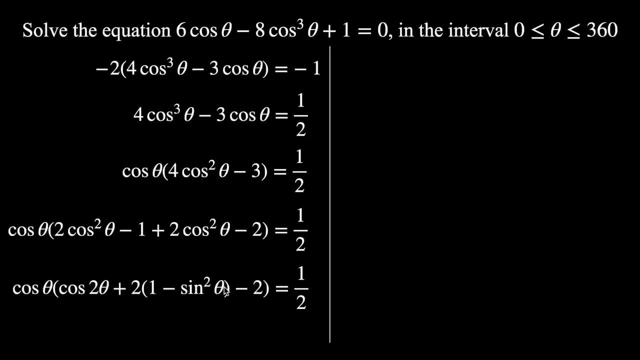 here is negative 2 sine squared theta. So my next line is cosine theta multiplied by cosine 2 theta take 2 sine squared theta equal to 1. So I've substituted 1 take sine squared for cosine squared 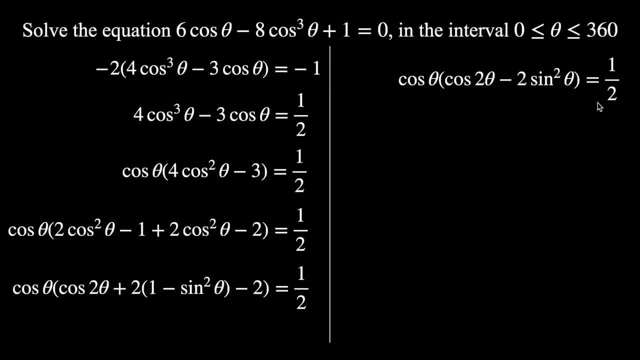 and 2 cosine squared theta. So I've substituted 1 take sine squared for cosine 2 theta. So my next thought is this is kind of looking like one of my sum and difference formulas. Okay, so let's expand these brackets and see where we can go from there. So multiplying by cosine theta, we get cosine theta cosine 2 theta. And here I'm going to write sine squared as sine theta sine theta. So cosine theta cosine 2 theta take 2 sine theta cosine theta. That's, you know, after expanding the brackets. 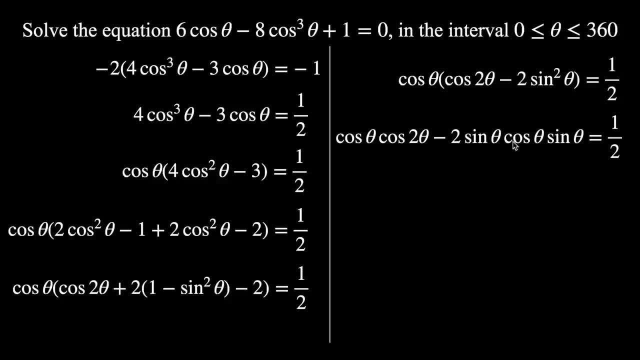 2 sine theta cosine theta sine theta. What's this in here? 2 sine theta cosine theta. That's the 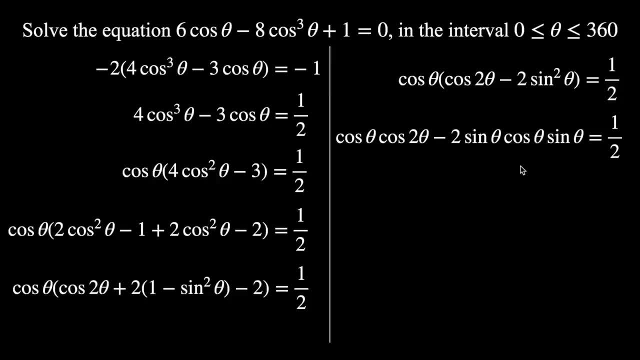 identity for sine 2 theta. So let's sub in sine 2 theta for this. Cosine theta cosine 2 theta take 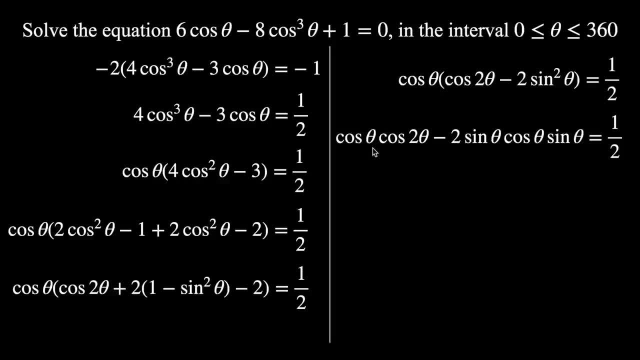 there. so multiplying by cosine theta, we get cosine theta, cosine two theta, and here I'm going to write sine squared as sine theta, sine theta. so cosine theta, cosine two theta. take two sine theta, cosine theta, that's, you know, after expanding the brackets, two sine theta, cosine theta, sine theta. what's this in here? 2 sine theta, cosine theta. 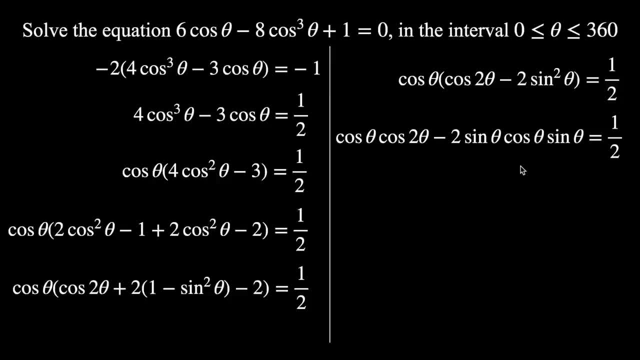 that's the identity for sine 2 theta. so let's sub in sine 2 theta for this cosine theta, cosine 2 theta. take sine 2 theta, sine theta equal to a half. now what do we have here? does this remind you of anything? hopefully thinking of? 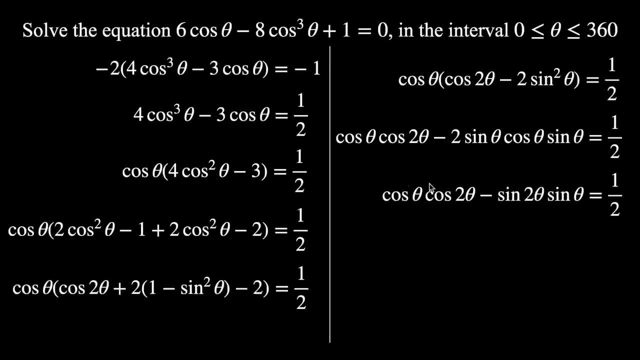 cosine of a plus B. remember, cosine of a plus B is cosine of a, cosine of B. take sine of a, sine of B, so we can write this expression as cosine of 2 theta plus theta equal to a half, in other words, cosine of 3 theta equal to a half. okay, 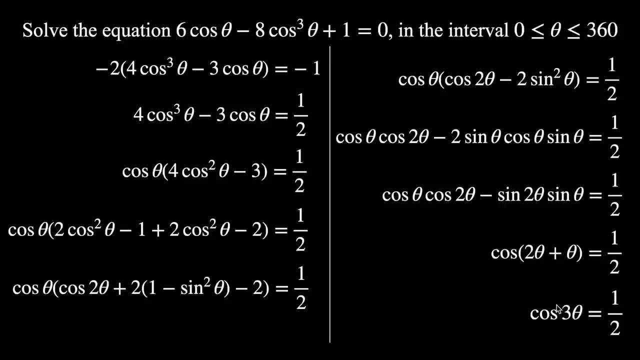 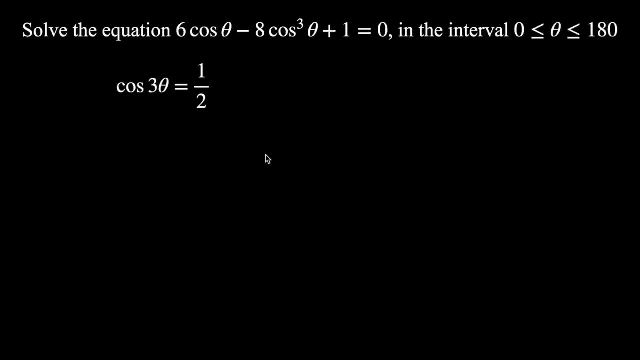 so after all of that, we have that trig function on the left, the constant on the right, and we can finally solve this for theta you. yeah, that's a bit of a step up from the previous problems. hope not too difficult, okay. so, cosine of theta equal to a half. let's proceed with our unit. 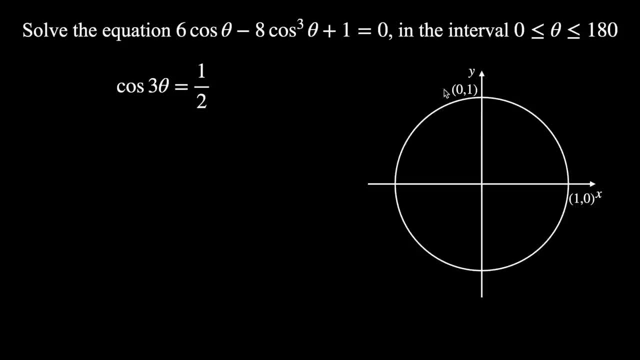 circle. picture that point because it's positive. it would be in the first and the fourth quadrants and the X coordinate is a half. okay, so we have that X coordinate drawing your radii and we want to figure out that angle. again, remember your exact values. when cosine of theta equals to a half, the angle is 60 degrees. so this angle in 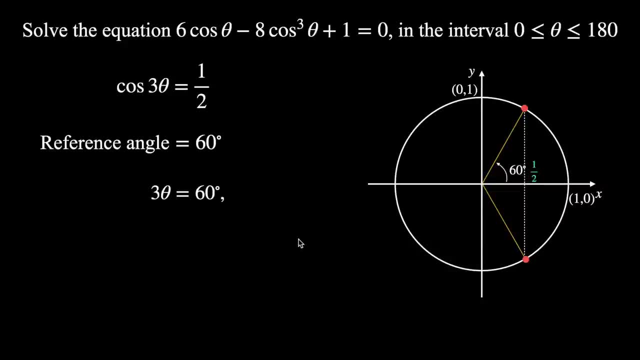 here is 60, so that's one of our solutions for 3 theta: 360 degrees. now is a good time to think about the interval. what's, what will be the interval for 3 theta? let's multiply the bounds by 3: the interval for 3 theta will be from 0 to. 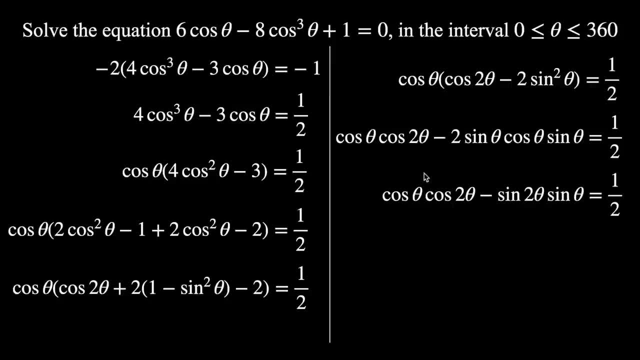 sine 2 theta sine theta equal to a half. Now what do we have here? Does this remind you of anything? 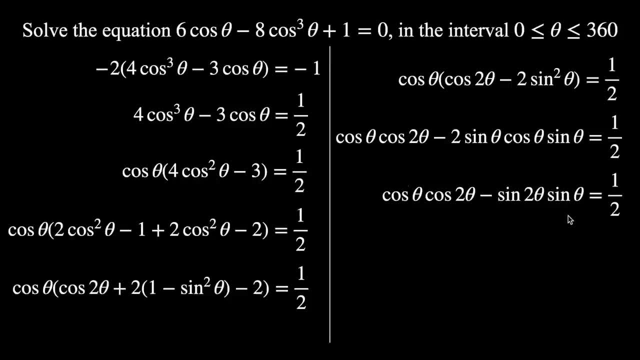 Hopefully thinking of cosine of a plus b. Remember cosine of a plus b is cosine. Cosine of a cosine of b take sine of a sine of b. So we can write this expression as cosine of 2 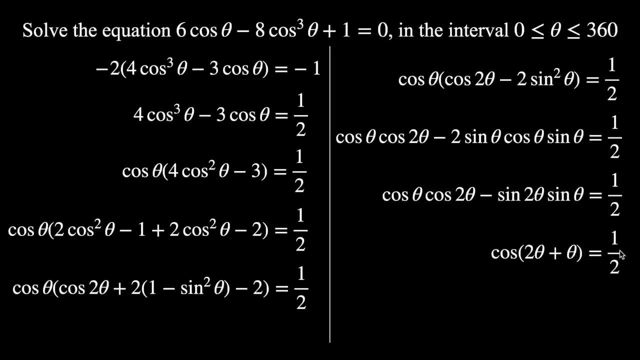 theta plus theta equal to a half. In other words, cosine of 3 theta equal to a half. Okay, so after all of that, we have that trig function on the left, the constant on the right, and we can finally 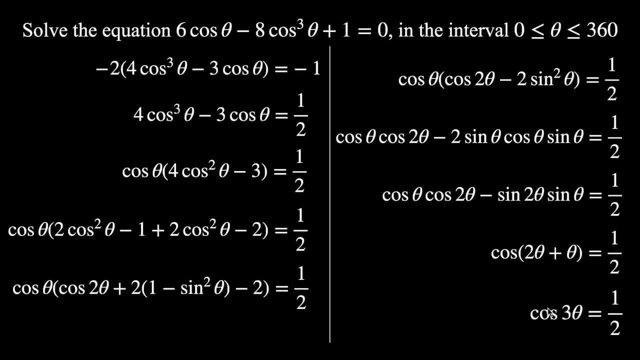 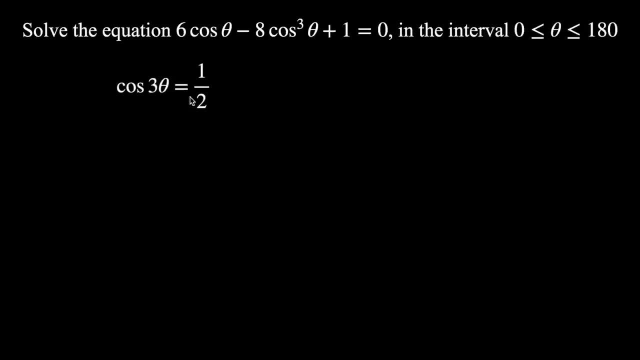 solve this for theta. Yeah, that's a bit of a step up from the previous problems. Hope not too difficult. Okay, so cosine of theta equal to a half. Let's proceed with our unit circle. 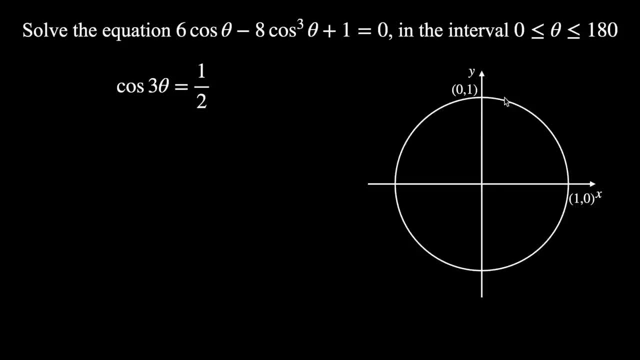 Picture that point because it's positive. It would be in the first and the fourth quadrants, and the x coordinate is a half. Okay, so we have that x coordinate. Draw in your radii, and we want to figure out that angle. 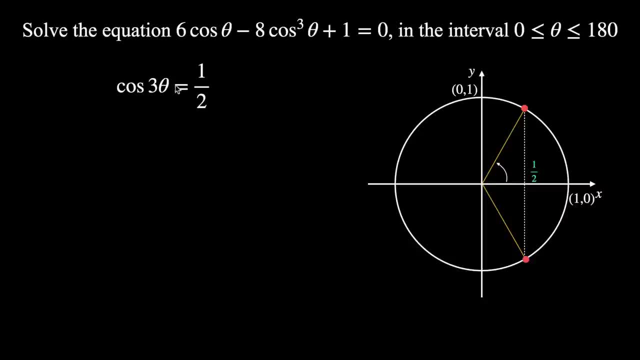 Again, remember your exact values when cosine of theta equals to a half, the angle is 60 degrees. So that's the 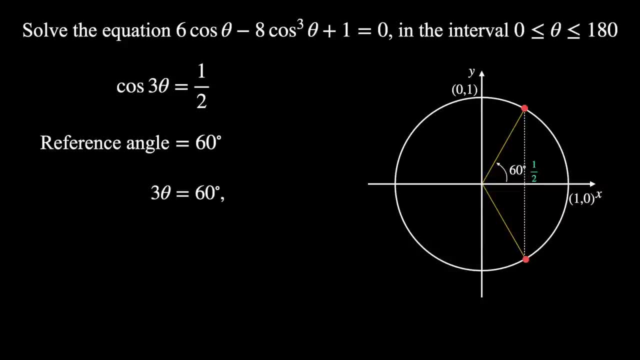 So this angle in here is 60. So that's one of our solutions for three theta. Three theta equals 60 degrees. 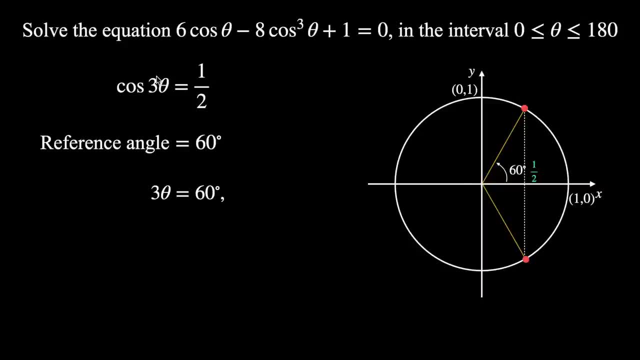 Now is a good time to think about the interval. What will be the interval for three theta? Well, let's multiply the bounds by three. 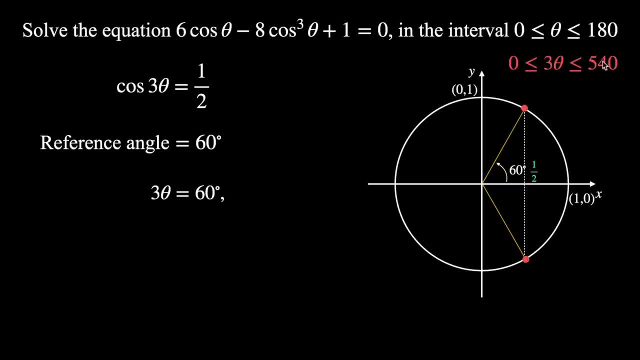 The interval for three theta will be from zero to 540. That's 180 times three. So we need to include all of the solutions from zero to 540 for three theta. 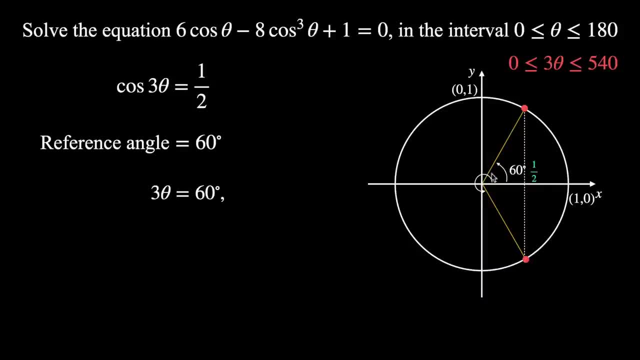 So that's going to be this one. That's 360 take 60, that's 300 degrees. And if we go around to this first point again, that's going to be 360 plus 60, that's 420. 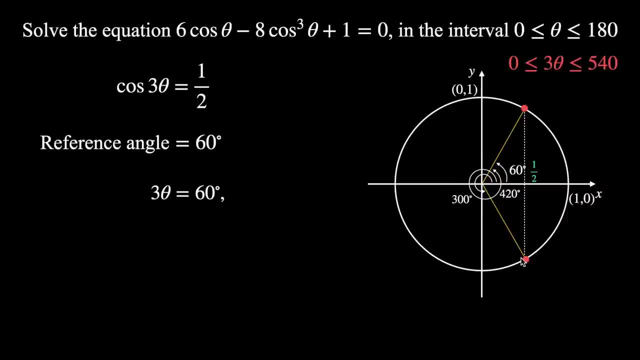 And if I go around a second time to the second point, that's going to be greater than 540.